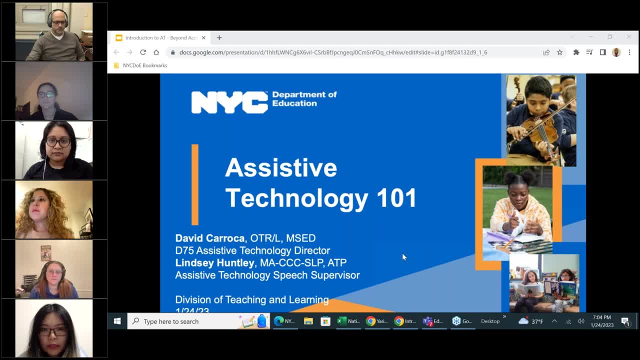 questions in for the central office And then for the central office and team to communicate concerns or questions that you have. The chat section is open for everyone to see, but we would like for you to refrain from using the chat section and direct all questions that you have for our central office team. 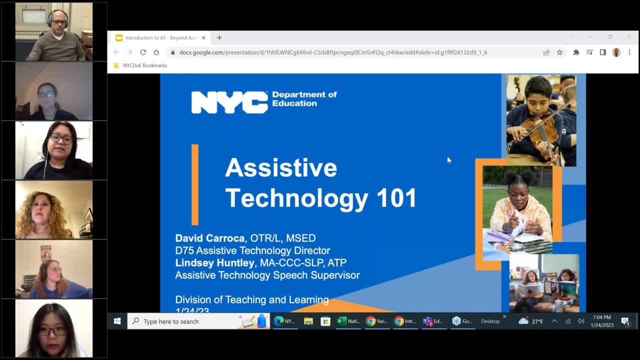 in the questions section, You should also see the option to raise your hand. We will not be using the raise hand option for this particular webinar session this evening And you should also see an option for you to raise your hand Or you to share your screen. 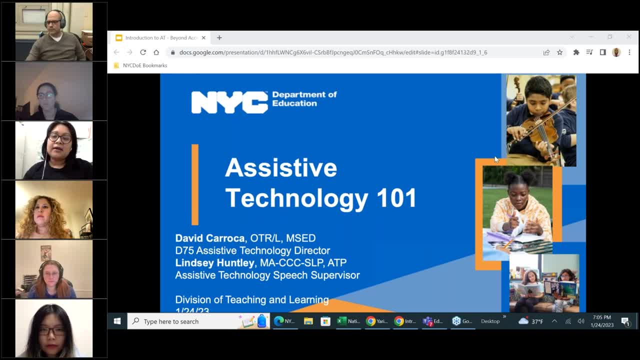 We have disabled that option as well. this evening You will only have the option to direct questions in the chat- sorry, in the questions section of your dashboard. So again, there is a dashboard on your screen and there you'll see a chat and questions. 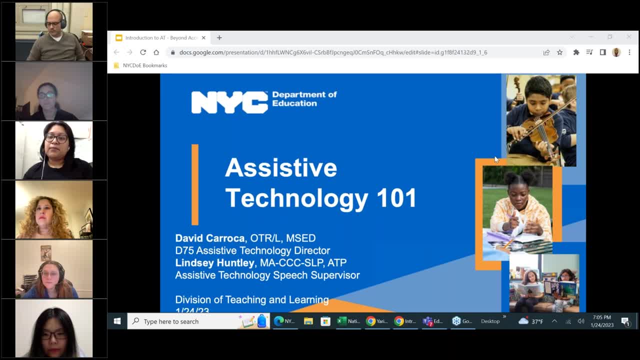 section. Please refrain from using the questions section of the dashboard. Place all questions that you might have or concerns in the questions section of your dashboard And our central office team will gladly respond to it throughout our session. Thank you, Thank you. Thank you very much. 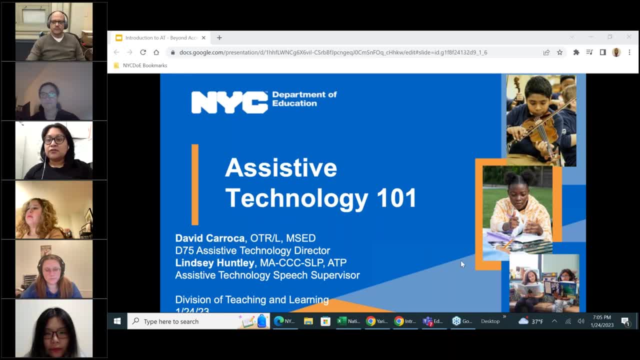 I appreciate your attention this evening. Okay, We're at 7.05.. And I see that we have a little over a hundred people with us this evening, So excited for that. Don't want to keep people waiting, So like to get underway. 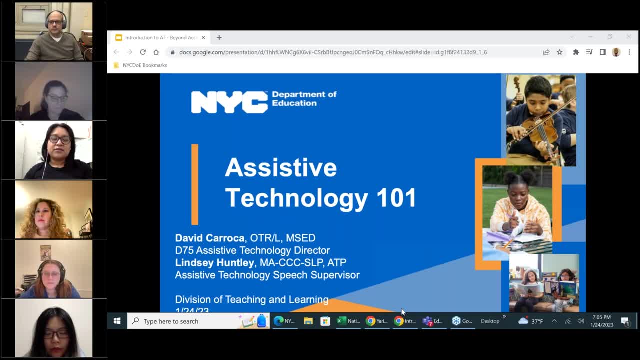 I like to introduce myself. My name is Andre Mitchell. I'm the director of Family Empowerment and Communications for the Division of Specialized Instruction and Student Support. I'm joined by several of my phenomenal colleagues this evening which are going to be facilitating 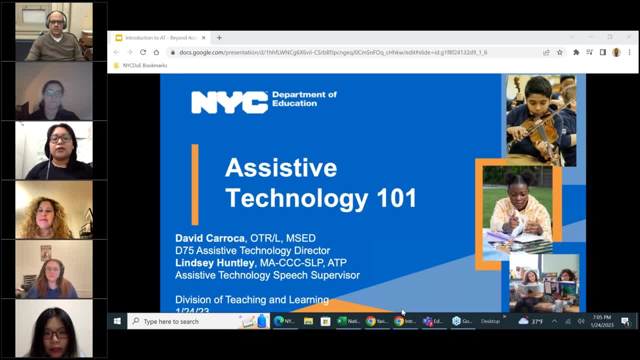 Assistive Technology 101 for you. But before I do that I'd like to have, Okay, one of our other directors give a warm introduction of the team. suzanne, the floor is yours. oh, thank you so much, andre, and uh so excited to have so many uh up- about 110 uh folks- with us this evening. 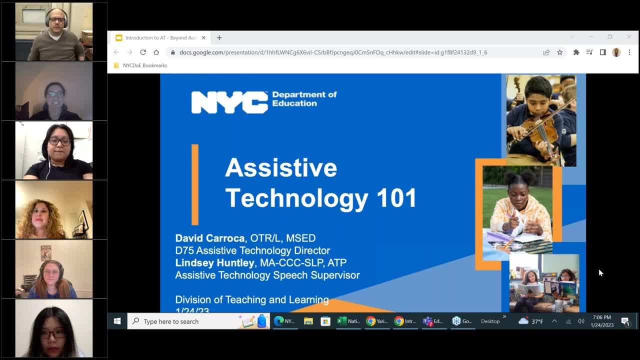 uh know that it's kind of cold and gray out tonight, so hope everyone is inside somewhere warm and we have a really informative uh presentation tonight to talk to you all about assistive technology. and assistive technology, as you're going to hear much more about, is any device or 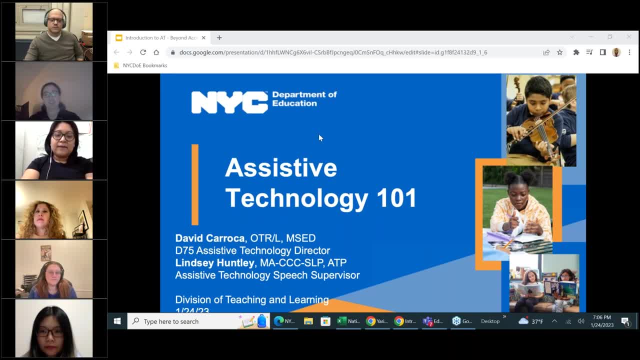 software or program that helps a student with a disability access their curriculum, socialize with their peers and just be active members of their classroom and school communities. tonight, leading the presentation is going to be david karaka. david is the director of district 75's technology solutions team and a specialist and expert in the continuum of assistive technology services. 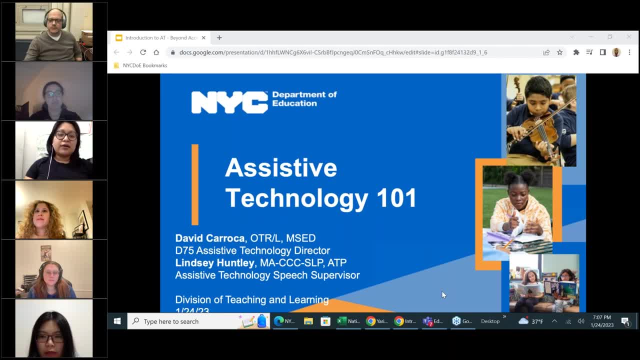 we are also joined this evening by assistive technology supervisor lindsay huntley. lindsay also has expertise across the continuum of assistive technology and she specializes in communication devices and helping students to communicate using a variety of different ways, in whatever way and method works best for that student. so we have a lot of information to get. 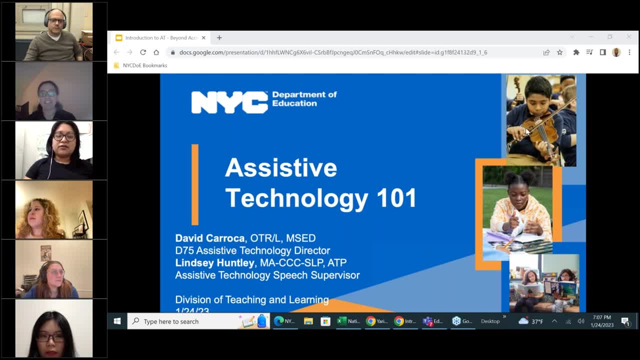 through tonight and hope that you can drop your questions, as andre referenced in the question section um, and i'm going to turn this over to david and lindsay right now. thank you so much. thank you, suzanne. thank you, suzanne. thank you, andre, for joining us today and we look forward to working with you in the future as well. 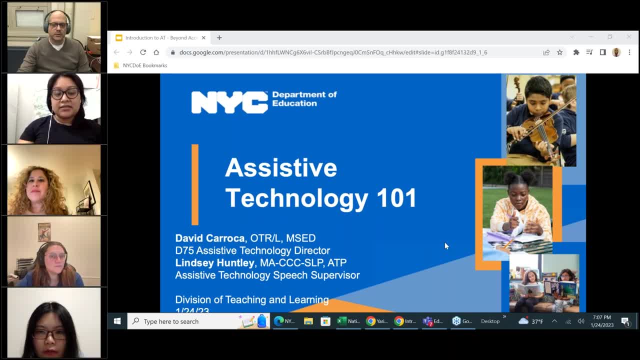 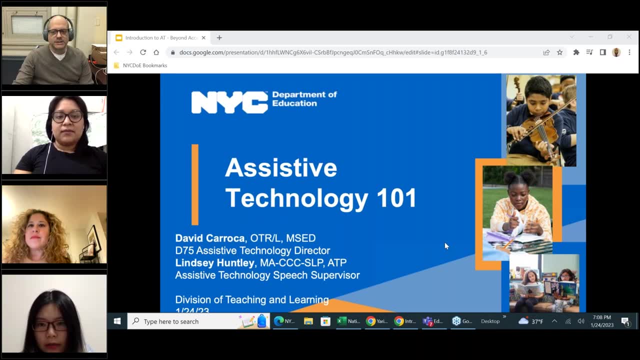 good evening. as suzanne said, my name is david karoka. i'm the director of assistive technology for district 75, um. we're so happy to be here tonight with you to discuss assistive technology as part of this beyond access series. my partner again for tonight's presentation is lindsay huntley. 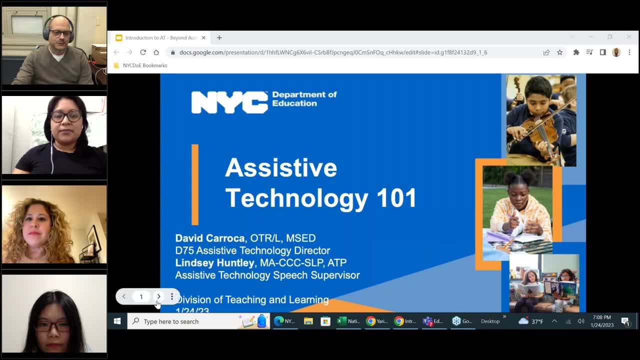 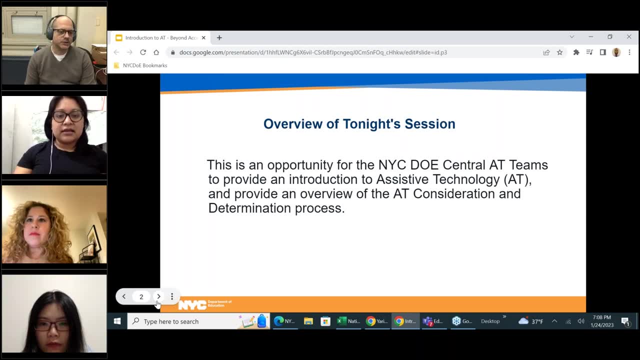 hello lindsay, good evening um andre. next slide to assistive technology, where we will be reviewing the assistive technology consideration and the determination process. we will also be providing an overview of a case study of a student who is benefiting from assistive technology to access reading and writing opportunities. we will be reviewing our 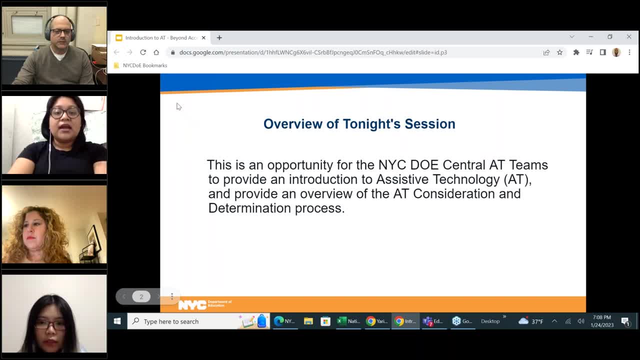 assistive technology toolkit and we will leave some time at the end for a question-and-answer session. next slide: yeah, what we do. some folks who just came in very most recently and wanting to hear the interpretation line will also drop that in the question for folks to. 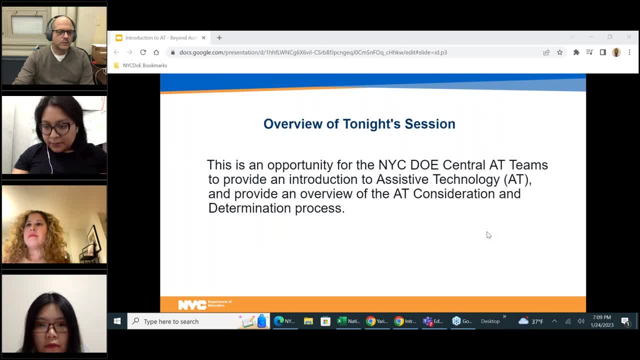 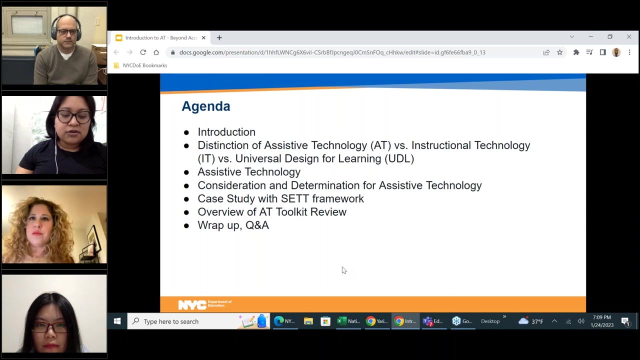 see, but can our Spanish interpreter please repeat the Spanish conference information one more time? yes, to join this up. our initial interpretation in espanol for former market: al-720-527-5818 ingress: el acceso de codico uno seis cero, cinco, cuatro, siete, cuatro. simbolo numeral nuevamente numero de teléfono es: 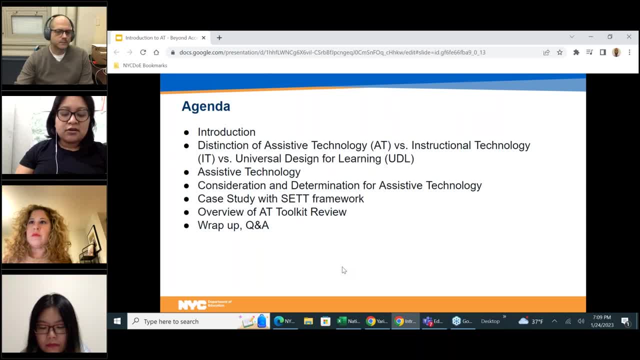 siete, dos cero cinco, dos siete, cinco ocho. uno ocho ingresa el acceso de codico uno ocho ingrese: el acceso de codico uno. seis cero cinco, cuatro, siete cuatro. símbolo numeral. gracias, thank you. thank you, David. thank you, so we will further the agenda for tonight's session. 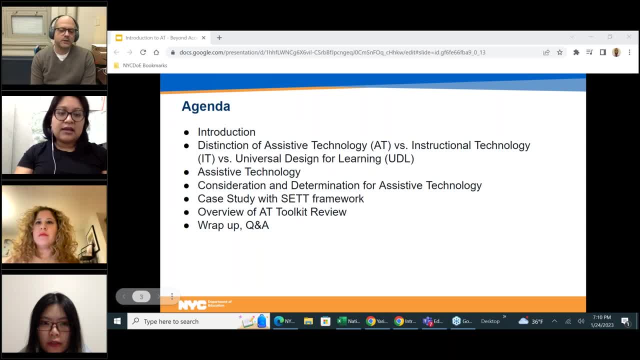 we're going to be introducing the two assistive technology teams in the shared mission of both teams. we will be reviewing the distinction between assistive technology, also known as a two assistive technology, and assistive technology, T, instructional technology or IT, and universal design for learning- UDL. we 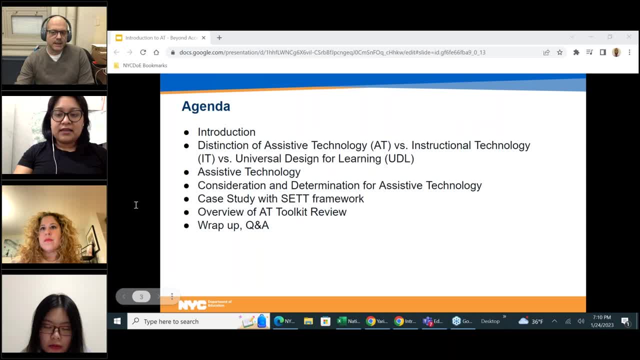 will be defining assistive technology according to IDA or the individual's Disability Education Act, with the, which is the federal law that supports students with disabilities, where we will review the a? T consideration and the determination process and discuss how the relationship of these processes supports IEPs. We will also be presenting a case study using 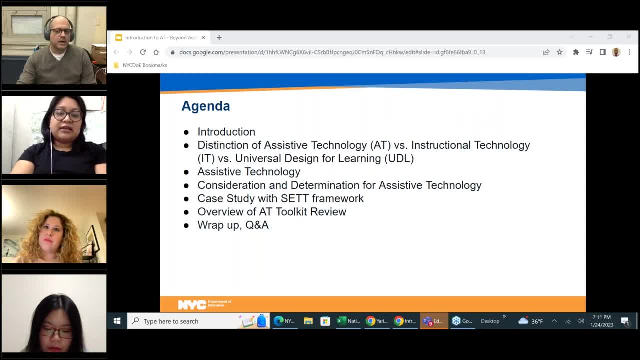 what's called the SET Framework, which can help IEP teams identify the needs and AT tools required to support students, And then we will also be reviewing our AT toolkits and present some of the tools that are most commonly recommended for communication, reading and writing, math and. 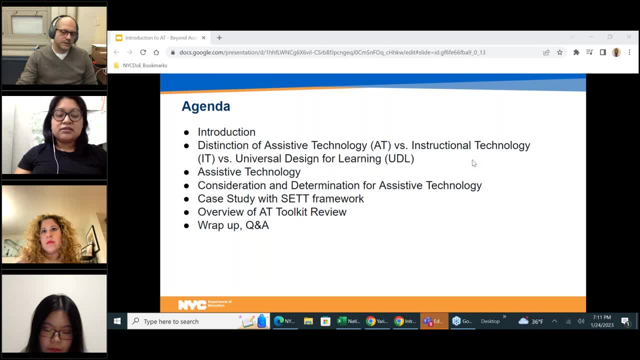 executive functioning, better known in our world as organizational skills, Andre, is there any way? there's some feedback. Is there perhaps like a mic that's on or no? Let me take a look. One of our attendees has their mic on Hold on one second. Is that better? 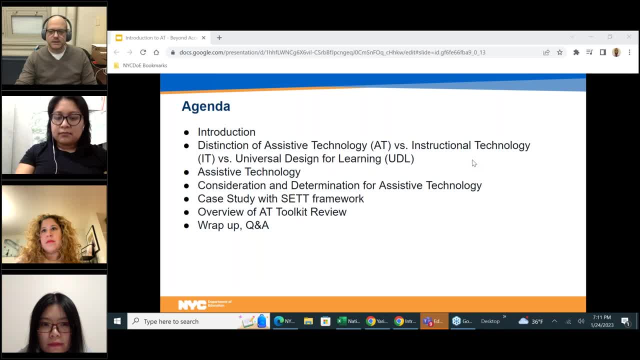 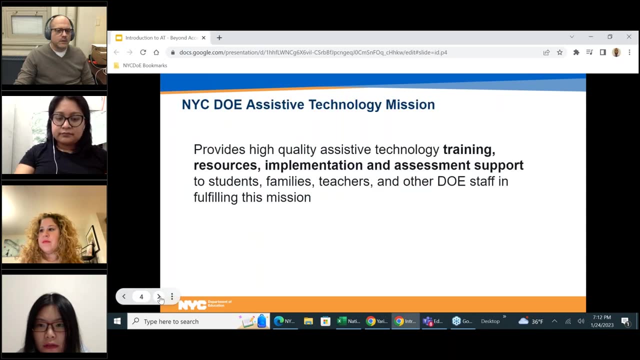 Let's see. I think that may be better. Yes, Okay, And again, we will have a Q&A at the end, Next slide. Thank you, Andre. So both teams, the District 75 Assistive Technology Team as well as the Center for Assistive Technology, share one mission. 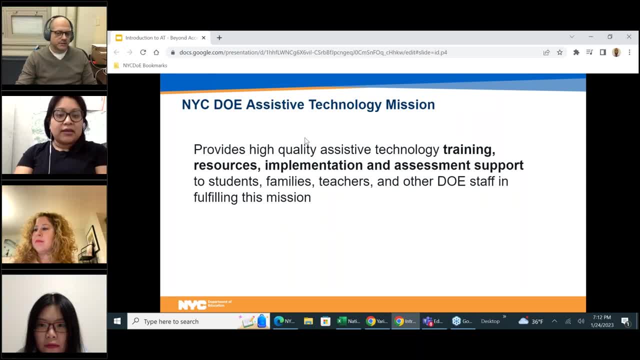 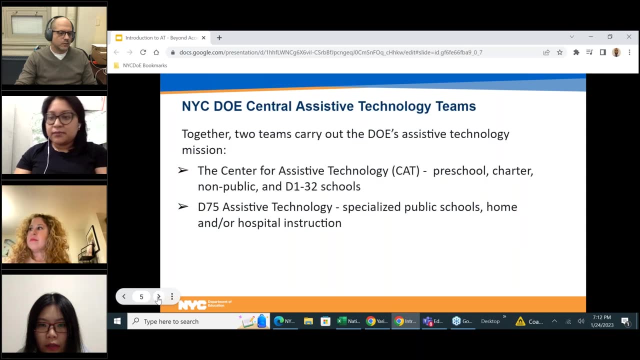 And that's providing high quality assistive technology consultations, training resources, implementation and assessment support to students, families, teachers and all NYCDOE staff. Next slide: The two NYCDOE Central AT teams consist of the Central Assistive Technology Team and they provide support to preschools, charter schools. 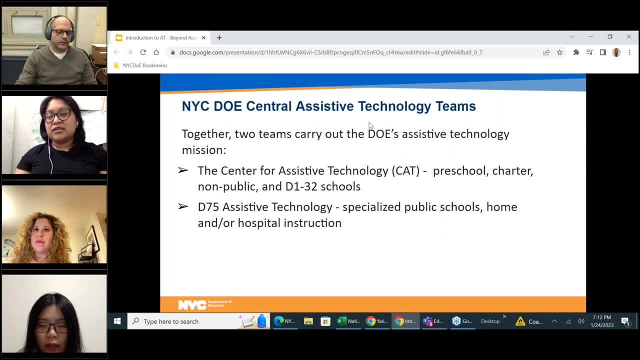 non-public schools in schools within District 1 through 32.. The D75 Assistive Technology Team provides support to specialized schools or District 75, students that receive home instruction services and also students that receive instruction that are in hospital settings. Next slide, please. 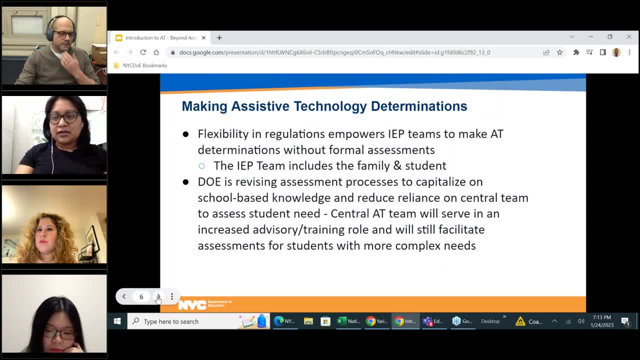 This is. I'm going to read this slide because this is an update to our AT determination process that will have great positive impacts on identifying students that need AT and providing them the tools that they need. So flexibility and regulations. empowers IEP teams to make AT determinations. 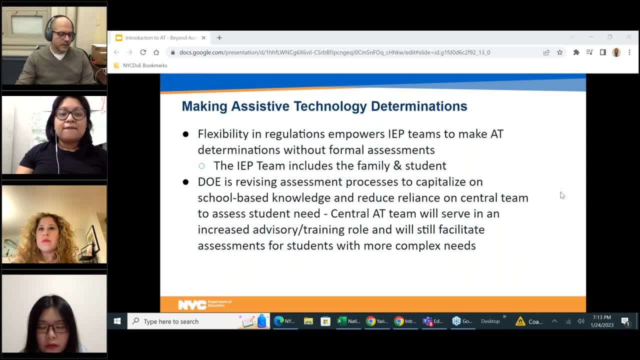 without the need for formal assessments. We want to emphasize that the IEP team includes the family and the student. The DOE and its leadership is revising assessment processes to capitalize on school-based knowledge and reduce reliance on central teams to assess student needs. The central AT team will continue to serve. 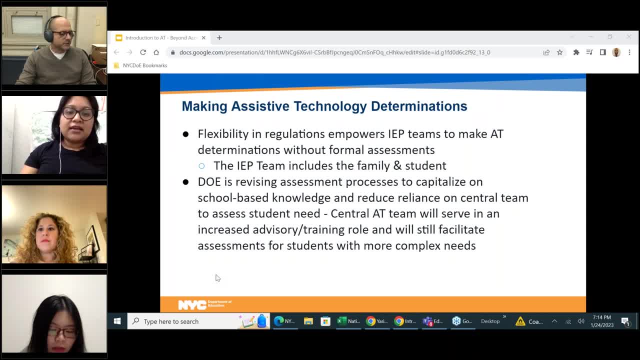 in an increased advisory and training role and will still facilitate assessments for students with more complex needs. We will review these changes more in-depth in future slides, but the updates, including empowering IEP teams, with the exponential growth in technology in schools since remote learning and blended learning of March 2020,. 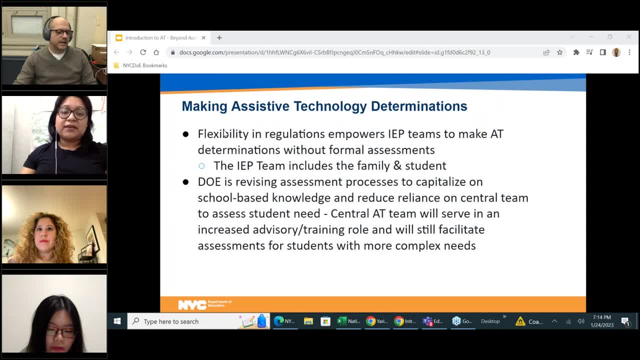 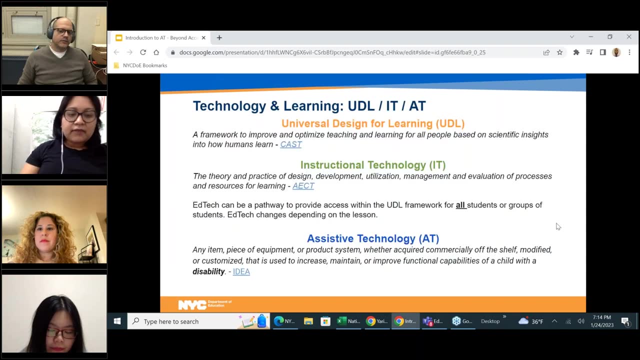 will ultimately expedite the process in identifying the AT needs of students and providing students with the AT solutions they need when appropriate. Next slide: In the next two slides we will focus on the relationships and differences of universal design for learning instructional technology. 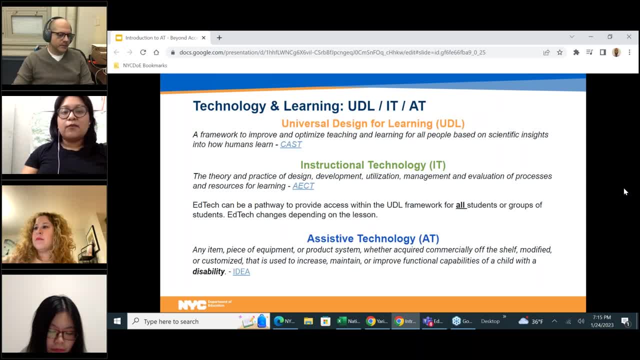 and assistive technology and how these impact the learning environment. UDL is a framework in which the goal is to remove barriers to learning and the focus is on the whole class, not the individual. If an environment, such as a classroom, is designed with all users in mind, 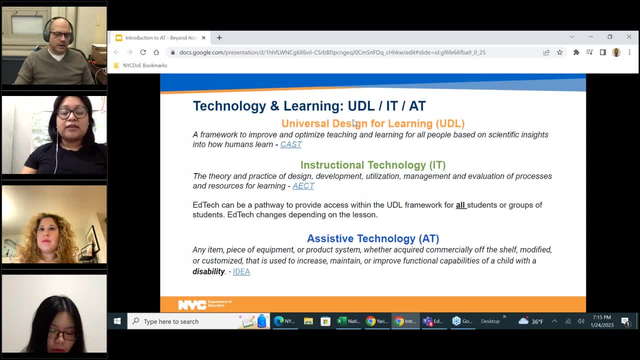 then most students will be able to access learning opportunities. This is the goal of UDL Instructional technology, again as IT. As with UDL, IT is focused on all students and designing lessons with resources for learning such as using computers, tablets and software programs. 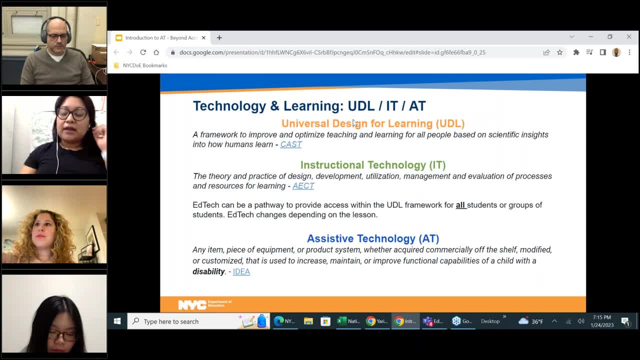 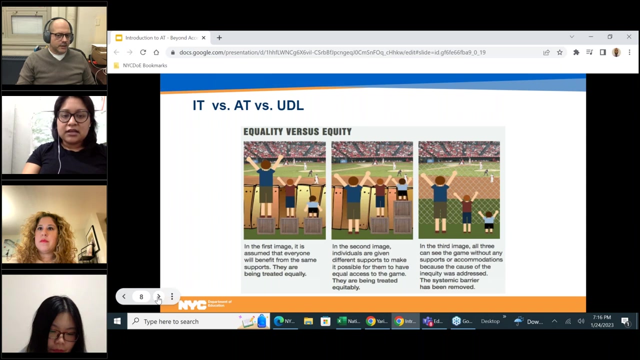 and the resources can change depending on the lesson. Our focus: assistive technology- what we're discussing today is focused on supporting the individual needs of the student, not the group. Next slide: So this is a good visual demonstrating the difference between IT, AT and UDL. 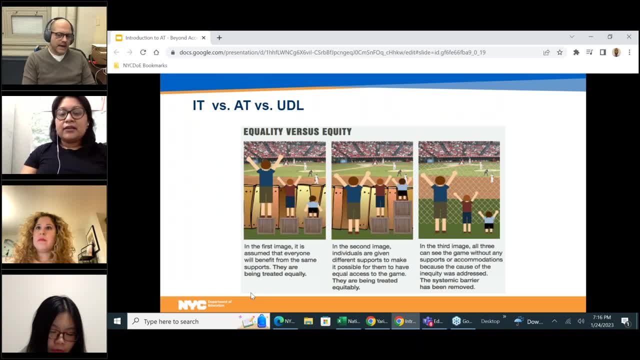 The baseball game is synonymous with the student's ability to access the curriculum and classroom learning opportunities, or, in this case, a baseball game. The picture on the left is an example of instructional technology. All participants have been treated equally by providing them with a crate. 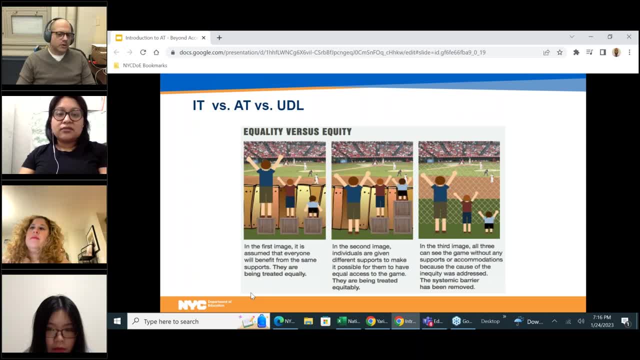 If we focus on the student on the right, we notice that even with the crate, the student is not able to access the game. The second picture is an example of assistive technology. The individuals are provided supports based on their need to be able to access the learning opportunity. 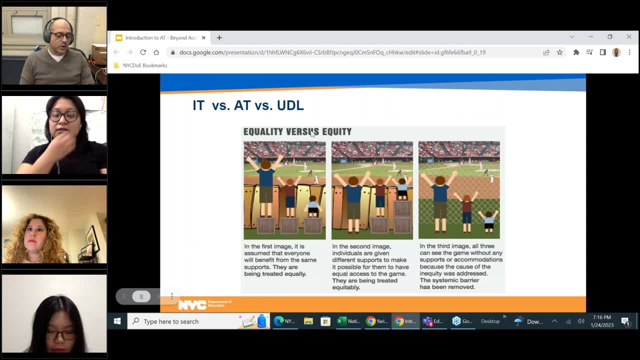 The third picture is an example of universal design for learning, where the focus is removing the learning barrier for all students, in this case the fence, which is an important point. Sometimes a student or students may not need additional supports if the curriculum is universally designed. 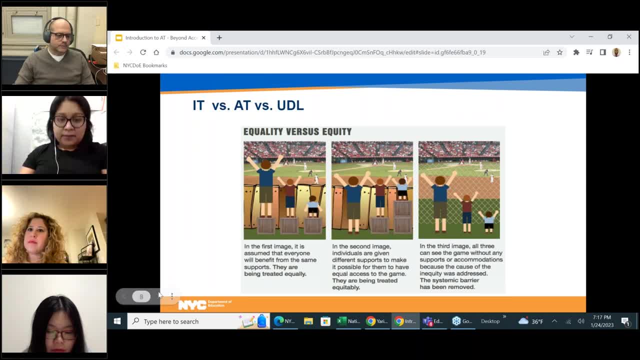 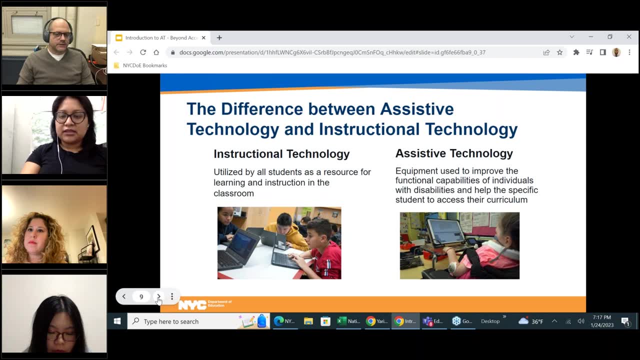 This is the first time we see this Slide. nine Next slide. Thank you, André. In this slide, we're delving deeper into the differences between IT, instructional technology and assistive technology, which can be confusing, as IT and AT involve technology in supporting students. 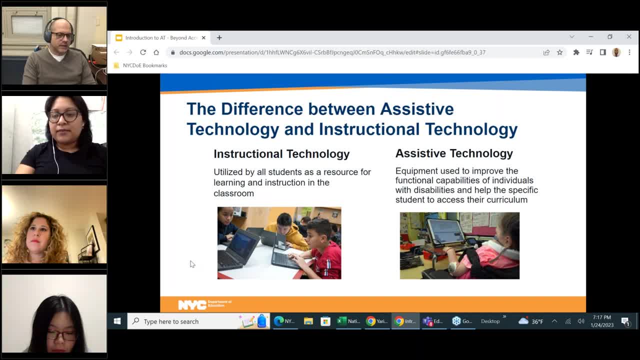 Remember what we discussed in the previous slide: IT, like UDL, is focused on supporting a group- students- where AT the focus is on the individual needs of that individual student. So in comparing the two pictures we see an example of instructional technology on the left versus assistive technology. 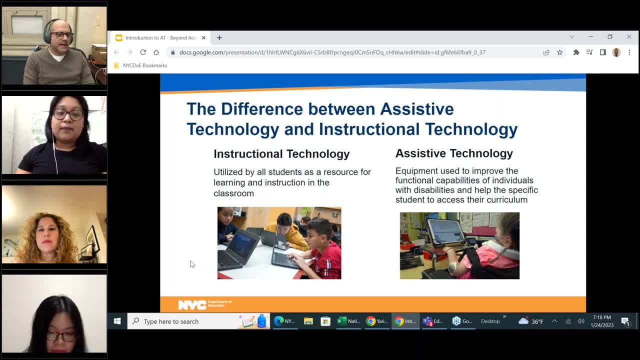 on the right, The difference between IT and AT is determined by what is known as the threshold between benefit versus need. On the left, the students are benefiting from the use of laptops to participate in the lesson, but may- operative word may- may still be able to participate. 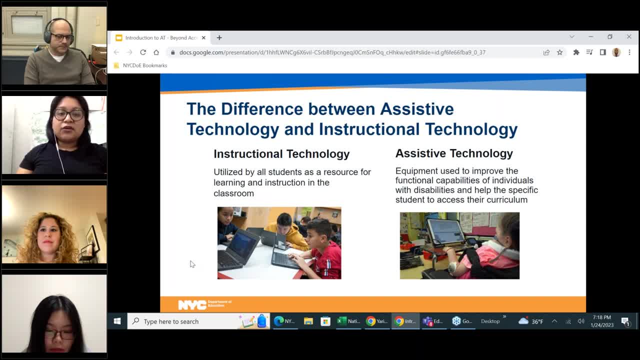 in the lesson even without the laptops, Whereas the student on the right has assistive technology that has been designed for their learning needs. Without AT, the student cannot access the curriculum, be very, very difficult to do so. This is the most important difference between instructional 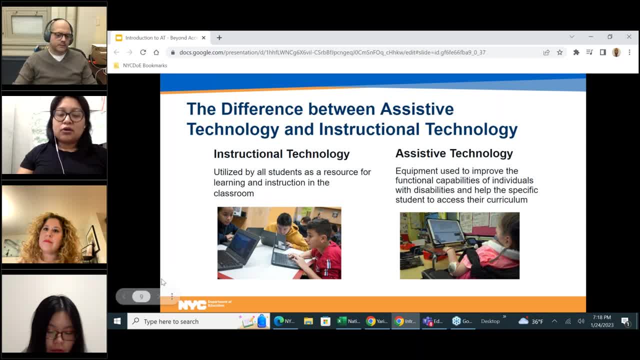 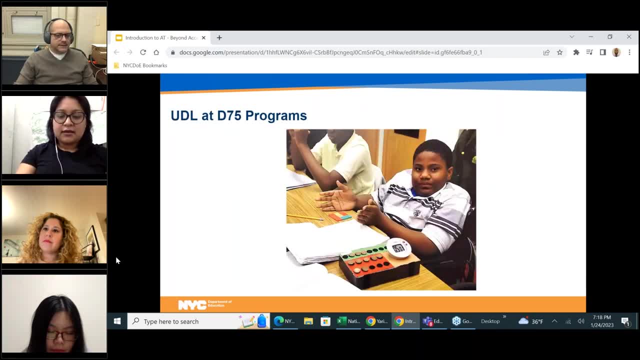 technology versus assistive technology- Next slide. So this is an example of a student participating in District 75 classroom that is incorporating universal design for learning principles. The student is participating in a math lesson with fractional tiles, So they have some tactile ability to participate in this lesson. It is a hands-on or tactile activity. 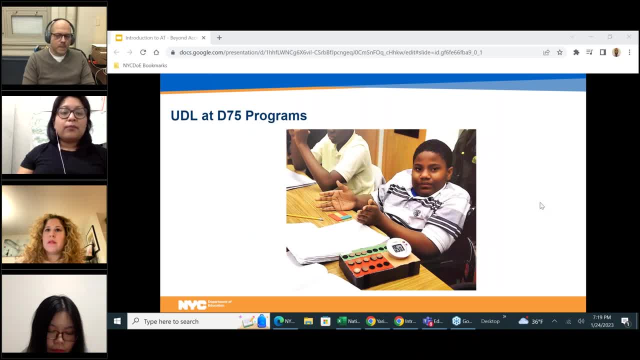 that provides low-tech solutions to access learning. Hands-on activities, both low and high-tech, offer a way to understand abstract context. With some adaptations and thoughtful strategies, math, literature, history and other subjects can be presented in ways that make the 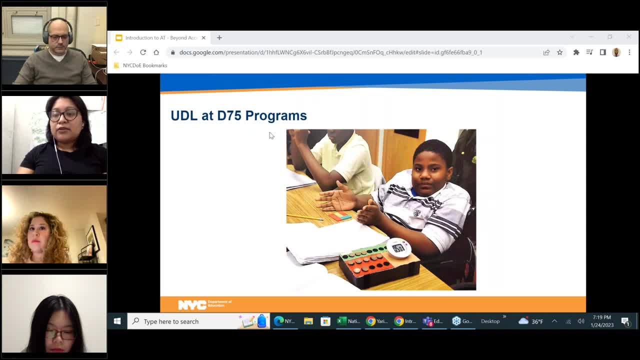 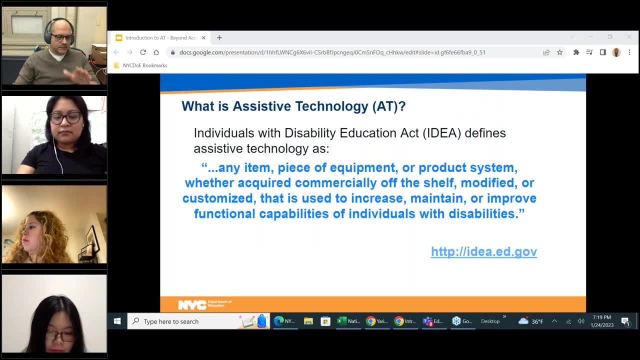 information more accessible. So this is an example of a student participating in District 75 classroom that is incorporating universal design for learning principles- Next slide. So thanks to Suzanne. She helped us define assistive technology right from the beginning. But we're just going to reiterate or remind people with this definition. 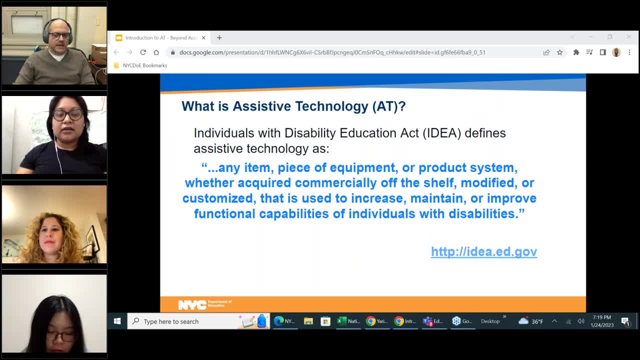 So, according to the Individuals with Disabilities Education Act, which again is a federal law that supports students with disabilities, AT is any piece or item, piece of equipment or product system, whether acquired commercially, off the shelf, modified or customized, that is used to increase. 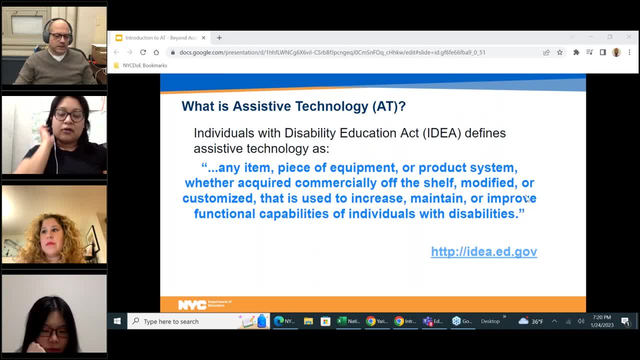 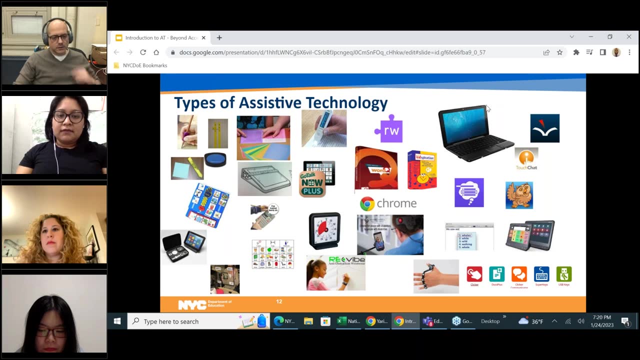 maintain or improve functional capabilities of individuals with disabilities. Next slide. Thank you, Andre. So here we provide some visual representations of AT or assistive technology, from low-tech to high-tech options. Low-tech options can be simple, requiring little maintenance. 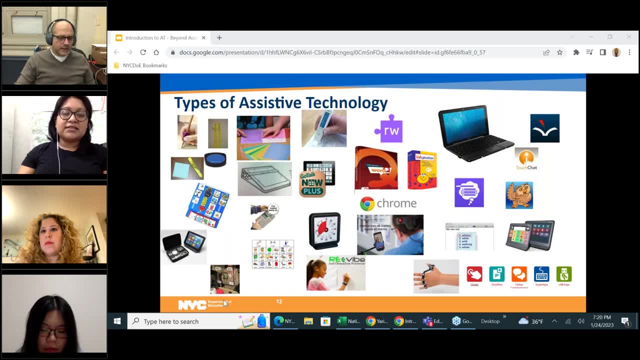 I think on the top left-hand corner, if you can see there's a pencil grip there- where high-tech options can be sophisticated communication devices and are more complex and require support and training. But we do want to note since March 2020,. 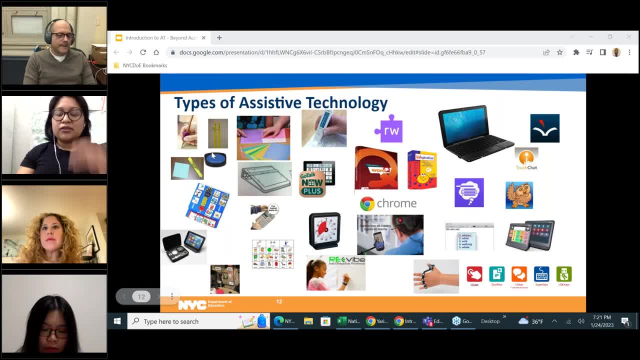 and the introduction of remote and blended learning. many devices, as the parents will know, on this call, such as tablets and computers- that's once required a formal assessment for assistive technology- are now available programmatically or school-owned devices in schools. 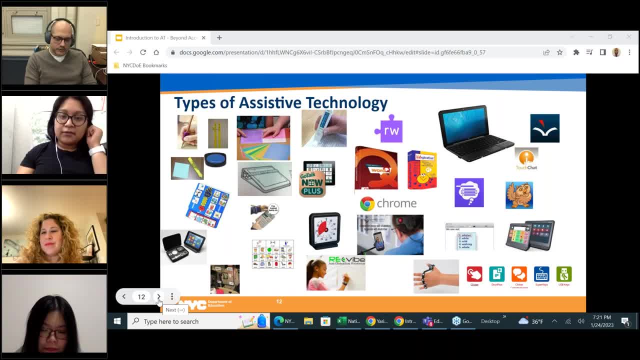 If an IEP team- and we'll touch upon this throughout the presentation- if a need is identified by the IEP team, these devices- programmatic or school-owned devices- can be assigned to a student as assistive technology and reflected on the IEP. 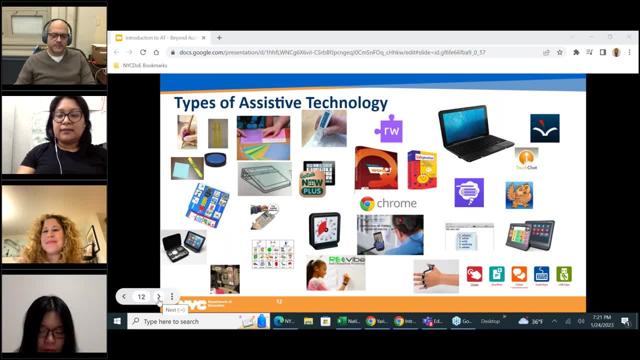 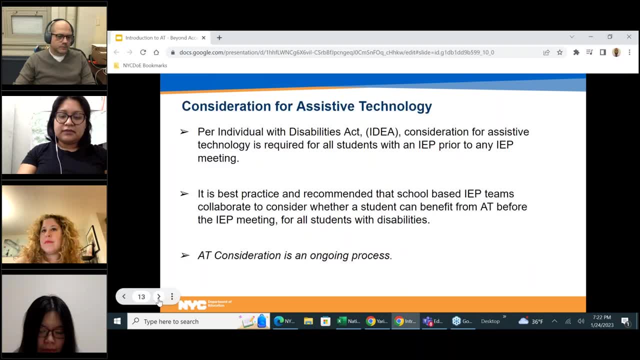 if it is identified again as a need by the IEP team. Next slide: So we're starting to go into the consideration process for assistive technology. We're referring back to IDEA. So by law, specifically again IDEA. 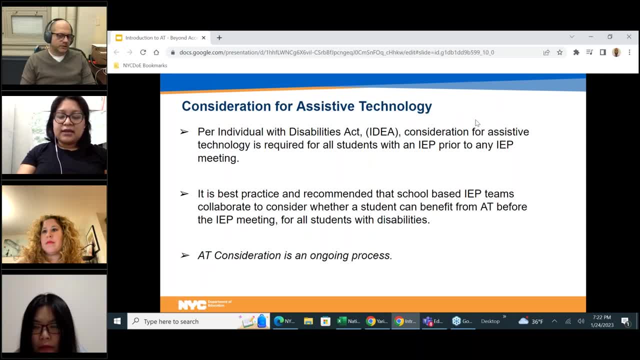 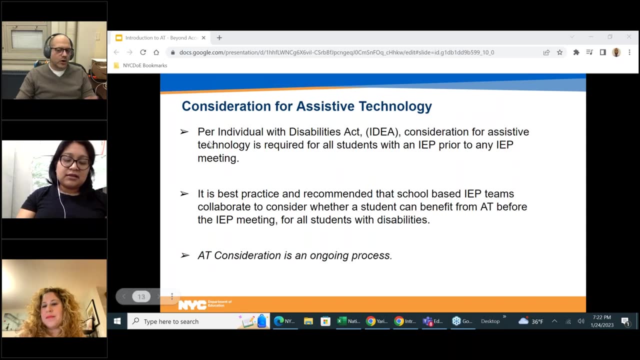 students with IEPs must be considered for assistive technology needs prior to IEP meetings. Just to reiterate: from a best practice perspective, school-based teams should consider the assistive technology for all students with disabilities prior to an IEP meeting. 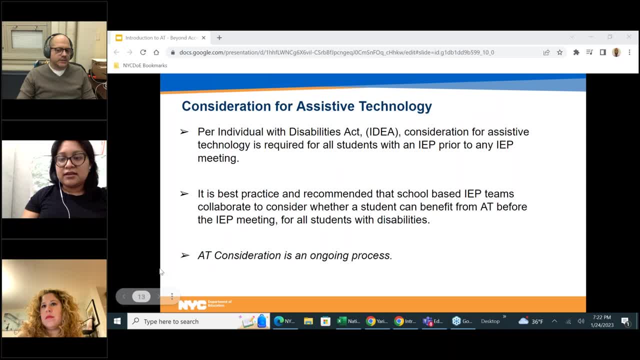 The AT consideration process relies on collaboration between the IEP team members. We want to reiterate again, this includes the parent and the student, And the team should ponder and ask questions such as: can this student benefit from assistive technology to help them meet their IEP goals and access? 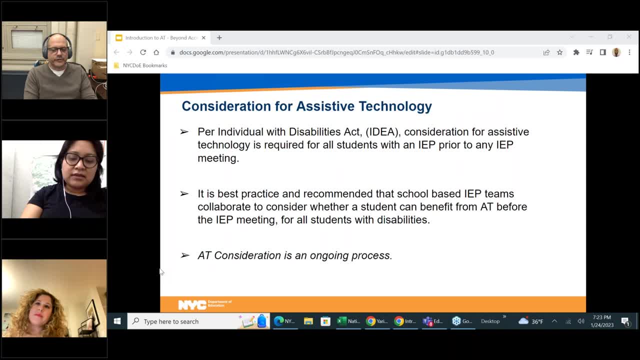 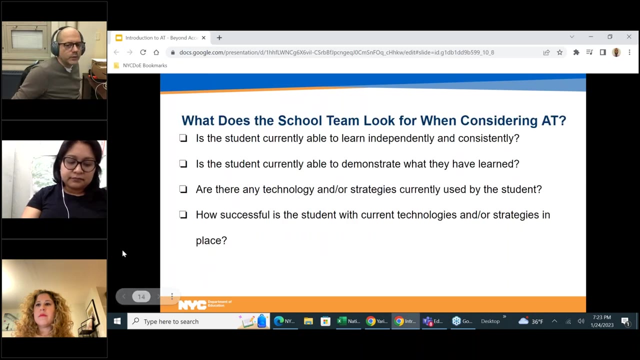 their curriculum. Just a few questions can prompt a conversation that may identify the AT needs of a student, and that's the main goal. As we will refer a few times during this presentation, the AT consideration process is ongoing. Next slide: We have provided here some sample questions that can assist IEP teams in determining. 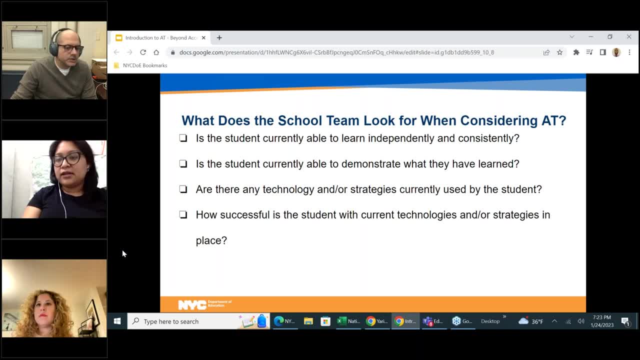 a student's need for assistive technology and we'll go ahead, read each one and provide perhaps a sample response. This could be a plausible response for a student. Is the student currently able to learn independently and consistently? Perhaps the student has a print disability and requires access to accessible digital content? 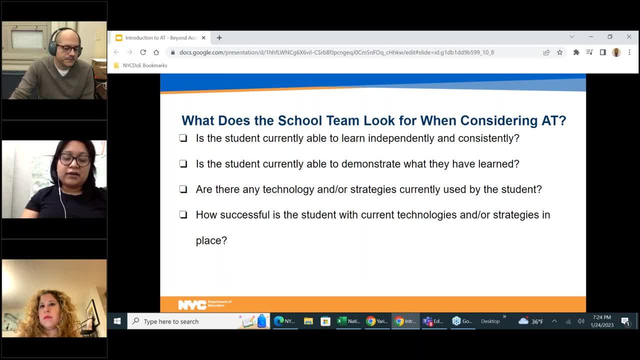 Is the student currently able to demonstrate what they have learned? Perhaps the student presents with communication challenges and may need access to an alternative augmentative communication system. Are there any technology and or strategies currently used by the student? Perhaps the student has access to which we just discussed? 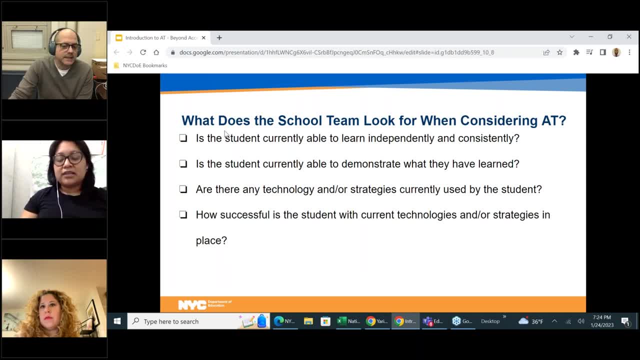 programmatic or school-owned tablets or laptops and needs the built-in accessibility tools such as text-to-speech or speech-to-text to engage in their assignments. Lastly, how successfully is the student with current technologies and or strategies in place? Maybe the student is using a school-owned device and perhaps the student can benefit from specific 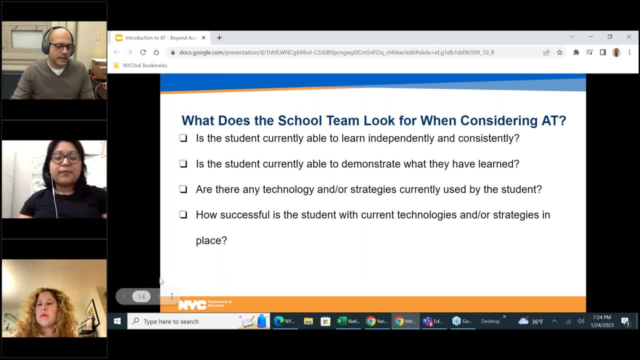 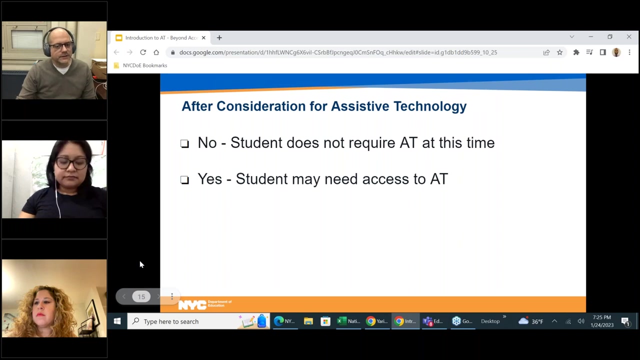 software to assist with the organization. Again, the objective is to ask relevant questions based upon the student's needs and their IEP, and then to determine if the student needs access to assistive technology. Next slide, Next slide. So, after the IEP team considers the needs for assistive technology, 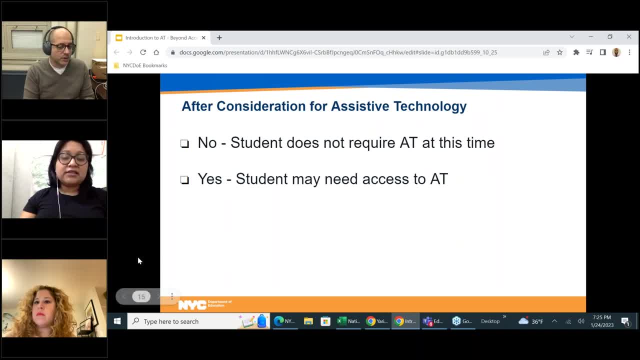 they have to answer this yes-no question. So if it's a no, the student doesn't require assistive technology to access the curriculum. maybe the student may be benefiting from the current structure of instructional technology and strategies provided by their IEP team. 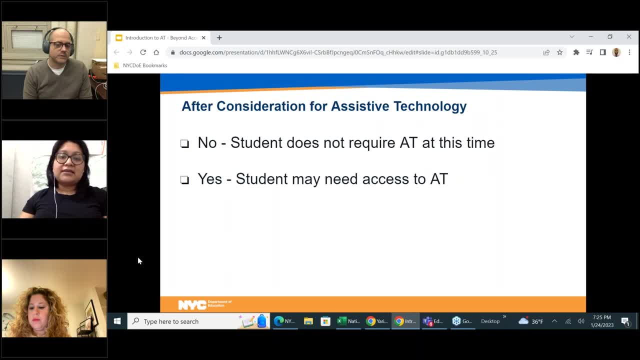 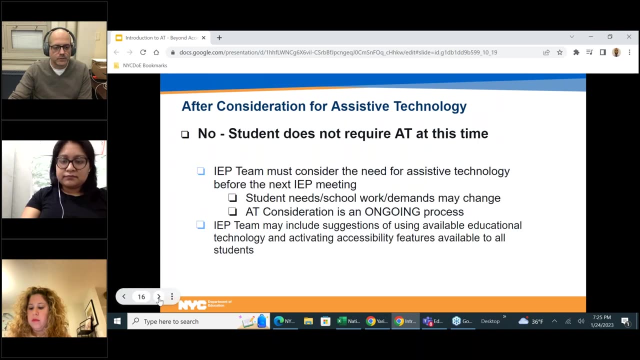 But if Beвед says that also the systems have to accept new and standardized documents, be, there should be a whole new program coming in to the classroom. If the IEP team continues not requiring assistive technology, they will likely do so without the need to have Make-a- sessions. adopt existing documentation, program content or information relevant to coaching and students' needs and does NOT NEED additional supports. and does NOT NEED additional supports. Or the answer is yes, the student may need access to assistive technology supports to access the curriculum. We will get back to this- yes, the YES- in a couple of slides. Next slide: 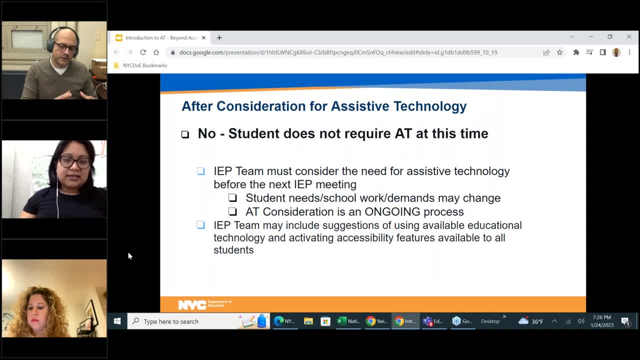 The Yes in a couple of slides, Next slide. So if the answer is no, as we stated previously, it is important to know that even if the IEP team determines that a student does not require assistive technology or technology at work assistive technology, during and before the IEP meeting they must consider the 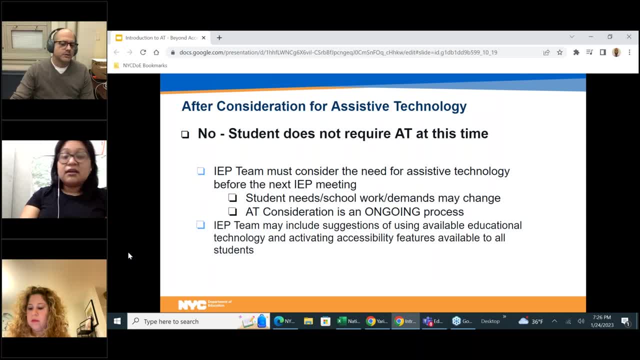 need for assistive technology and subsequent meetings. student needs and expectations change, including work demands, and assistive technology must be considered at a future time. additionally, the consideration process, even if the answer is no, but it still may inform the IEP team to make suggestions throughout that IEP, for example, for the student to use instructional technology. 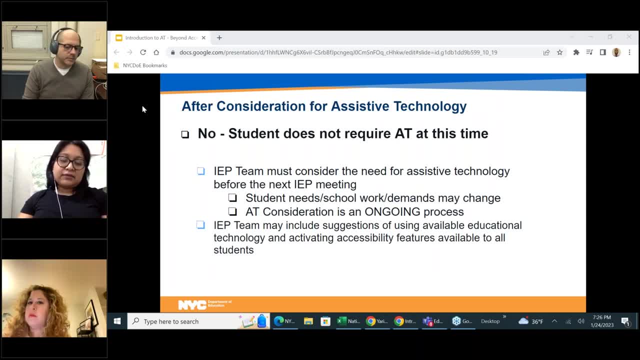 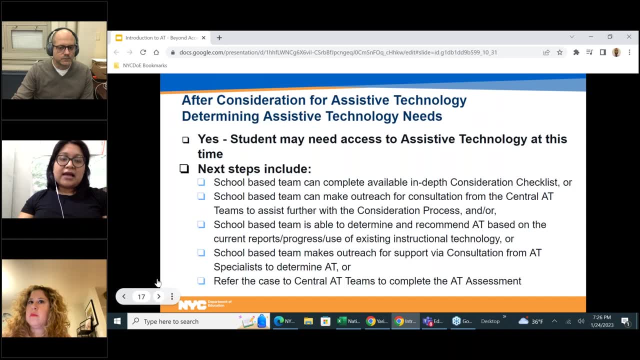 as is stated here, to access built-in accessibility features. let's get back to the yes next slide, please. so if the answer is yes, the student may need assistive technology to access their curriculum. a school team can provide the best possible assessment and guidance to the student. 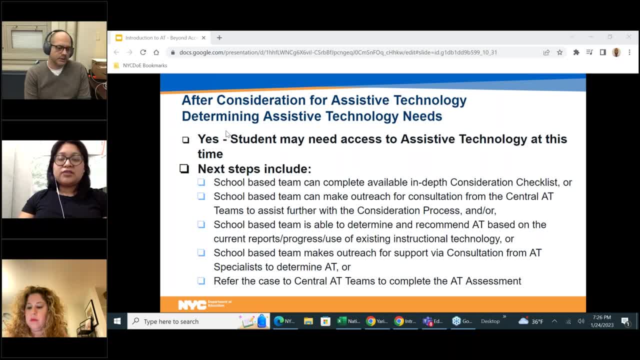 can follow the steps below, based on the needs of the student. This is not necessarily a hierarchical list, So the school team may use the consideration checklist to identify the need and the AT tool required, or the school IEP team can request a consult with one of the central AT teams to assist. 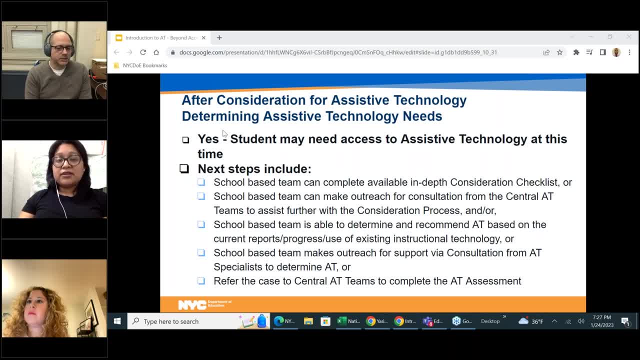 with the consideration process. School IEP teams can use existing IEP team reports in progress to determine the need and AT tools required for the student Or, during the consultation session, the IEP team, in collaboration with the central AT teams, can determine that an assessment is required to determine. 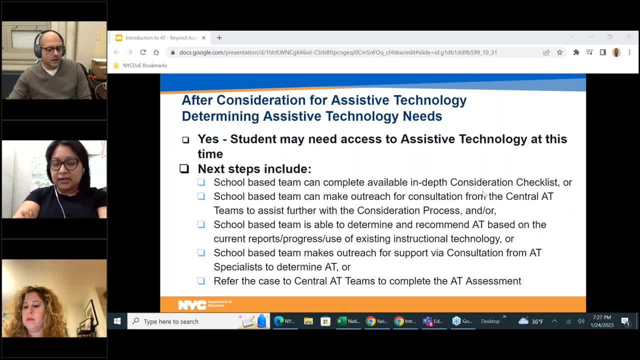 the AT needs of the student. As was stated in prior slides, in many instances- and this is certainly an update that will play out in the future- This will positively impact the ability of students to access AT School. IEP teams are able to make an AT determination. 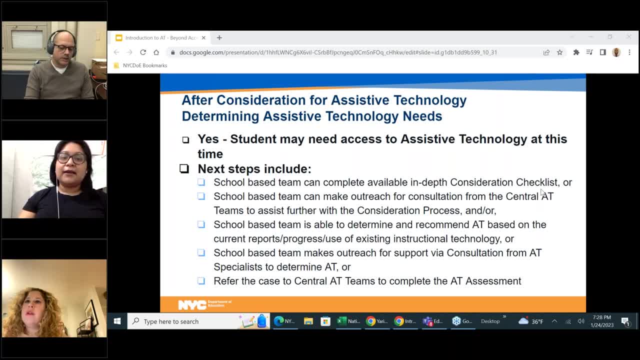 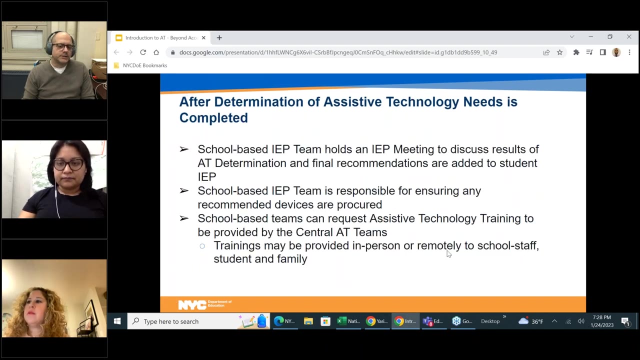 at the school level without a formal assessment or reliance on the central AT teams. This flexibility and regulations allows the school teams to identify the AT needs of students and provide them with the necessary AT resources. Next slide, please. So once a determination has been made, 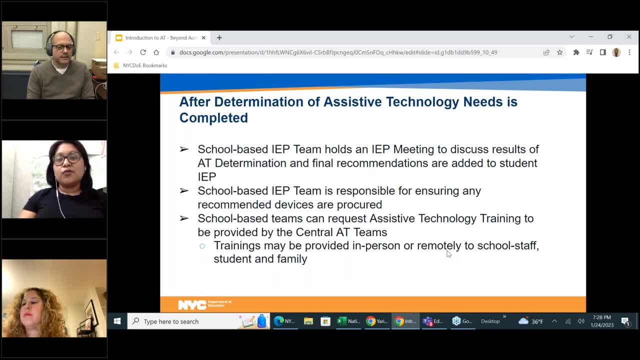 that the student needs AT. what are the next steps? to complete, The school-based IEP team will hold a meeting, an IEP meeting, to discuss the results of the AT determination and the final recommendations are then added to the student's IEP. 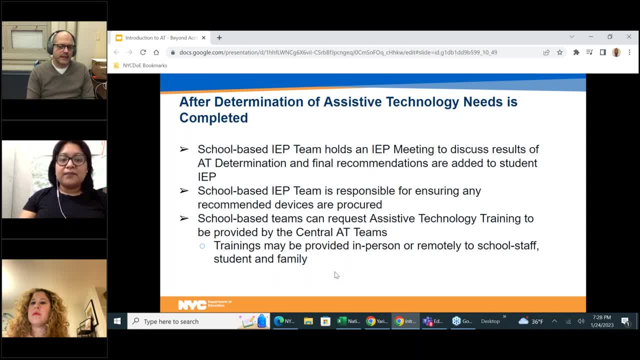 The school-based IEP team is responsible for ensuring that any recommended devices are provided. Central AT teams will be available for ongoing training, implementation and support, and these trainings can be provided in person or remote to school staff, students and family. 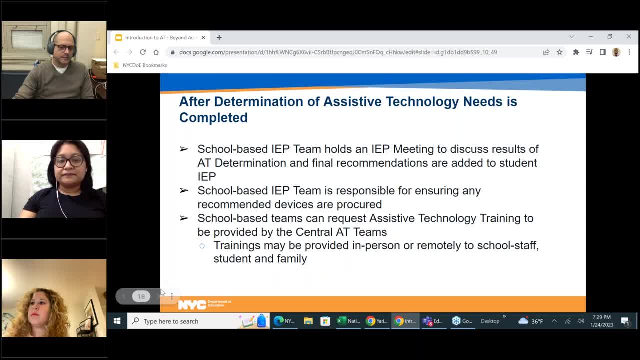 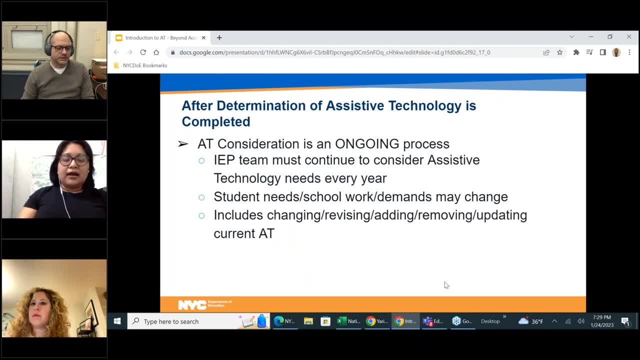 Next slide, please Continuing on. once Assistant Dean's office is completed, the student's IEP team will start identifying and leading the teams into the IEP meeting. This is recommended by the IEP teams so that the student needs to include AT needs. 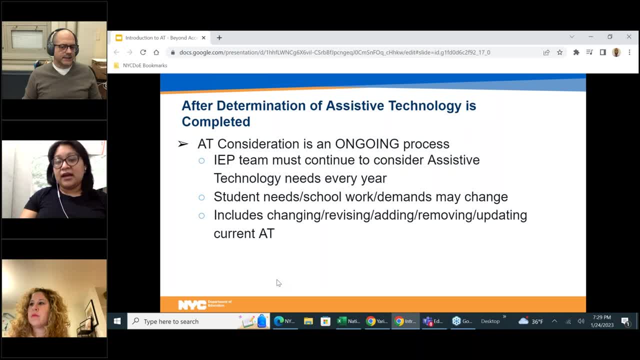 in all of their IEP meetings. Therefore, it is a benefit for each student. as a result of the IEP meeting with the student, The IEP team is working to roll out a comprehensive IEP to greatly improve the performance of student. student improvement in the student's IEP. 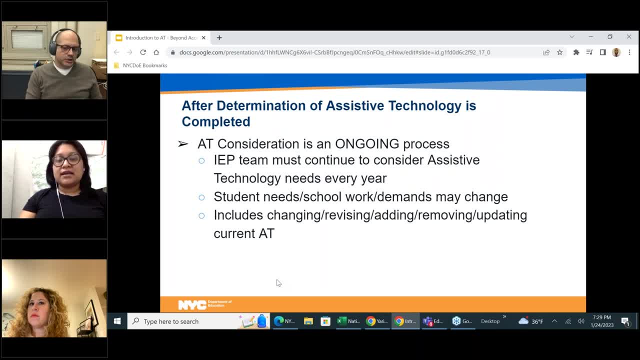 As the student's IEP team continues to review the tasks and potential IEP requirements, these changes and consider the needs of the student. they may require an updated program to assist with reading and writing or a more robust alternative augmentative communication system based on progress that they've made. we 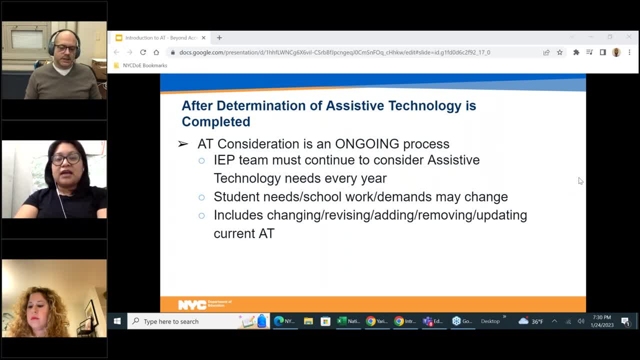 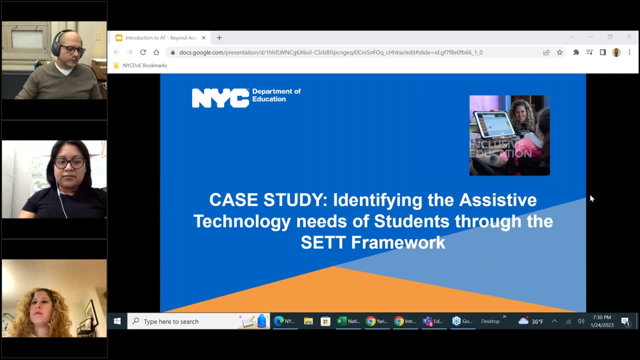 encourage parents to talk to their school-based teams to continually review the assistive technology needs of their children. next slide. next I will pass the presentation on to Lindsay Huntley and she's going to be discussing this case study and identifying the assistive technology of students through what's called the set framework. Lindsay, Thank You, David. next. 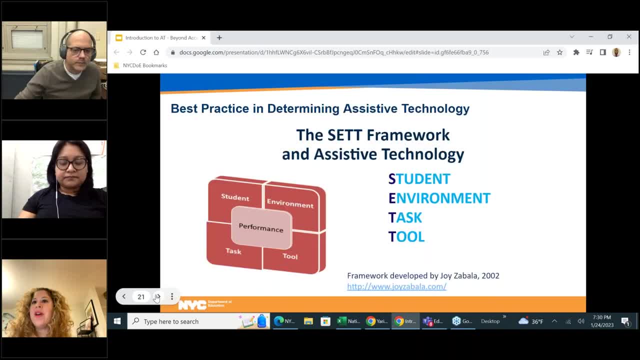 slide please. so best practices in determining assistive technology is we eliminate the need for students to use assistive technology in the classroom? look at the set framework and assistive technology. there is no standardized assessment for assistive technology and, as a David discussed, there's lots of. 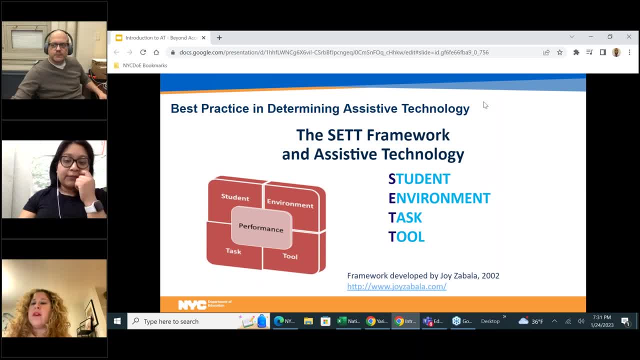 ways that we can determine what a student needs, and one of them is to look at the student, the environment, the task and this tool. so we want to know what can the student do with it out technology and what can't they do without technology. so, for example, if a student is having trouble with a 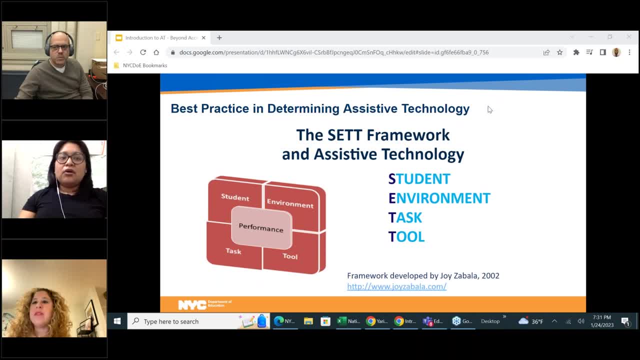 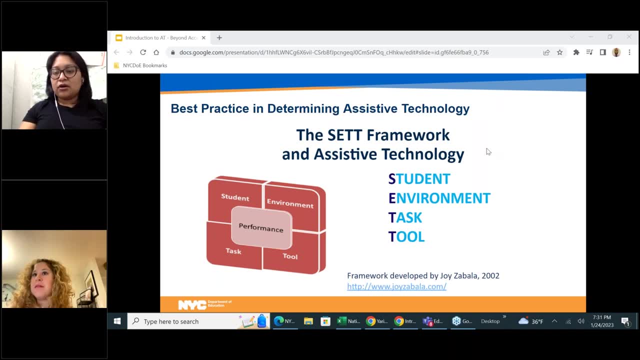 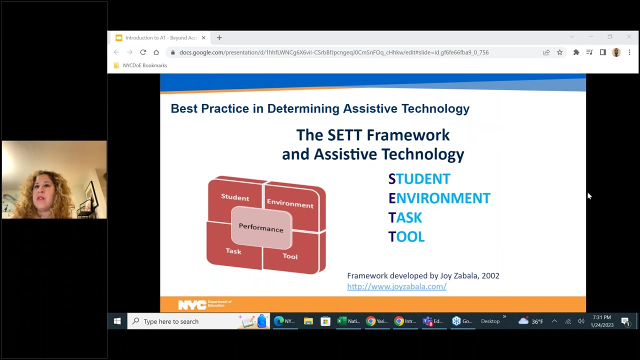 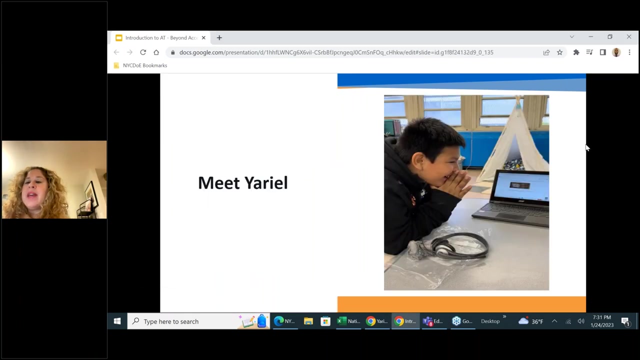 writing plan this time, and they need to be Ав acha from a Chrome IDE system. this time it's best to try something similar that you can find on nine to determine what will benefit the student to access their curriculum Next slide. So we're going to meet Yariel. This is a case study we're going to share with you. 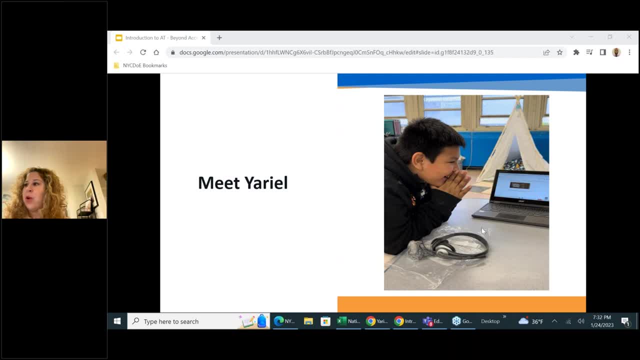 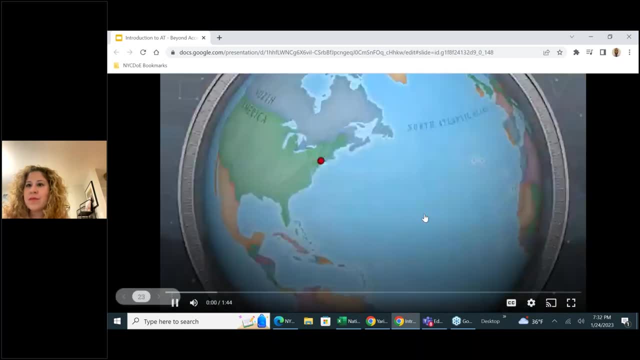 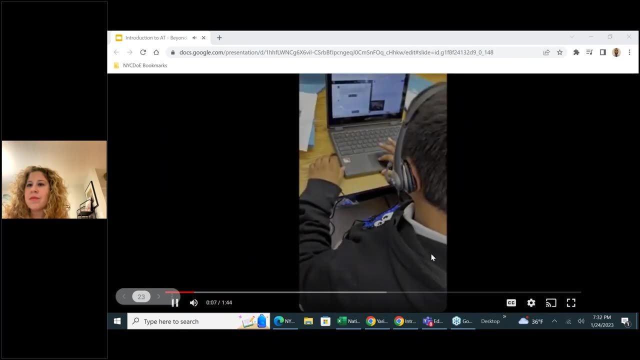 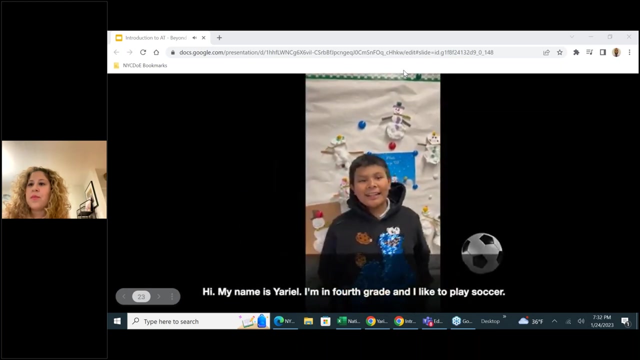 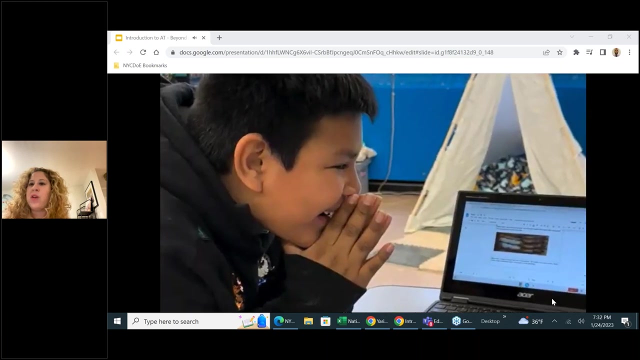 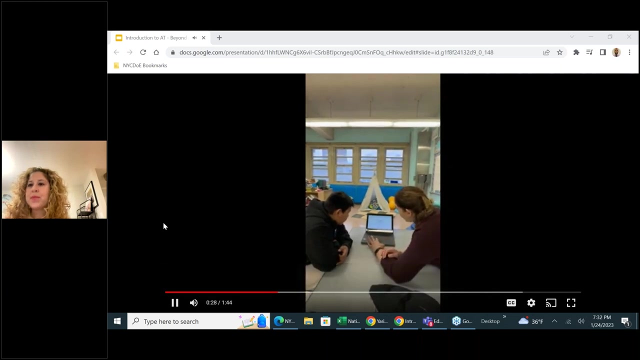 and we're going to show you a fabulous video. I hope it plays Next slide, So this is just showing you Yariel as we the day of his assessment and training at his school. There was supposed to be some music, but it's not working. We apologize. 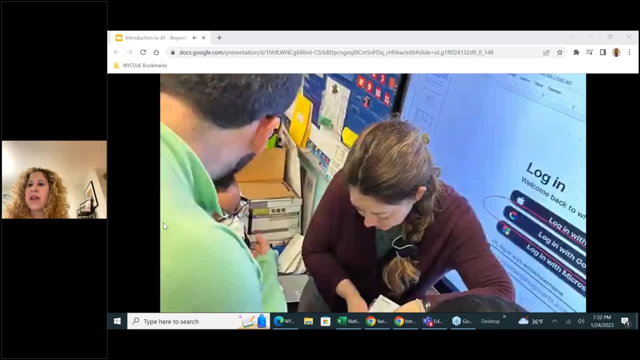 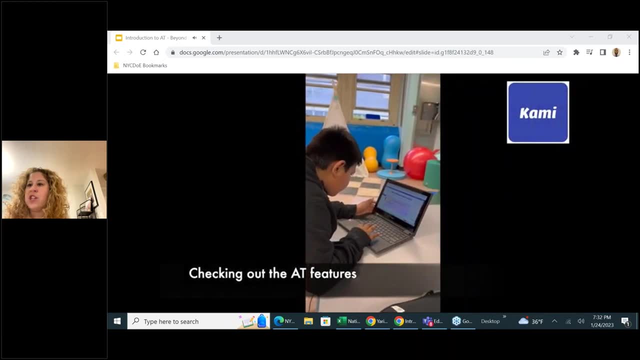 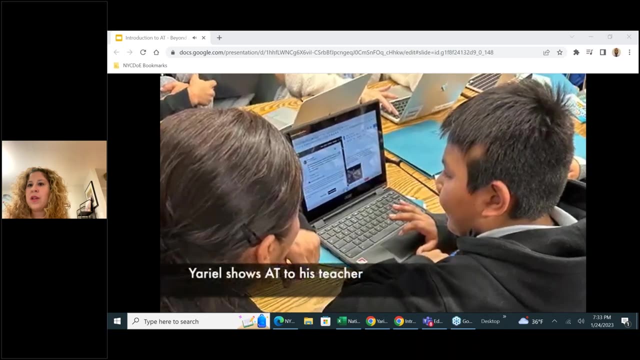 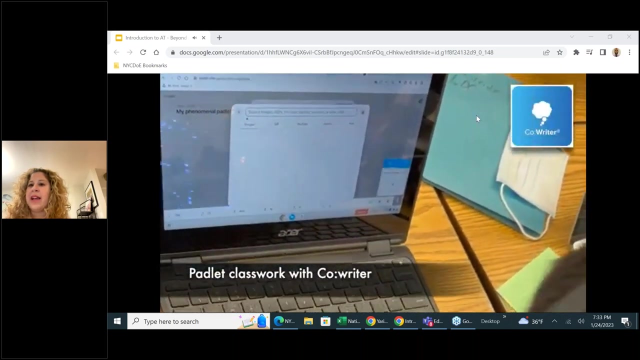 Next slide. So here he's using a scanning pen, He's using a laptop and looking at the AT features and Kami, He's showing his assistive technology to his teacher. He's using Padlet classwork with co-writer, and we'll explain this in the further the next slides. 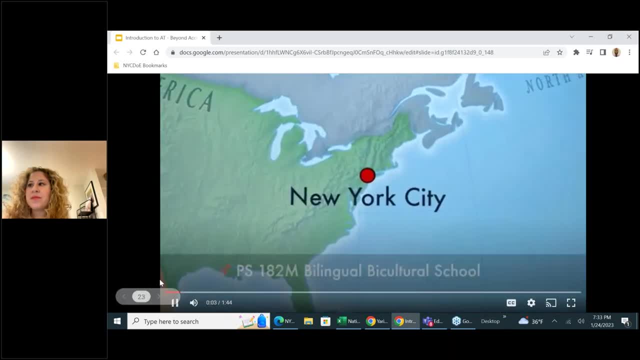 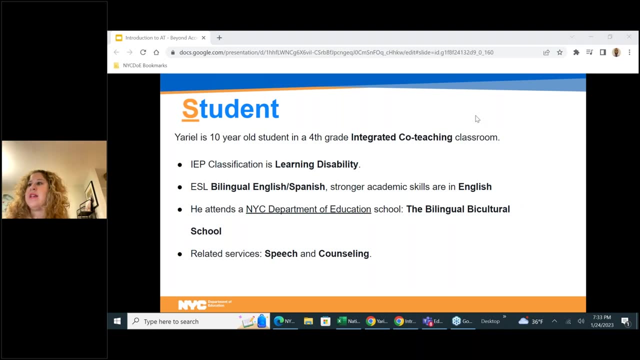 So now we're going to look at the set framework. So the student, Yariel, is a 10-year-old student. He's in fourth grade. He's in an integrated co-teaching classroom. His IEP classification is learning disability. He is bilingual in Spanish and English, and he has 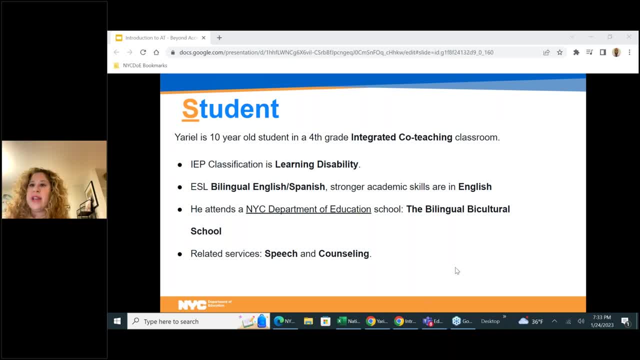 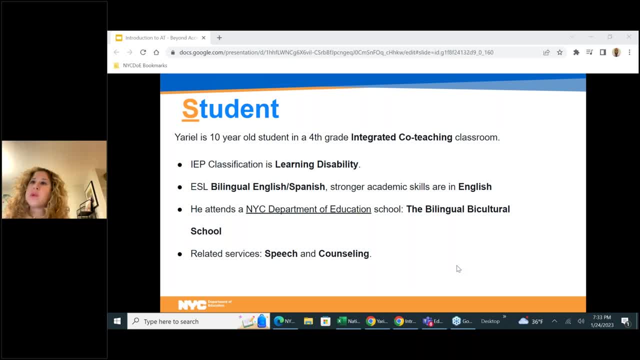 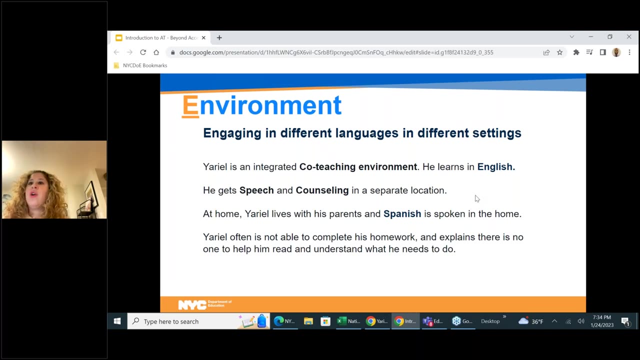 subur elementary school called the bilingual, bicultural school, And his related services that he receives are speech and counseling. So when we were looking at the environment and trying to determine this assistive technology, we wanted to engage in different languages and different settings. Yariel is in an integrated 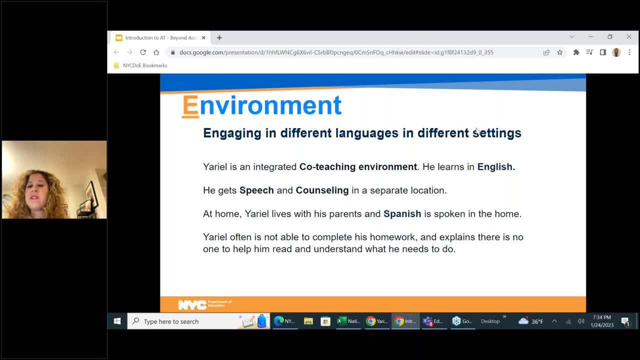 co-teaching environment. He learns in English, he gets speech and counseling in a separate location, and at home he lives with his parents and Spanish is spoken. so he's often not able to complete his homework as there's no one to explain to him at home or help. 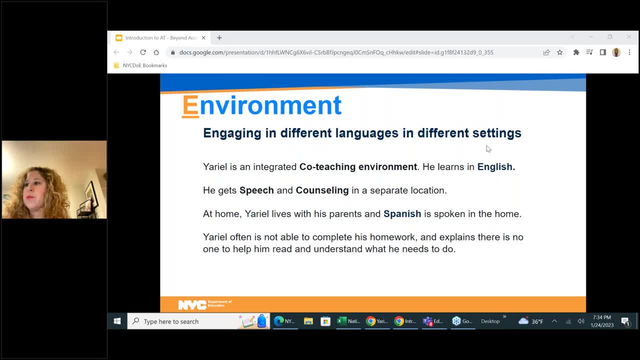 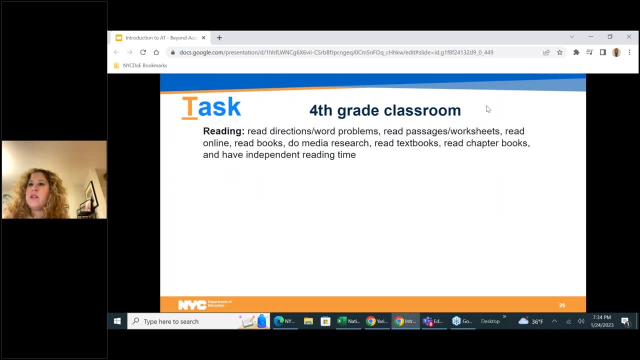 him to read and understand what he needs to do. next slide, please, so if you can. there's more pop-ups in that slide, please, so I guess keep clicking. yep, want two more times, thank you. so when we're looking at the task, the fourth grade classroom. so for reading, the student has to read directions, word problems, read. 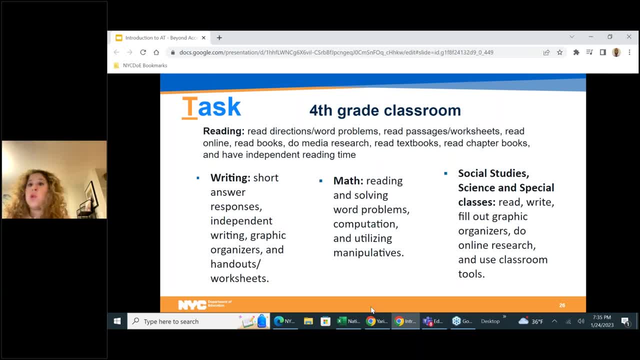 passages, worksheets, read online, read books through media research, read textbooks, read chapter books and have independent reading time. that's what he has to do in reading in writing. he's responsible for short answer responses, independent writing, graphic organizer and handouts and work and sheets and math. he needs to read and solve word problems, do computation and 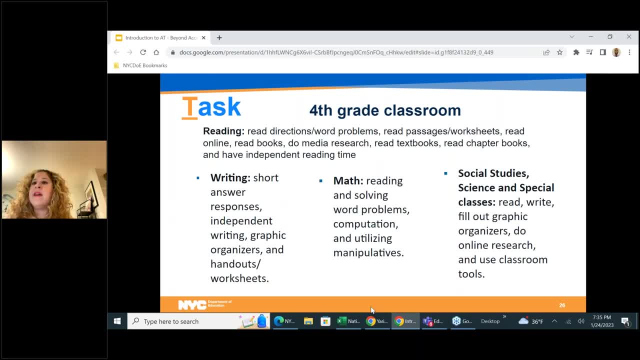 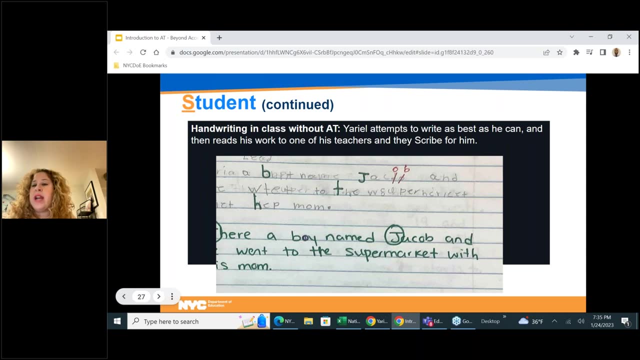 utilize various manipulatives and in social studies and science. he needs to read, write and fill out graphic organizers do online research and use classroom tools. next slide. so here you can see an example of his handwriting without the use of assistive technology. so we're still looking at the student. the student, Yariel, attempts. 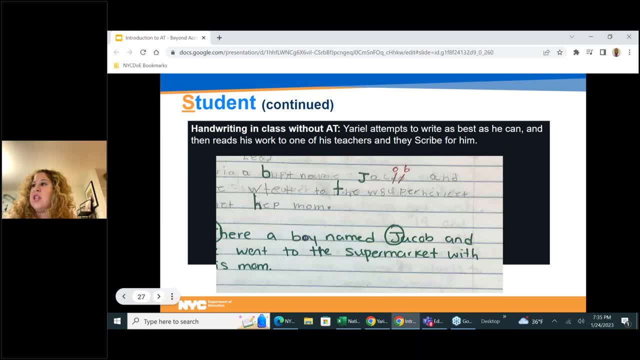 to write as best as he can and then reads his work to one of his teachers. so you can see on top that's what he wrote. and when he was reading it back to his teacher because it's difficult and to read because it's illegible, he read back. 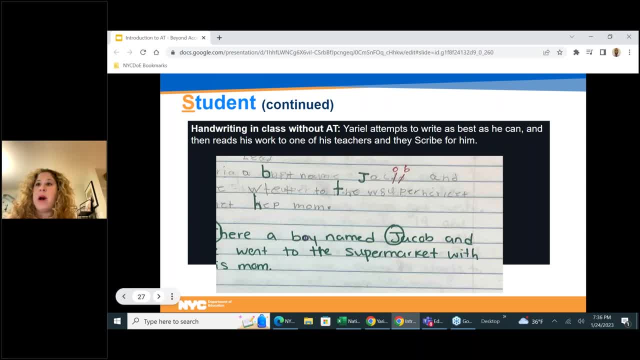 there's a boy named Jacob and he went to the supermarket with his mom. but you in the above sentence. it's very hard for the teacher or unfamiliar people that don't know his handwriting to read what he wrote. now we're going to look at his reading next slide, so if you can click again twice to show the pictures, 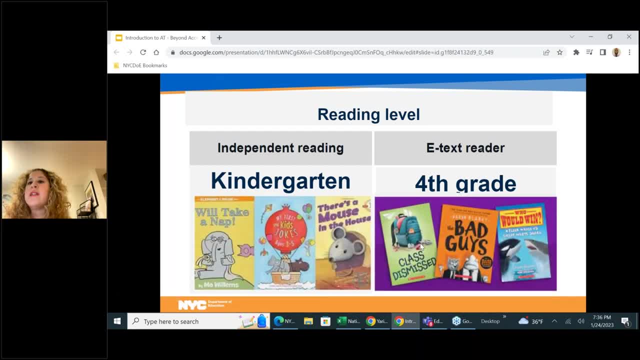 so his reading level: when he was reads independently, without the use of assistive technology, he's reading at a kindergarten level. but when he was read, when he was able to be given the assistive technology with an e-text reader, he was able to read and comprehend and a fourth grade level. so eight. he doesn't remove the learning disability and the outra Content. he does not remove the learning disability and has been able to be developed particularly with a higher level of power and precise communication. tekn 거 brush cars in front of the classroom, C Awards and a total of 26D in her adult learning course within alaska. 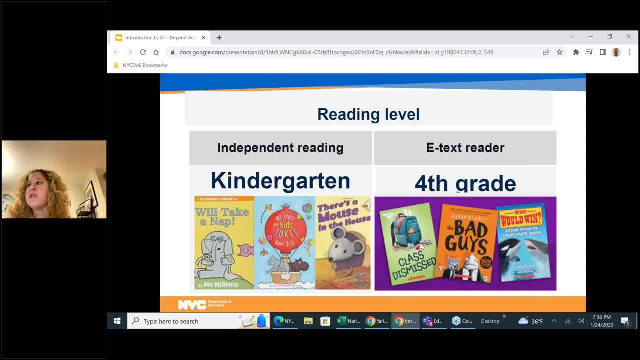 and the student will still need teacher support with understanding and grade-level vocabulary, Additionally needing to support for task-focusing prompts and teacher check-ins. All those things are still important. We don't eliminate all the environmental factors in the student. We will still need to support with background knowledge. 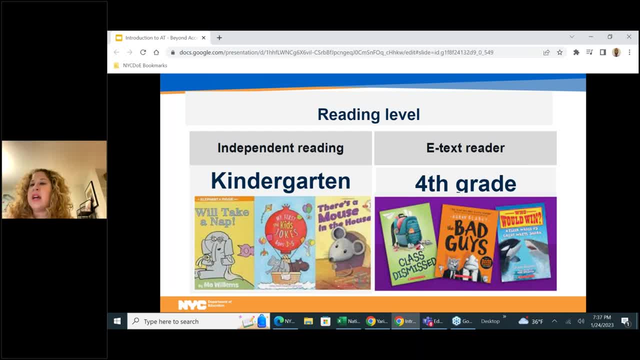 So what we're saying is, with the tool of the e-text reader, we're able to accommodate him in a fourth-grade- you know, fourth-grade- reading level. So it was a huge amount of progress just with the e-text reader. If you can go to the next slide please? 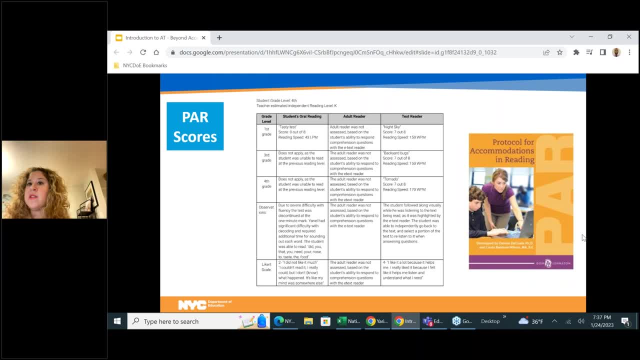 So here we use the protocol for accommodations and reading. This is a tool we use to assess how Yariel does with reading when using an e-text reader. So, basically Based on interviews with his current special education teacher, Yariel's reading benchmark is at level one which was below grade-level standards. 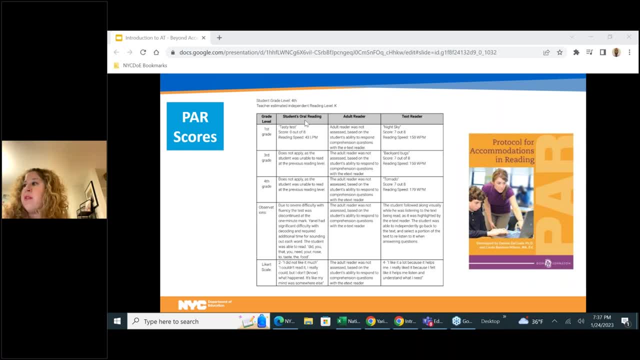 And the student is reported to be reading at a kindergarten level using Fontas and Pinnell as an assessment tool. He has been receiving reading intervention at the school using the recipe for reading and Orton-Gillingham approach to phonics and decoding fluency, comprehension and vocabulary or factors. 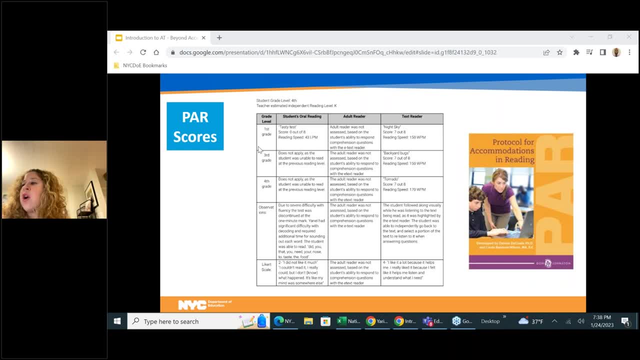 that most impact Yariel's reading. So current interventions that the school was doing already was they were doing a reading intervention program. They were visualizing questions read out loud, and guidance and prompting And students were expected to follow reading materials in the classroom. 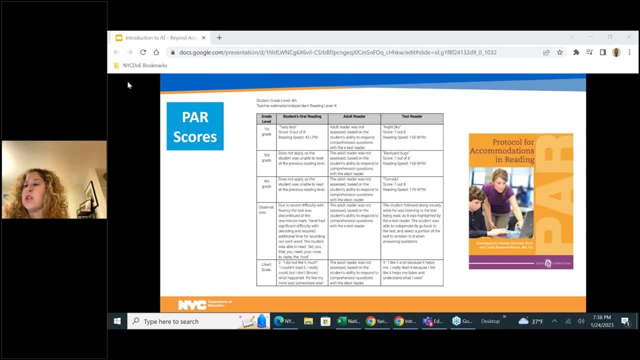 such as reading directions, word problems, read passages, worksheets. So Yariel had difficulty doing all these expectations without the use of assistive technology. So then we tried him with various tools. So if you can go to the next slide, please, 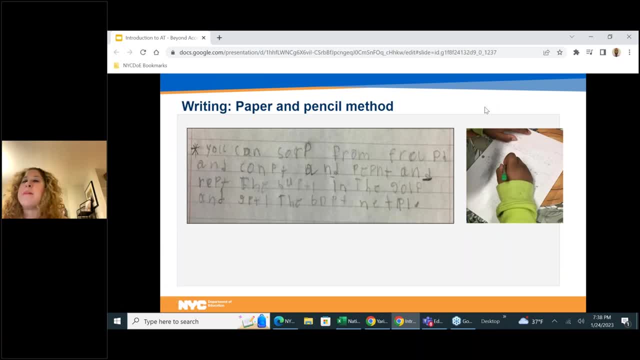 Here he is without his assistive technology, writing with paper and pencil. You can see his handwriting up top. It's a little bit illegible. And he, when he read back to the evaluator what he was trying to write, he wrote: 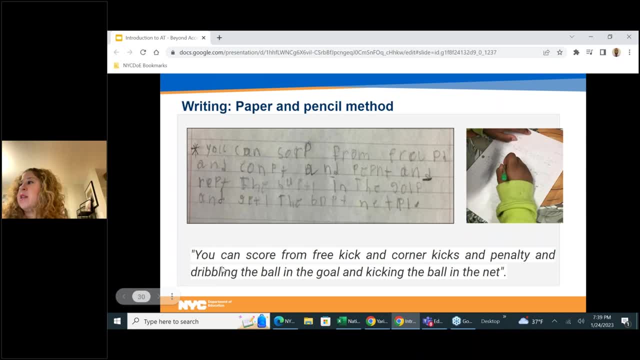 you can score from a free kick and corner kicks and penalty and dribbling the ball in the goal and kicking the ball in the net. But it's very hard to read that due to his illegible handwriting, So we provided him with assistive technology. 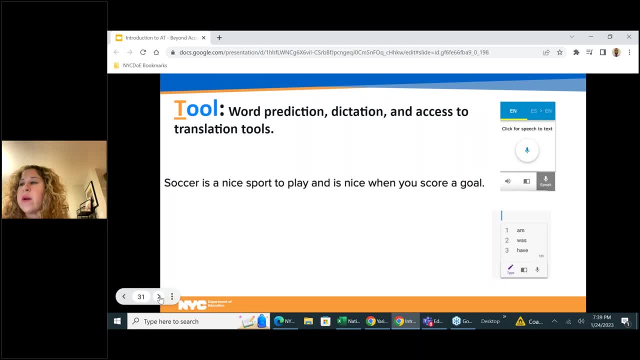 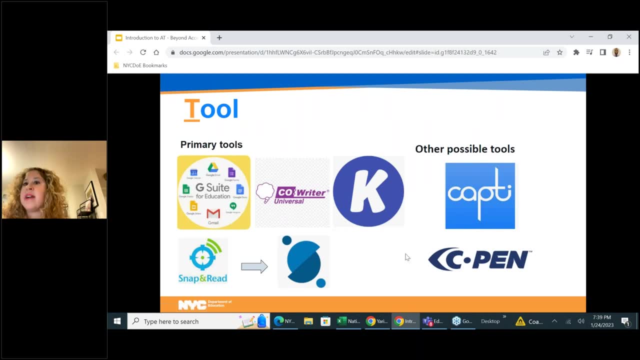 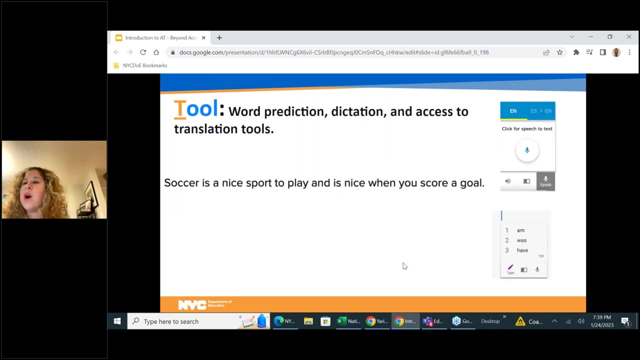 And if you can go to the next slide. The tool that we provided him had word prediction dictation, so he can speak what he wants to say, and access to translation tools. Can you go to the previous slide please? So just using it one time he was able to write. 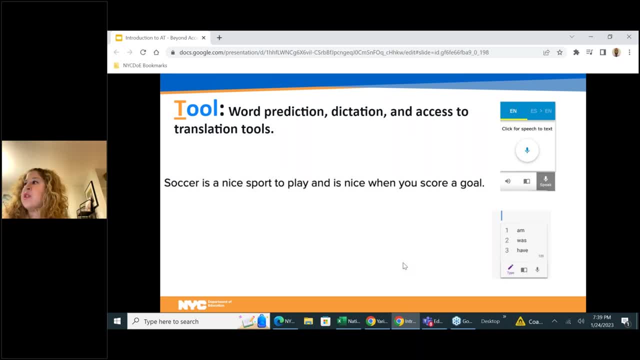 soccer is a nice sport to play and it's nice when you can score a goal. So it was a more complex, better syntactical structure to his sentence. just from using the tool one time- And this was the day of the evaluation or when we came in- 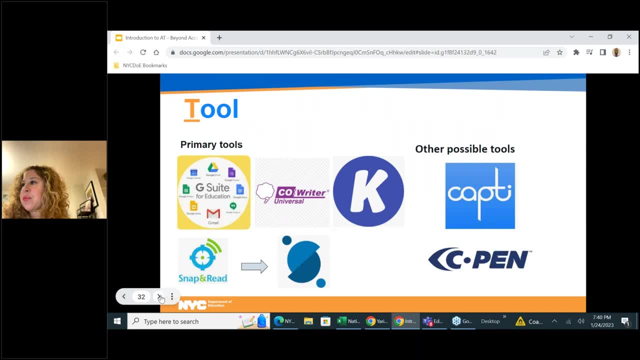 Can you go to the next slide please? Okay, So these are the tools that we recommended for Yariel to use To access his curriculum. So one of the primary tools is G Suite for Education, which is a universal design for learning tool because all our kids have access to it. 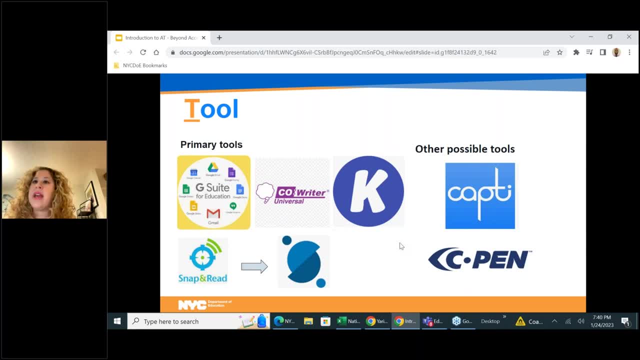 We also recommended Co-Writer, which was the tool that gave him word prediction, dictation, support for writing, Kami for annotation and Snap and Read so he can take notes And other things we looked at were Capsy and if you saw on the video, 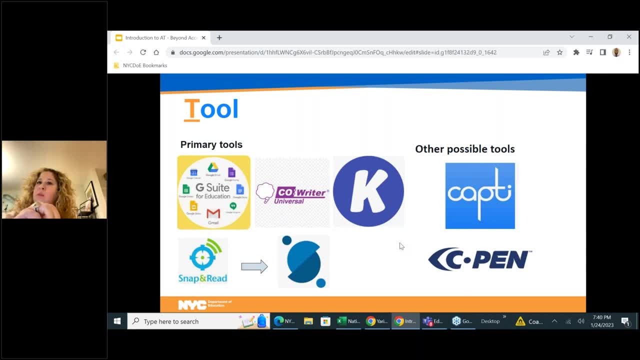 there was a C-Pen. it kind of looks like a highlighter and when he puts it over the text it will read it out loud, it will define a word and it will translate in Spanish if he needed support. So now we're going to do a brief overview of our assistive technology toolkit. 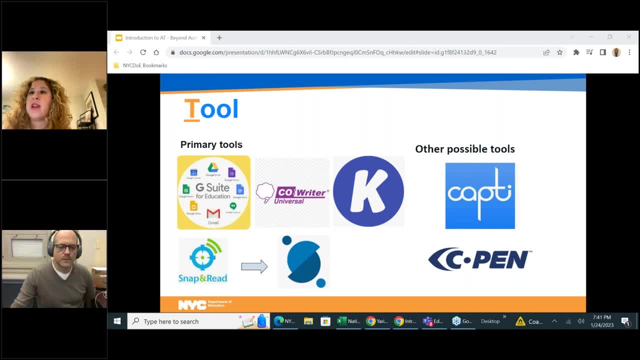 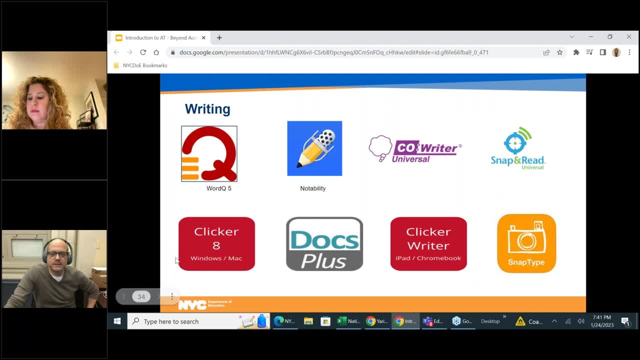 Yep slide after that. So, as Lindsay was alluding to, we really do have access to an extensive library of assistive technology supports. We're going to start with writing, So we're providing you just an overview of some of our most recommended AT writing supports. 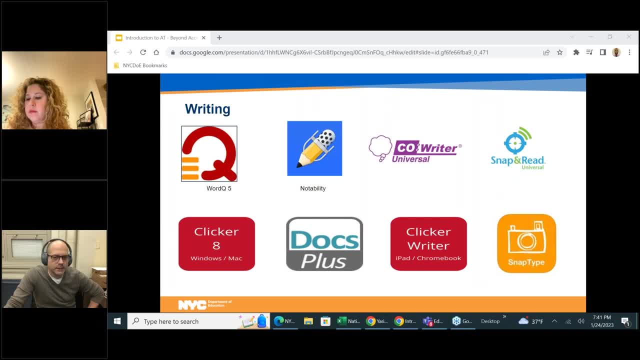 highlighting Notability, which is the icon in blue, which is an Apple-based program that works on Macs and iPads. It's basically like a note-taking device- the name is Notability- and allows users to quickly create and edit notes by dragging and dropping documents, photos or audio recordings. 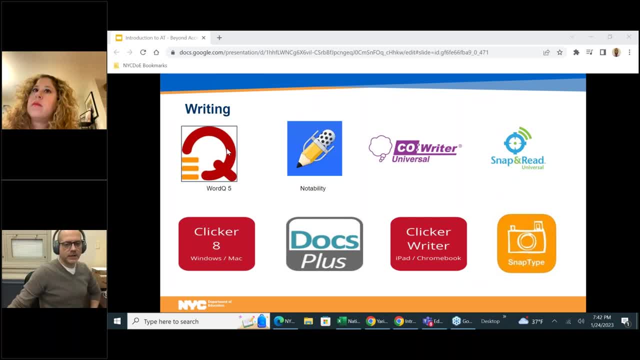 Co-writer, which was one of the apps that Yariel was recommended for, is a universal and cloud-based program. Co-writer helps students write with proper grammar and spelling, using topic-specific vocabulary And, as we saw with Yariel, co-writer assists with predicting the intended word with a selection. 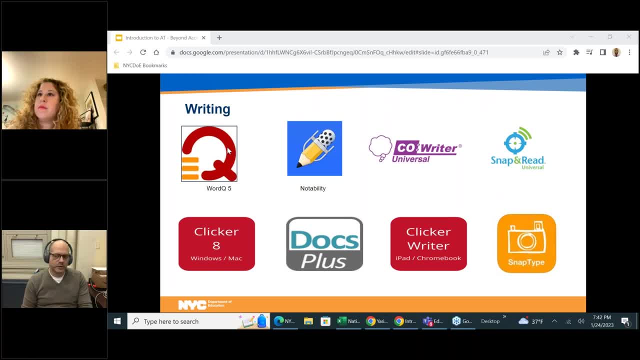 of word suggestions using what they call grammar-smart word prediction. SnapType Pro is an interesting and simple app. Yeah, It's available both on iOS and Android devices. so basically, students who struggle with graphomotor skills, who have messy handwriting, they can use SnapType Pro and they can take. 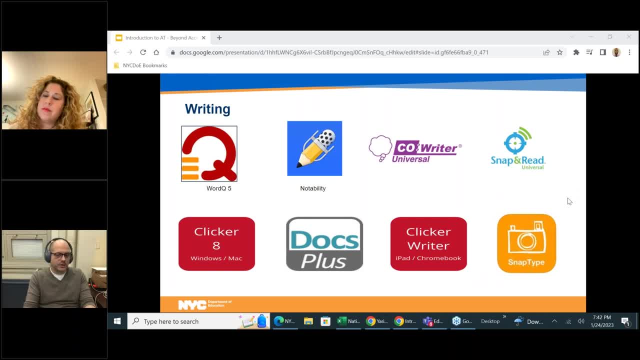 a picture of any test worksheet or piece of paper, and then the student is able to use that app to type on the digital copy instead of having to handwrite, And then they can share their work with teachers and peers. Okay, So the bottom three icons, Clicker 8, Docs Plus, Clicker Writer- these products belong. 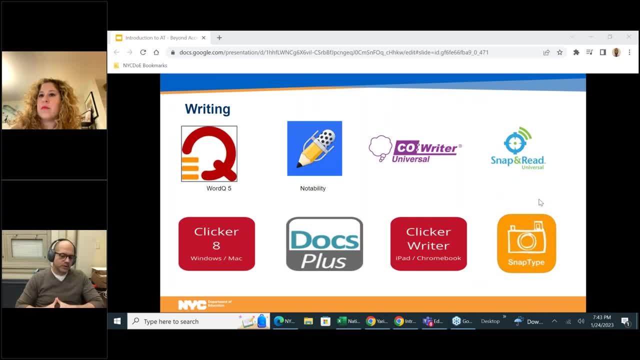 to a suite of software programs from a company called Crick Software, which happens to be some of our most recommended IEP-mandated assistive technology tools to support writing and reading as well. I know we're focused on writing now And they can support students that are at that early literacy level. 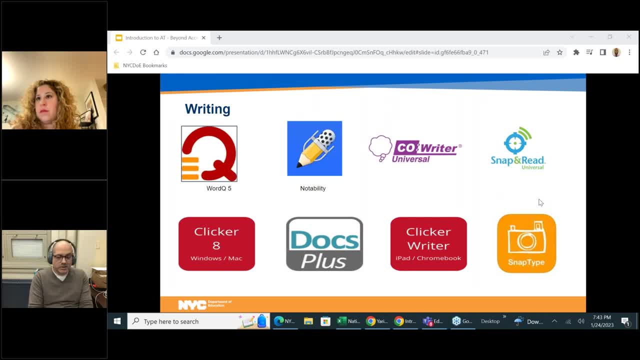 Who may need things like sentence starters. to students who have some physical access issues and they may require switches. to students who maybe are participating in standardized assessments, who may require some simple supports like word banks or organization pages. Next slide. Next slide. 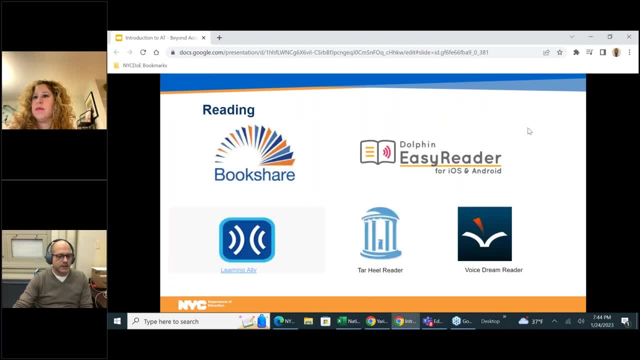 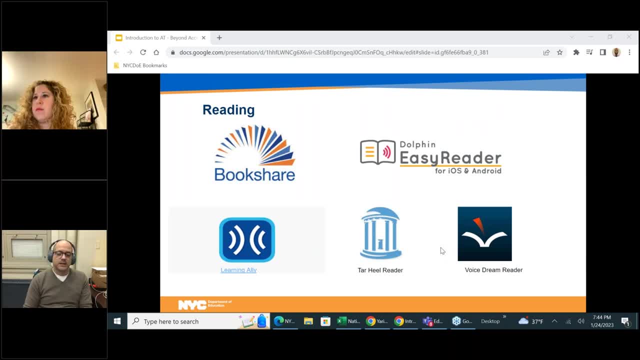 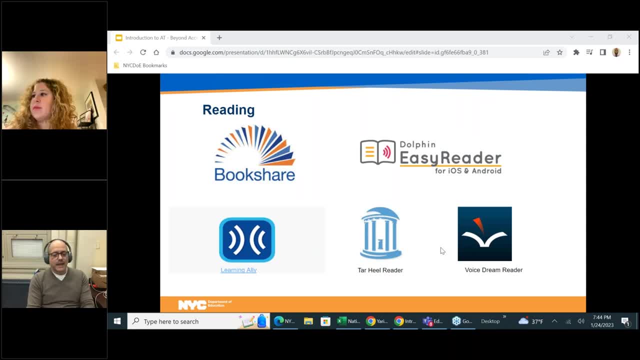 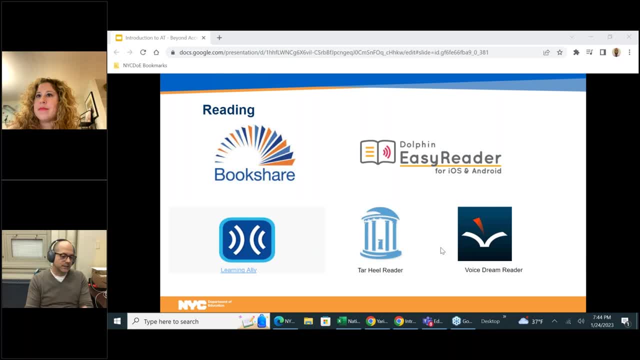 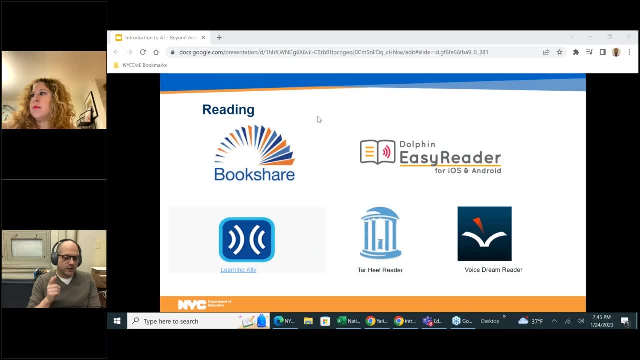 is really Learning. Ally has human-read audiobooks, and so both of these- Bookshare and Learning Ally- can support students with learning disabilities that are impacted by challenges with accessing physical print. okay, and they may need access to accessible digital content. Dolphin EasyReader. 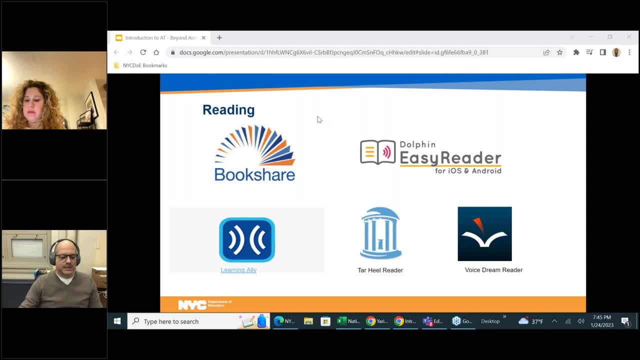 and Voice Dream Reader. These are some of the apps that we use to actually access the content of Bookshare, and so these are designed again for those students with print disabilities, such as dyslexia, low vision, blindness, learning disabilities- Both of these reader apps- 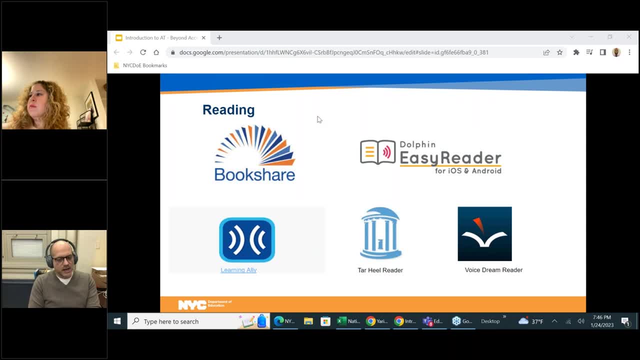 Dolphin EasyReader is free. Voice Dream Reader is not free, but it's still a product or software solution that we recommend for students, and we have Luke Martin I COAPS, and both of these reader apps are customizable for the user, So you're able to change the text. 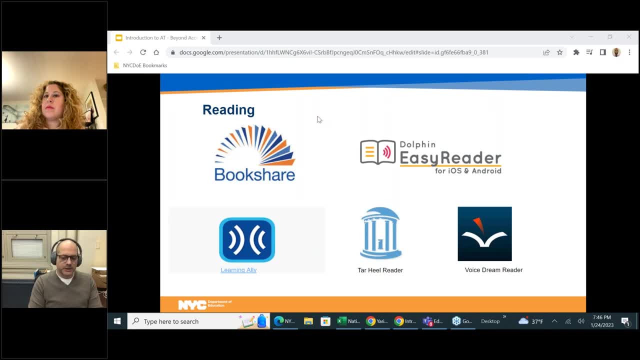 size the font, high contrast color schemes for maybe those students with visual issues: line spacing. Another big one is: if you're listening to audiobooks and it's speaking too fast, you're able to slow that down. Tar Heel Reader- we're mentioning this. 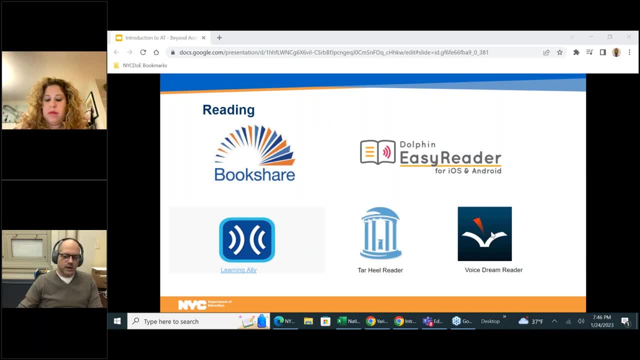 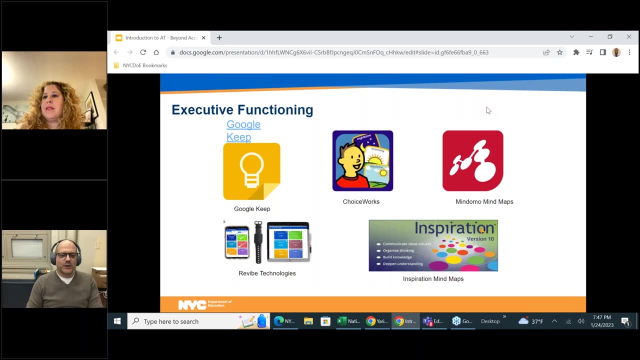 because this is a free and accessible resource and they can use it to open up source content. They do have a collection of accessible books on a wide range of topics. Next slide, please: Math, my favorite subject. So these are some of our most recommended AT tools. 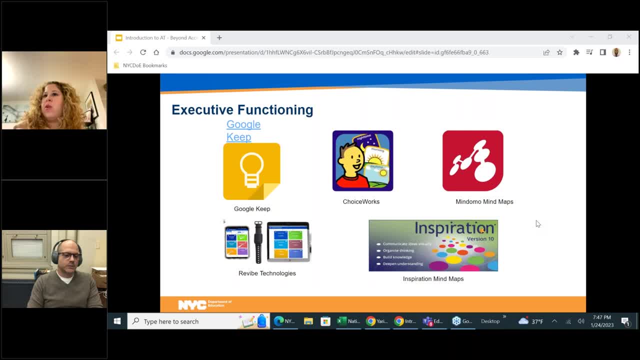 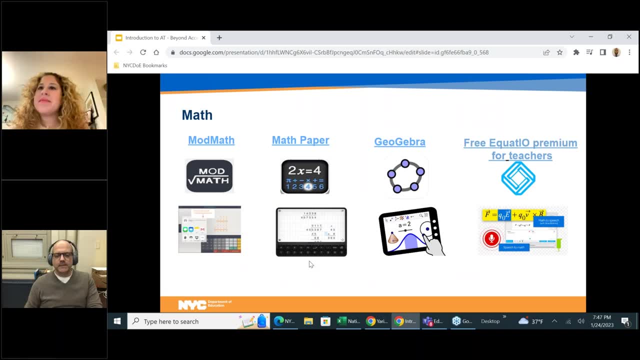 to support students who may struggle with math. Andre, can you go back one? I'm sorry we're on. Oh sorry, OK, math, Thank you, thank you. thank you, math. We want to note that most of these tools 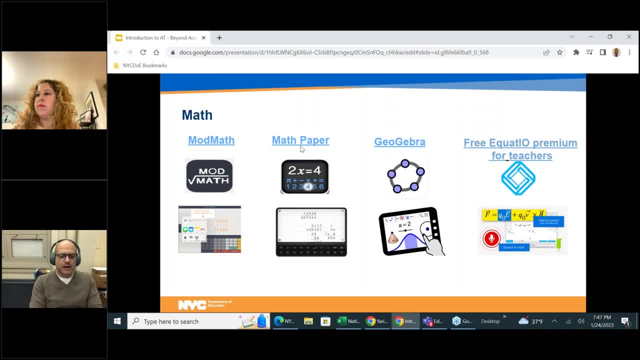 with the exception of GeoGebra- act more as an organizational tool and do not assist students with computation or providing students with answers. We get asked that question by parents all the time. We want to make sure that their children and their students are able to work through some of these math problems. 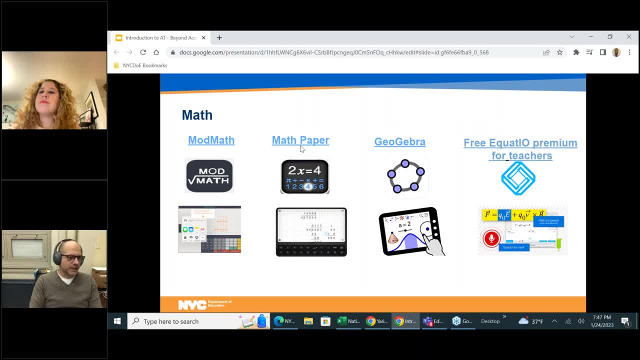 And we don't want to be provided. We want to be providing them solutions that's going to give them the answer. that kind of defeats the purpose. right, We do want to highlight ModMath because it's a free and it's a unique tool. 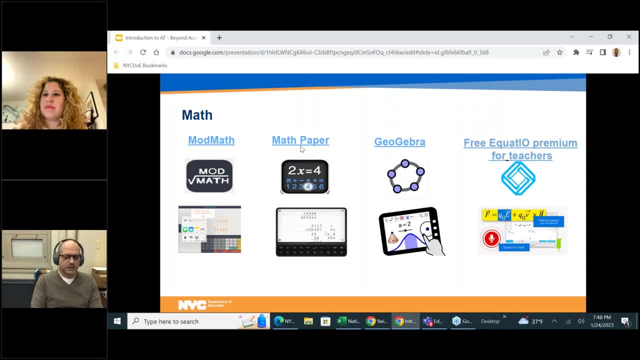 It was created by two parents that have a child with dyslexia and dysgraphia. It offers kind of a streamlined multi-sensory approach for kids with messy handwriting and those that struggle again with lining up problems. EquatIO, the one on the right. 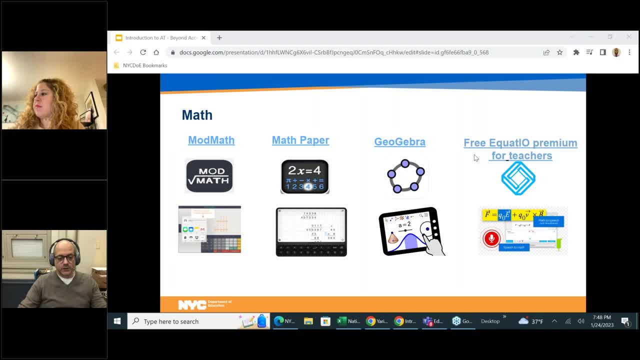 It is a premium product for us when we recommend EquatIO for students, and it's one of our most recommended and in-depth math AT supports. Some of the features include the ability to handwrite and then transfer that handwriting into text, so then students are able to listen to that information. 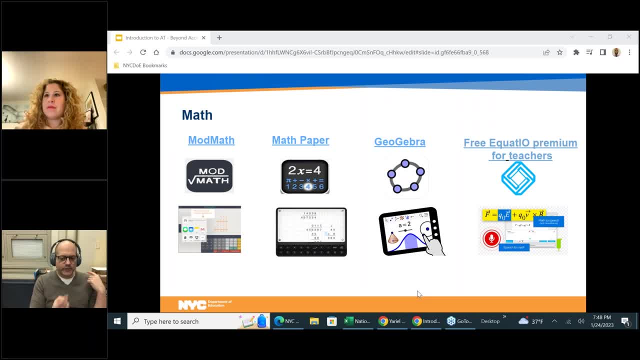 as well as use speech input or speak into the program so that you actually see the text come out On the screen. Parents, please spread the word about EquatIO because, although it's a premium product for us, teachers can access this resource for free. 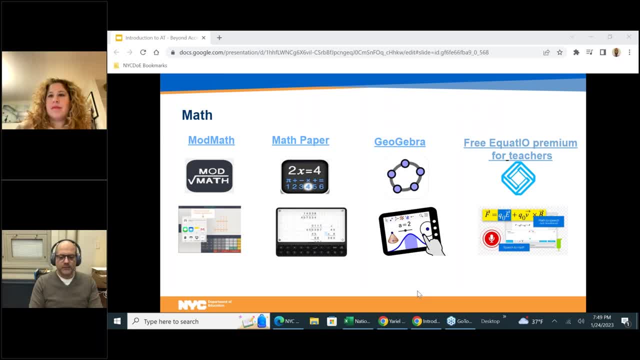 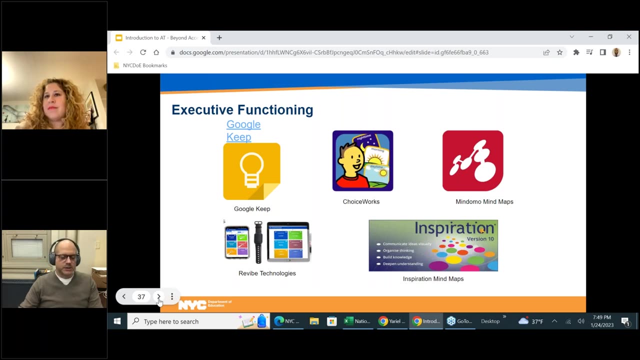 and incorporate in their classroom to support students from, like, an instructional technology perspective, again helping all students. Next slide, please, And we are at executive, Executive functioning, which, again in our minds, we think organizational skills. These skills that allow students to plan, stay focused. 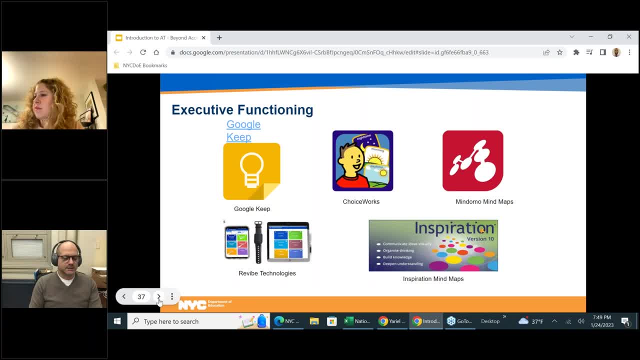 follow directions, stay in control and follow through on tasks. A few of the tools that we recommend: we highly recommend Google Keep. It's one of our most recommended free tools to support organization and it allows users to record plain text notes and organize. 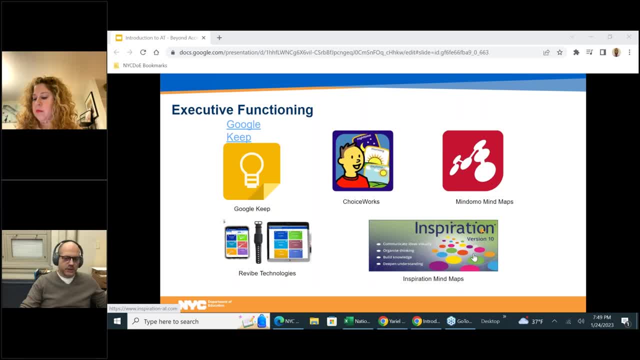 edit or share them with others using a suite of collaboration tools: Free resource, Google Keep, Mindomo and Inspiration Mind Maps. these are two of our most recommended organizational mapping software applications: Revive. I'm going to turn this over to Lindsay. 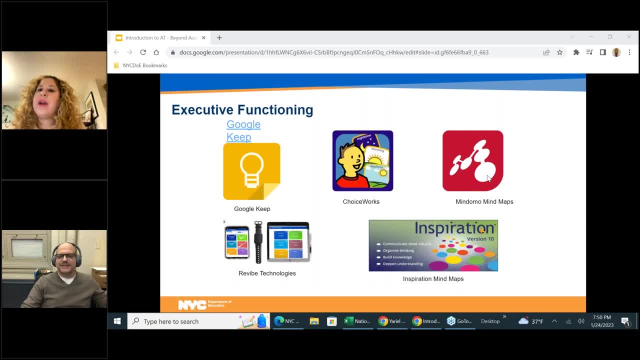 because I think you know a little bit more about Revive than I do. LINDSAY GOLDBERG- OK, So Revive is? it looks like a watch. It's used for students who have ADHD Attention Deficit. 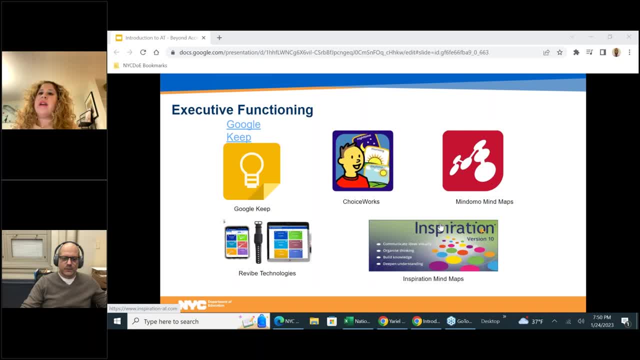 Hyperactivity Disorder or ADD, And it pairs with a companion, an app companion, And, instead of the teacher or an adult constantly tapping on the student's shoulder to remind them to stay on task, it has different vibrations that it. it vibrates at different frequencies. 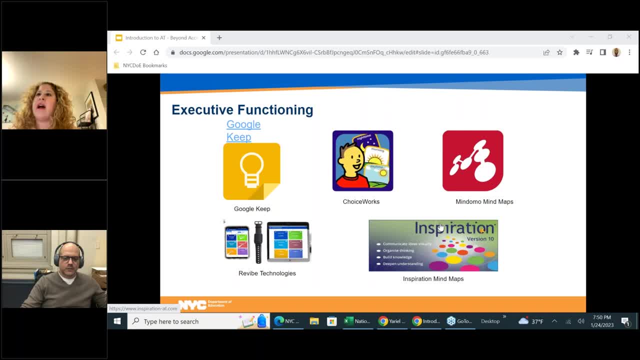 And the student can self-regulate whether they're paying attention or not. And why it's unique is because it will vibrate in different frequencies, so the student can't get used to it and just shrug it off. So it's a great tool. 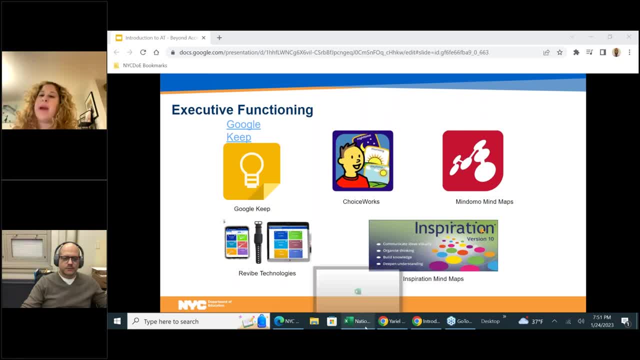 It gives you a lot of data to see if your student's paying attention And there's homework reminders. stay on task reminders And you can schedule different frequencies at different times based on student need. LINDSAY GOLDBERG- OK. 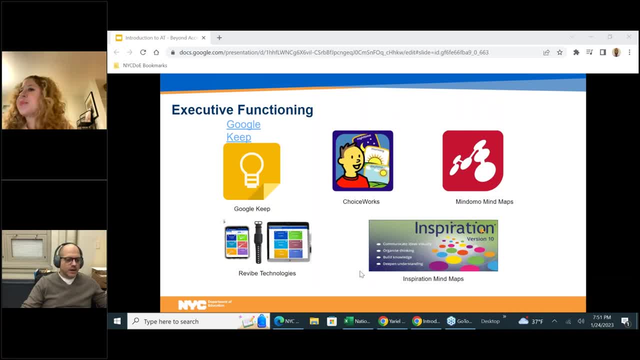 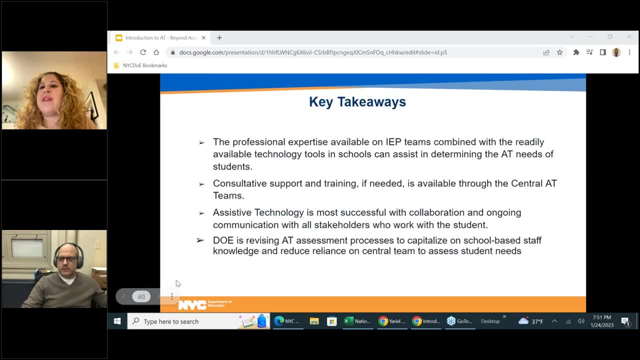 It's such a fascinating product, Lindsay. Lindsay, now I'm going to turn it over to you again because we're going to be discussing AAC right. LINDSAY GOLDBERG- Yeah, OK, so can we go back to the slide before? 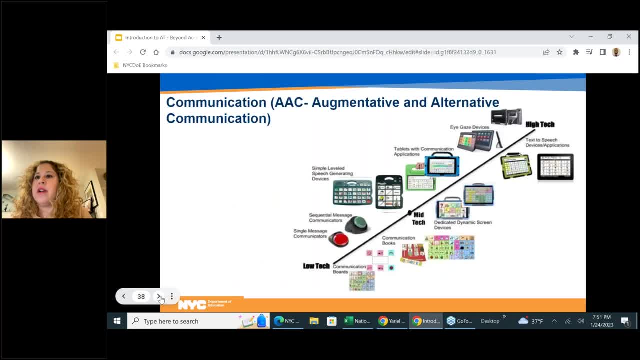 Yep, So we're going to talk about communication, alternative and augmentative communication. So this is used if a student is non-speaking or has limited verbal ability, or they may have an articulation disorder. LINDSAY GOLDBERG- Oh yeah. 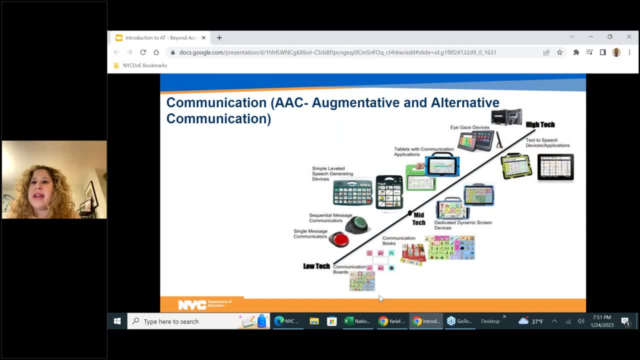 So if you have a student who's not speaking and they're trying to speak, you can click on the AAC button and you can select that, And then you're going to go to AAC And you can select the AAC button and you're going to select the AAC button. 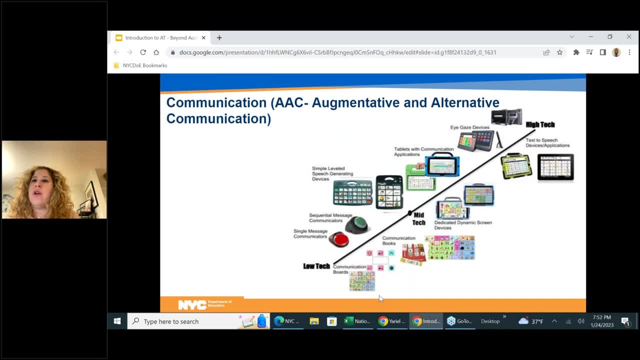 And then you're going to select the AAC button, see if you can see the red and green button. and it can be a student just touching a simple message: Yes, no, my turn. It can be a communication papered base board or a picture exchange communication book. 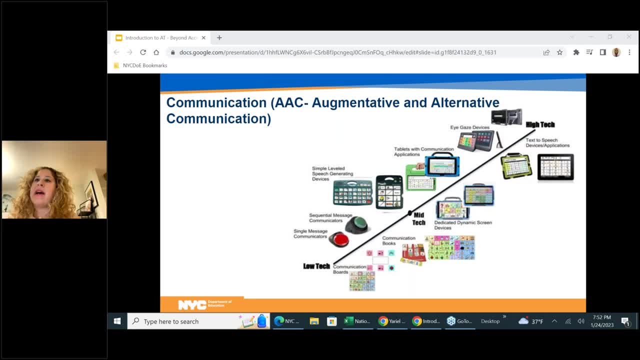 where there's various symbols on a book and the student can point to or exchange a symbol And as you move up it's up to you to choose which one you want to use. LINDSAY GOLDBERG- OK. 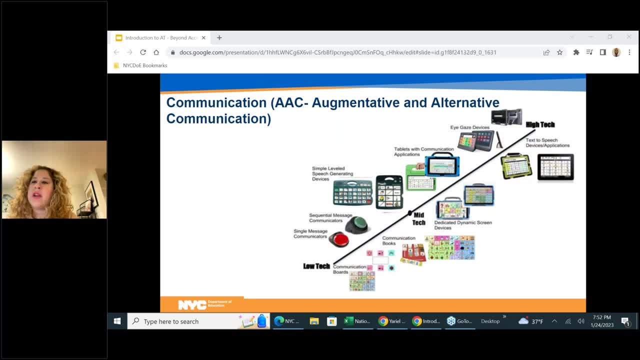 OK, you move up in the continuum. you have simple leveled speech generating devices where the student presses the button and there's voice output to say, maybe I want to read a book. Then we move up the continuum to where we have dynamic display speech generating devices. 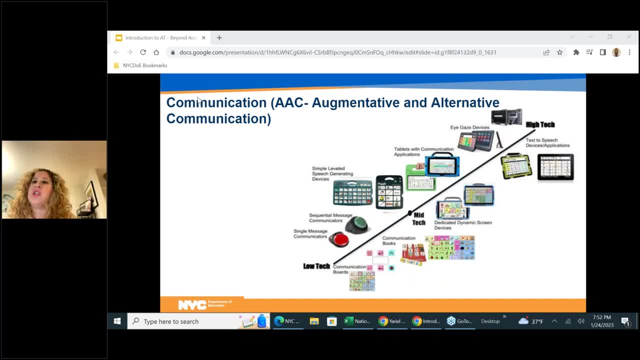 which maybe can be an iPad with various communication applications, all the way up to the continuum, where you may have a device that you can activate using your eyes. So there may be a student that doesn't have the ability to move their hands or to speak verbally or to activate. 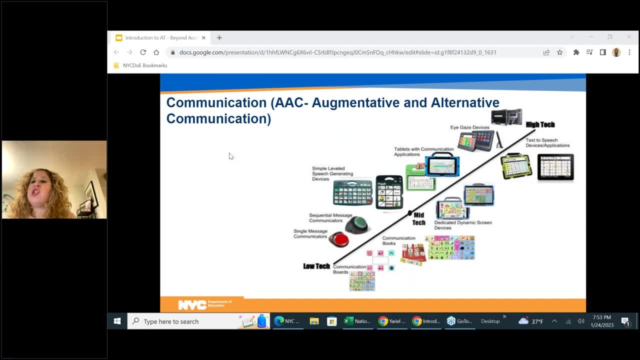 a switch and they can activate what they want to say just by using their eyes. So there's a variety of tools that we can use to determine which assistive technology is appropriate for a student that is struggling with communication and needs to access their curriculum. 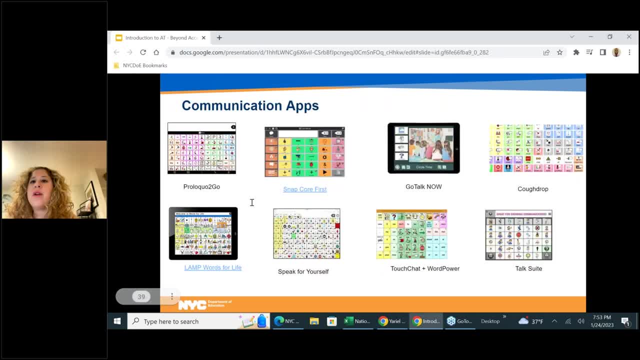 Next slide. Here are some examples of these are iOS apps, some of the communication apps that we use. As you can see, there's different levels and layouts and they're organized differently. So when we go in and we look at your student or your son or daughter, we try to determine or help. 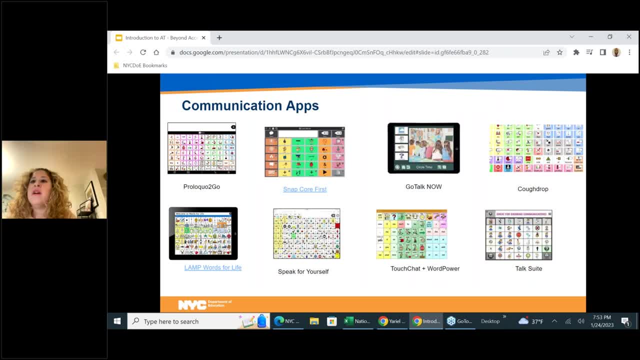 the school-based team determine which would be the best application for their student. One of these apps is the CoughDrop app. Most of them are iOS based, with the exception of CoughDrop, which is on the upper right, and CoughDrop is the only communication application that will work on an. 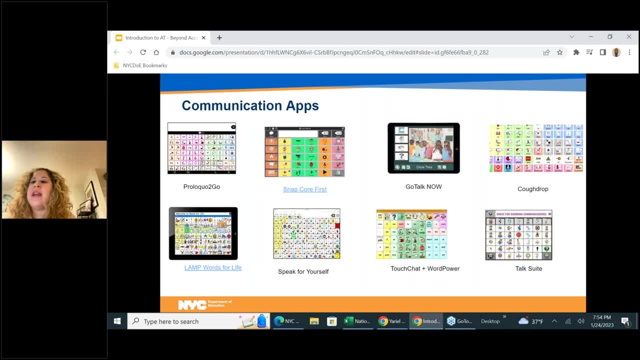 Apple device, a computer, a PC computer, a Chromebook and an Android. So it works through it's web based, So it will work on any platform, But all the other applications here are only available on an iPad. Next slide: 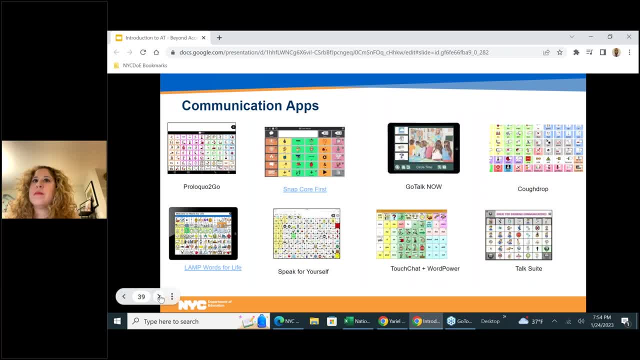 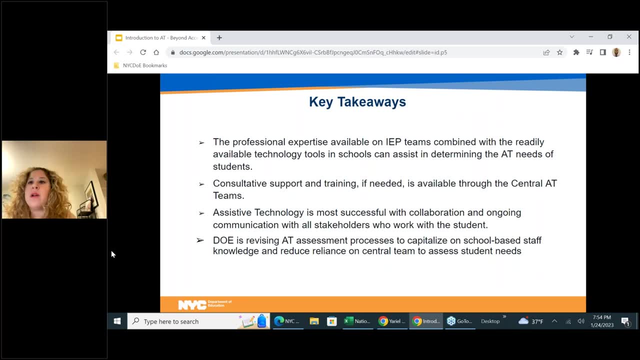 Next slide. Next slide, please. So we want to talk about some of the key takeaways. The professional expertise available on IEP teams, combined with readily available technology tools in our schools already can insist in determining the AT needs of students. So consultative support and training if needed. 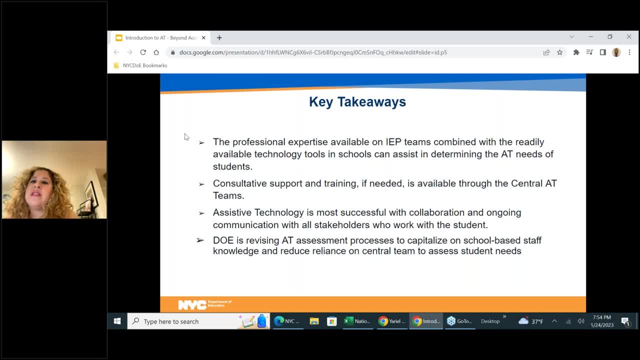 is available through the central AT teams And assistive technology is most successful with collaboration and ongoing communication with all stakeholders who work with the student, And the family is a very important stakeholder And, as we touched upon earlier, that the Department of Education. 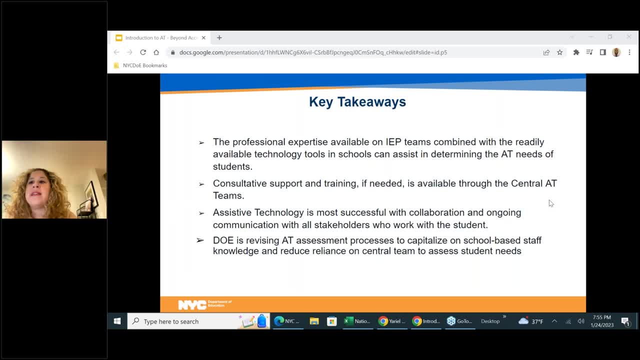 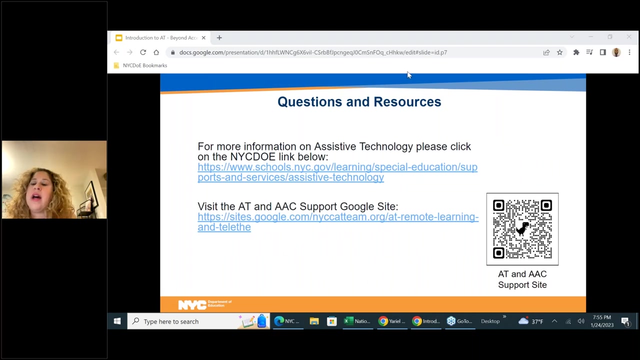 is revising AT assessment processes to capitalize that school-based staff, or you know, have the knowledge and reduce the reliance of coming to the central team to assess students' needs. Next slide, please. So here's some additional resources So you can click on. well, you can't click. 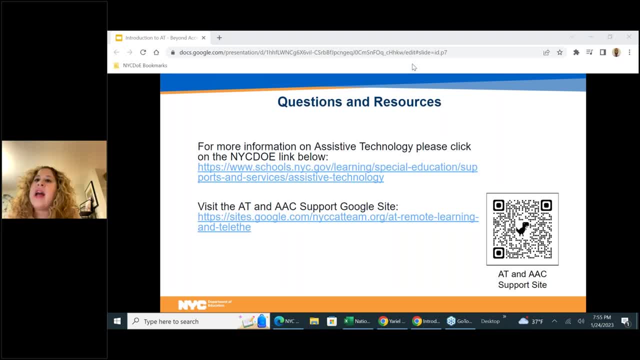 but you can Google the assistive technology, New York City, DOE and you'll come with the link above. But if you have a phone or iPad at home, if you have an iPhone, you can open up your camera and see where that little dinosaur is. 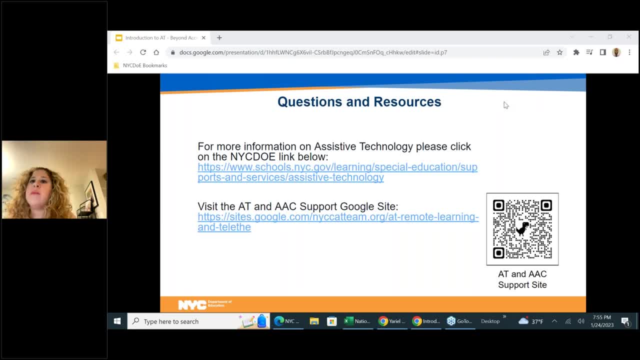 You can put your camera up to the QR code and you will be able to see our AT and AAC support Google site. If you have an Android and have a QR code reader, the same thing, or an iPad. If not, you can quickly snap a picture of the Google site. 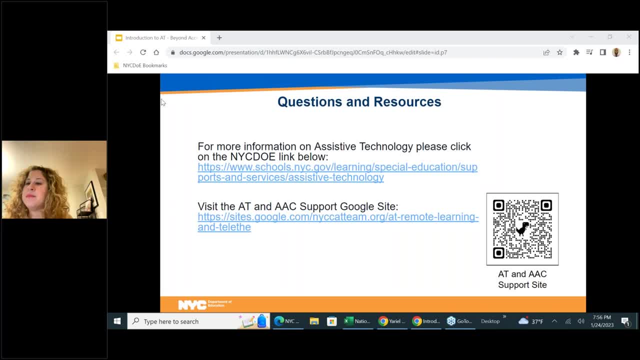 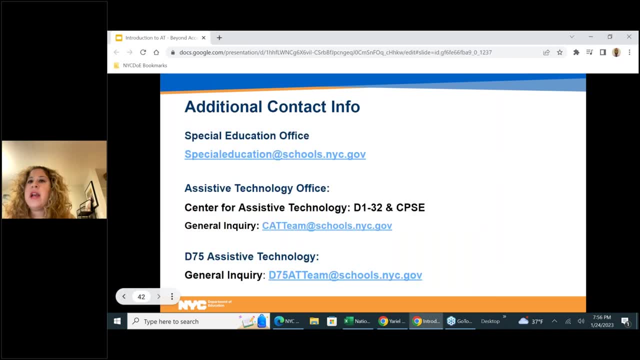 and you can type it into your browser if you don't have a QR reader. Next slide. If you have additional questions, you can always contact the Special Education Office at specialeducationatschoolsnycgov, The Assistive Technology Office for the Center. 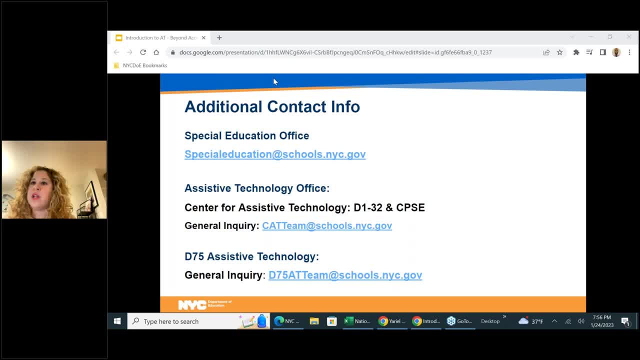 for Assistive Technology. again, we serve as districts 1 through 32.. And CPSC and CSE students, you can email us at catteamatschoolsnycgov And for District 75, you can email them at D7580. 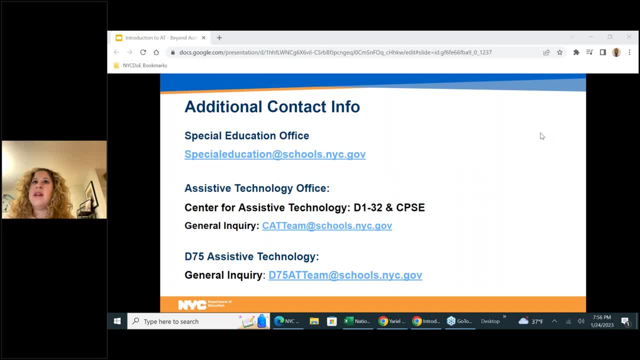 Thank you And if you have any questions, you can reach out to us at cptteamatschoolsnycgov And we now have opportunity for if there's questions, Suzanne and Andre. Hey, Lindsay, this is Suzanne. Can you just mention Saturday Academy? 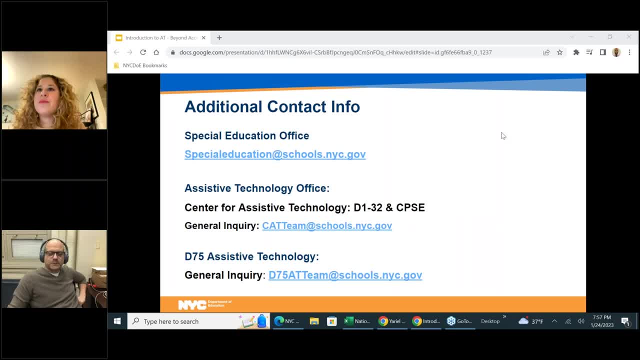 Yes, And folks can use the CAT Team email and then we can send them the survey. Yes, OK, great, Thank you. So there's a fabulous new initiative that the Special Education Office has. It's called the Saturday Academy. So if you have students that have IEP-mandated or 504-mandated, 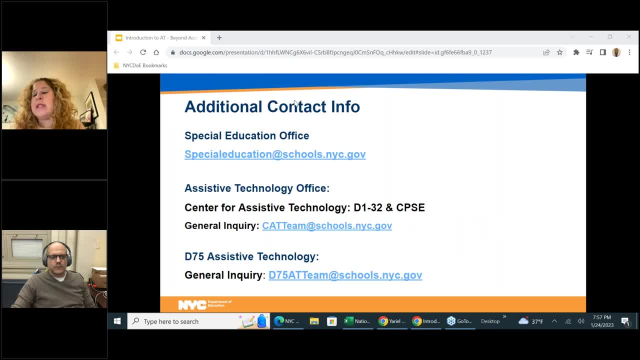 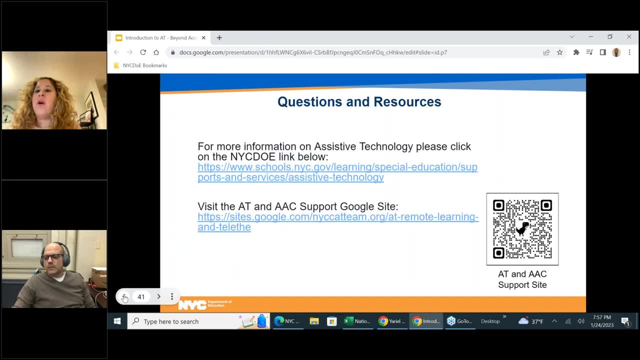 assistive technology and you want training or implementation support or you have questions on how to utilize whatever assistive technology your child has at home, you can email us at catteamsatschoolsnycgov And we will send you the link where. 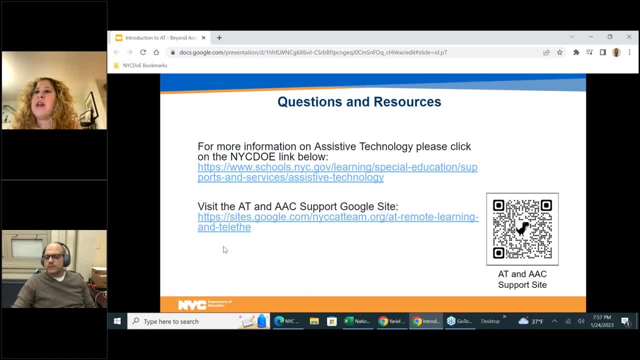 you can book an appointment and come to one of our locations. They're in the five boroughs. There's two locations in each borough And we're available, from 830 to 230, to assist you with your assistive technology needs, And we'd love to see you. 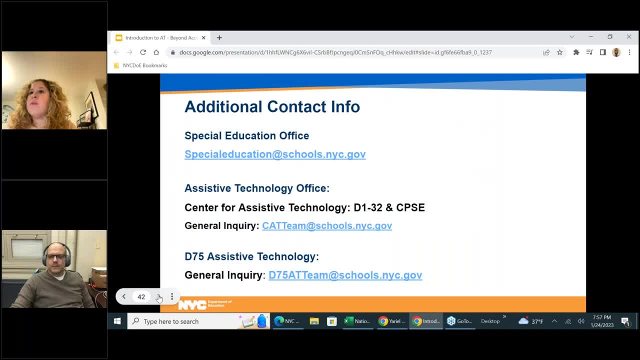 And there's opportunities for you as a family, as a parent, So you can bring your child, You can come alone And you can see other assistive technologies. So maybe you have a communication system and you need to figure out how to address literacy or writing. 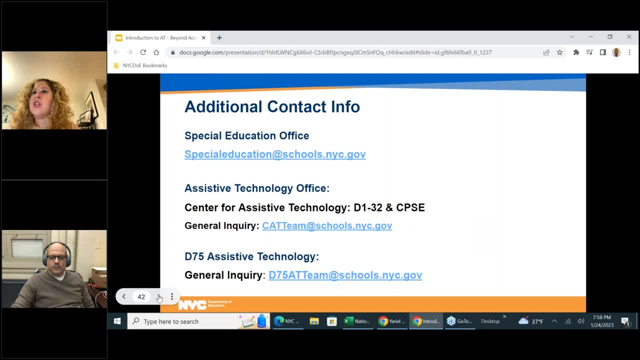 with your student And you feel that they need additional assistive technology. We can show you some of the things that are available for your student, Lindsay. I just want to add that it's just an amazing opportunity for parents to engage with some of these resources. 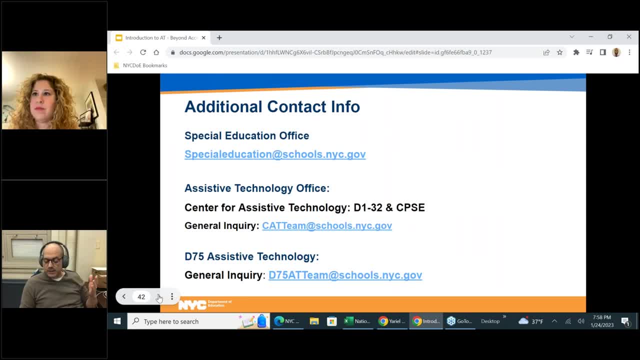 I mean, even if you don't have a student with assistive technology and you think, hey, maybe some of these resources can benefit my student, we have amazing providers that are available on that Saturday Academy and can walk you through Some of the resources that we share today. 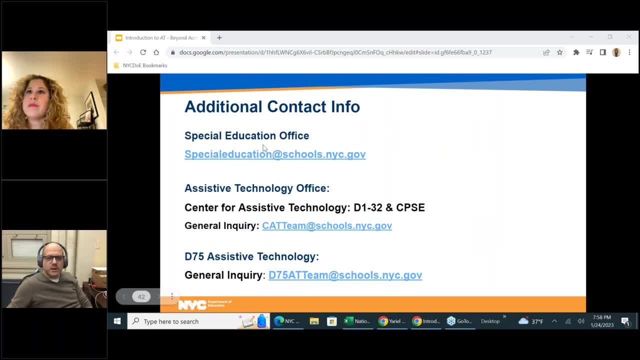 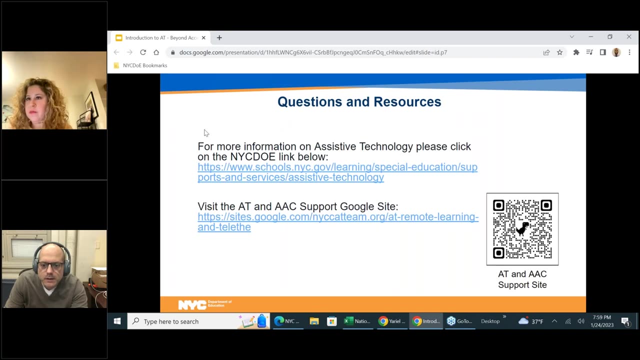 It looks like we do have some questions. Andre and Suzanne, do you want to? If you see the question about LAMP, that might be a good place to start. If you see that question, Where is the LAMP one? Do you see it, Lindsay? 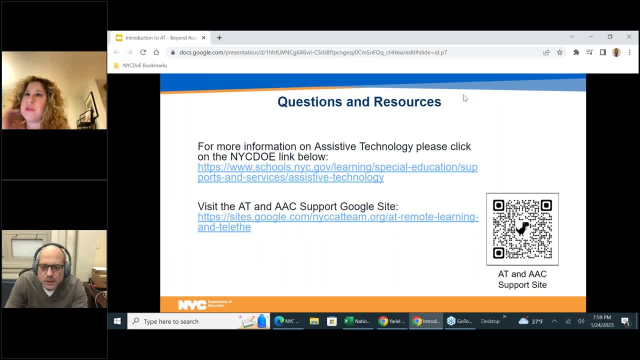 No, I don't have access to the questions, So if you guys want to screenshot them and text them to me, I can answer them. So let me let folks know. So I apologize, We're just showing the QR code because that was a request again. 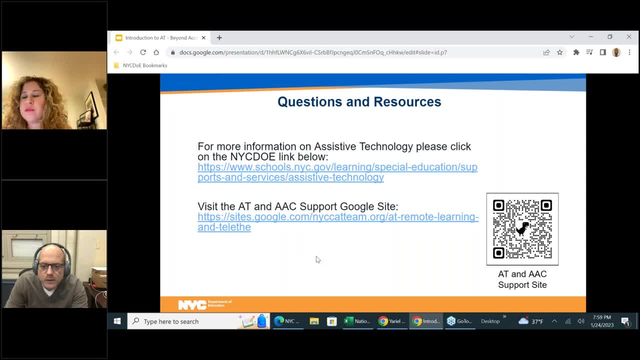 So we're showing that again. There will be a copy of this recording sent out to everyone within 24 hours after the conclusion of our session this evening. We will also add to that email, which has the link to this recording, the URLs which are currently on the screen. 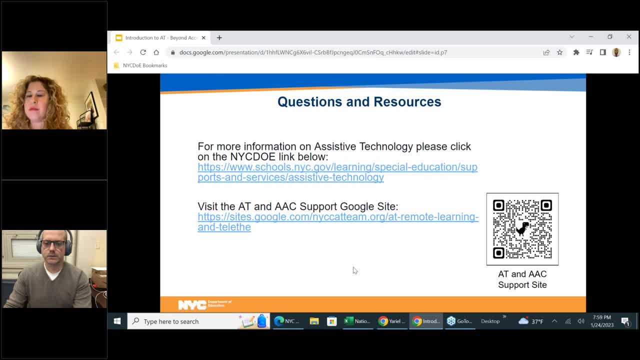 So we will provide the links to the URLs that are currently on the screen in that same email that you will get 24 hours after our conclusion this evening, as well as the link to the recording so that you can add for your own records. We will not be providing the slide deck. 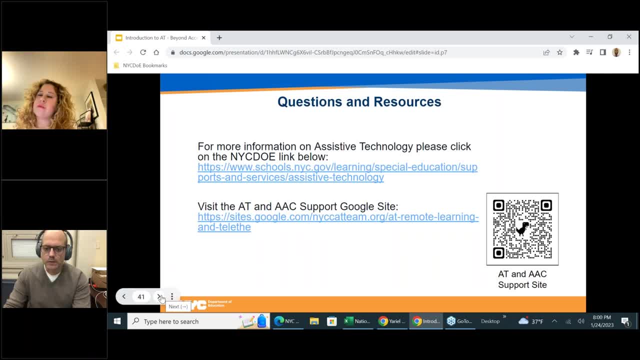 but again, you will have access to this recording, So I'll leave the QR code open up for another second or two And then, just for those who had questions or concerns around the email addresses, we'll put that back up currently for folks to see. 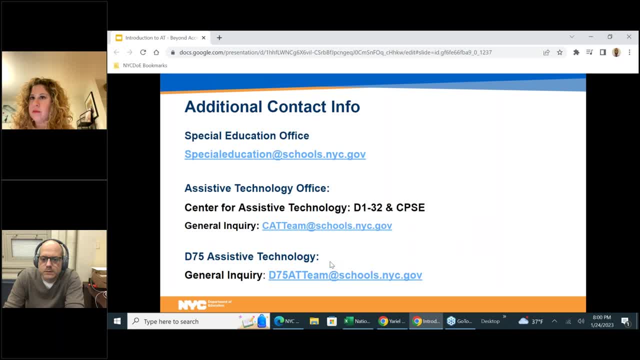 and record that for your own records. We are exactly at 8 o'clock, so we will take two to three more questions And we do have access to the questions that were not answered in the chat and we will try to get back to you subsequently after. 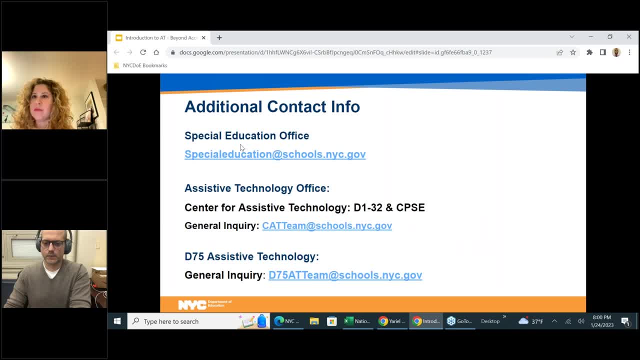 So we will get to as many questions as we can this evening, both over the mic and in the chat And directly to you in the chat over the next two to three minutes that we have. So we'll go another two to three minutes. 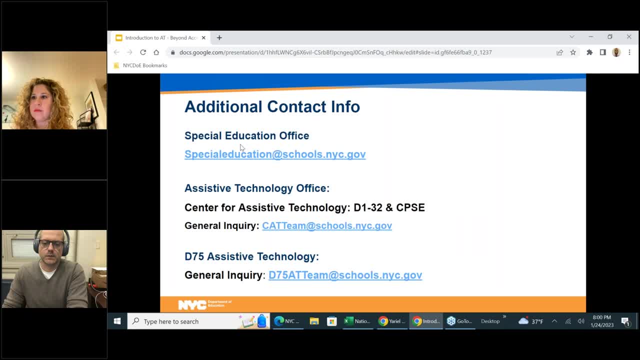 But we apologize for the sake of time, we won't be able to go through every single one. David, were you able to find that lamb question? I haven't. I'm just going from down and up. Yeah, Someone said thank you. 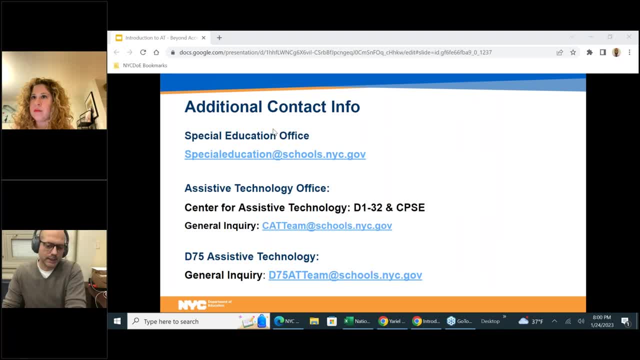 Is this a weekly or monthly program, Or is this a one-time thing? The Beyond Access series is a Monthly program. Monthly program: Saturday Academy. the question is about Saturday Academy. That is, to my knowledge, Every week through June 17th, I believe. 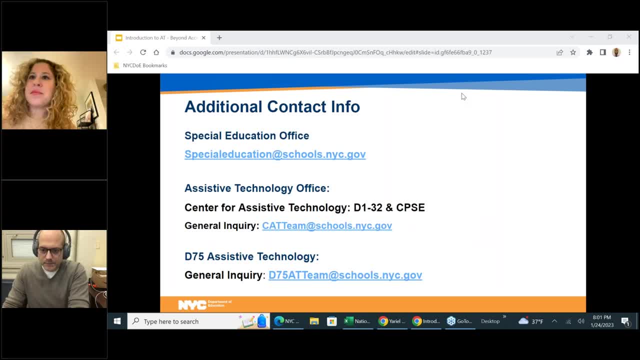 That's correct Question from Jennifer Fishbein. Can you confirm which team supports regular public school students? That is the Central Assistive Technology team. But families and folks don't worry about that If you send the email to one group and it belongs to another. 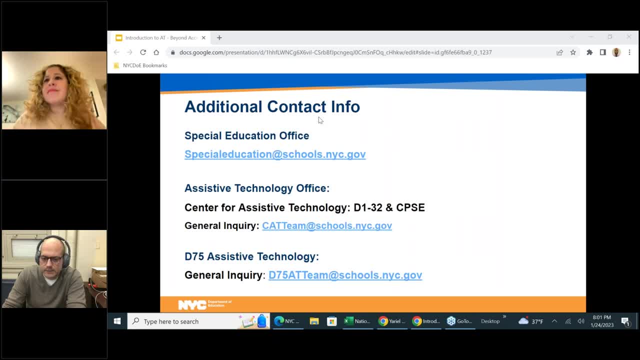 They will talk to each other. Yeah, These teams work seamlessly together And no issue there. Regarding the softwares that are not free, does the school DOE provide those software programs? Yes, Yes, We do. You do not have to worry about cost. 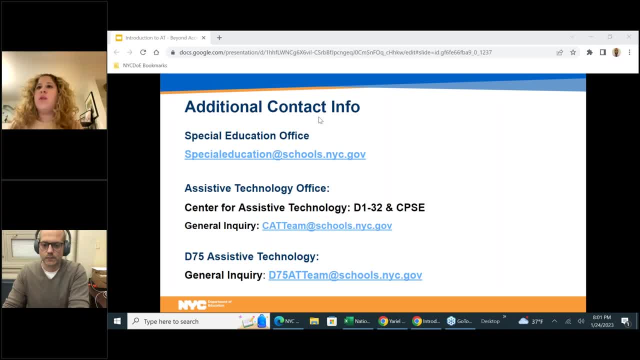 If your student is eligible for Assistive Technology, the central teams will take care of the cost of the product. Next question from Ms Castro. Yes, I asked about support outside of Assistive Technology, Like middle high school students who are grades behind. 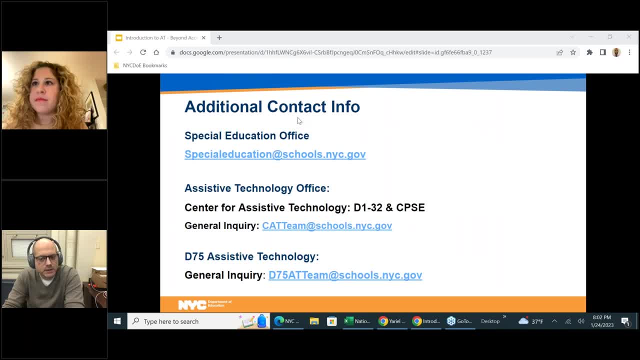 and reading aren't currently receiving AT versus. So this is a great question And what we would ask is that again, you'd go back to your IEP team And consider the needs of have them consider the needs of your child. 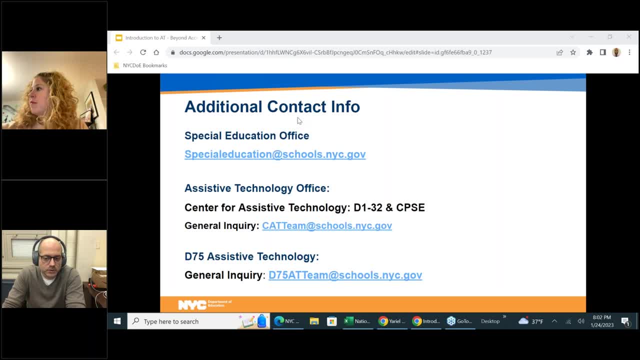 Perhaps this particular student, upon consideration, may benefit. There's a need for Assistive Technology to support their reading and writing. Let them know that you had this presentation And if they have any questions about Assistive Technology, we can certainly support you and the school team. 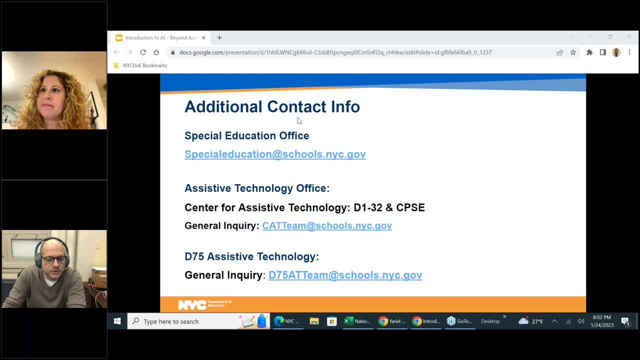 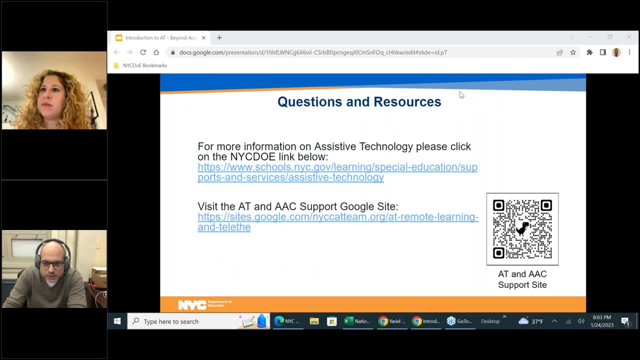 Can I get the QR code to work? I think that's an Andre question. The IEP agrees to using AT for students. David, can you speak to if a parent has a child who has hearing delays or hearing deficits, and who would they contact? 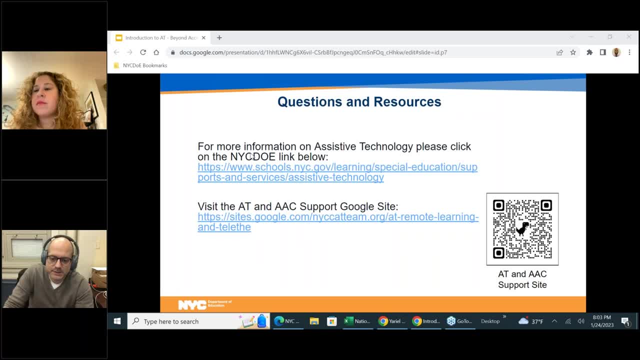 You know what I'm just going to say. contact me at D75 AT Team And I will assist in that process here in the District 75 office. Indeed And Lindsey. this question has come up a few times in the chat. I've answered a few. 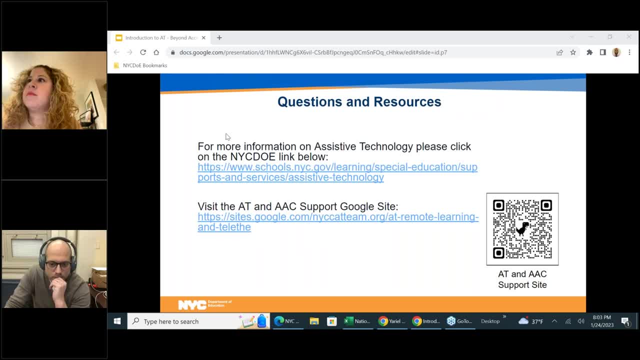 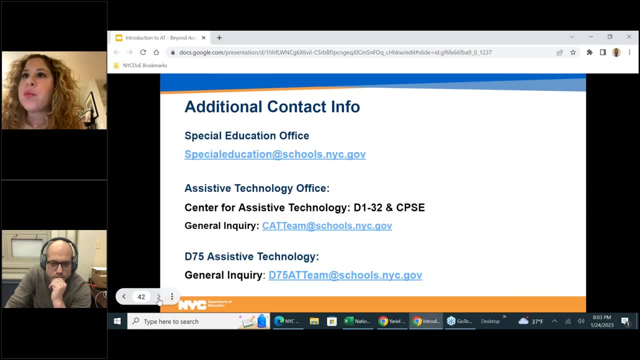 but it's a really important question: What if my child had AT but it was broken? Okay, How does the person get a new device for their child? So if it's broken, you can also email CAT Team And we have tech support. 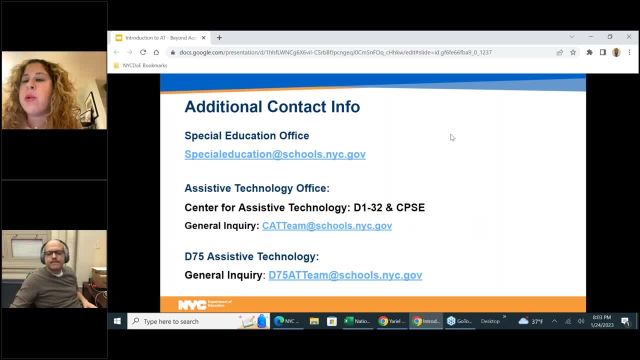 So we can send you guys the link for tech support And you can fill out a ticket And if we can fix it, we will fix it, If not, we will replace it. So you can email catteamatschoolsnycgov. 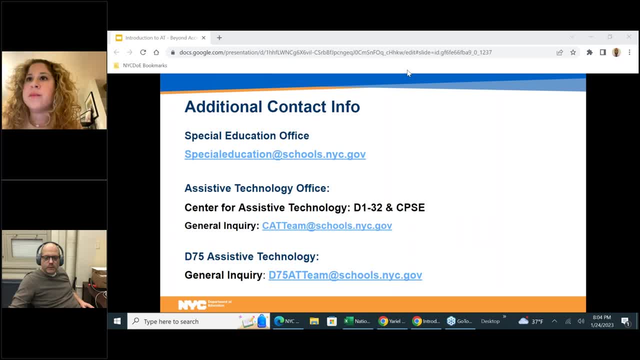 And we will send you the link to our tech support. Great, And there was one question, Lindsey, where you were talking about a specific device. Lindsey, you were, I'm sorry, a specific program just before. And there's a question if it requires Wi-Fi. 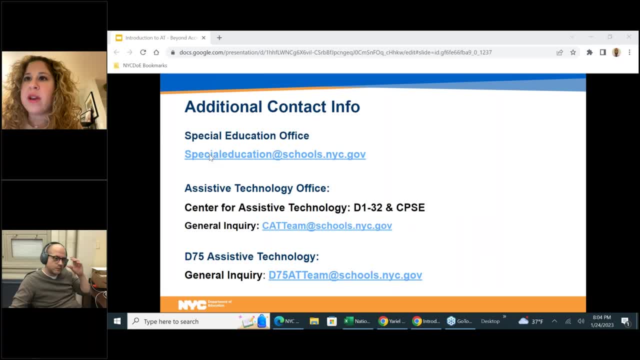 For that program. Are you talking about the Revive Watch? I think so. Reema is asking Reema if you want to tell us specifically. But I think so, Lindsey. Okay, So the Revive Watch. you don't need Wi-Fi for the actual watch. 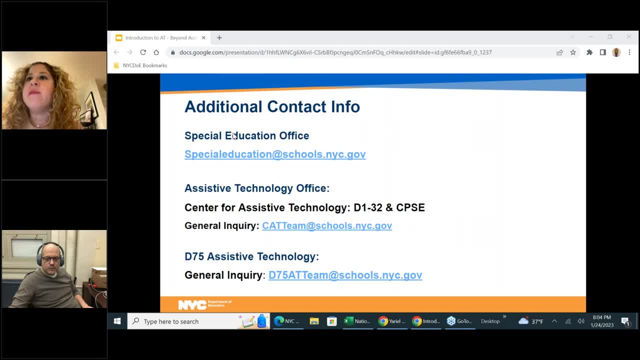 You do need Wi-Fi. The companion app lives with the teacher, So and the parent has access to that also. So if you want the data from the watch, you need Wi-Fi, But the actual watch you do not. the student does not need Wi-Fi to use the watch. 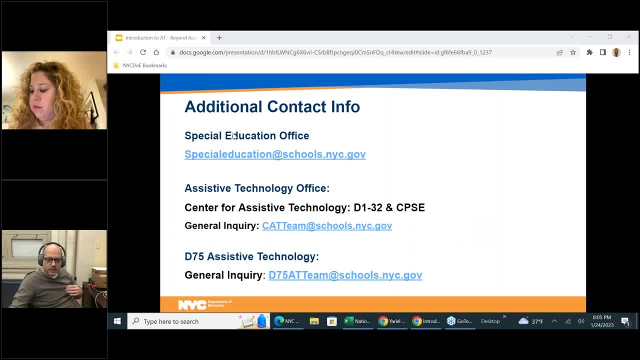 This is a great question by Ms Kasata. How long does it take, once the IEP team agrees to using AT, for the student to start receiving AT As soon as it's on the IEP and the student has that equipment in their possession? 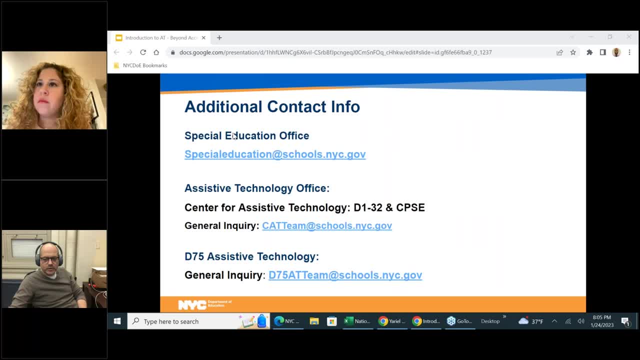 the IEP team has that equipment in the possession and the software programs. It's a go. The student can start receiving the assistive technology that they need. Reema asked a question. Ms Esquiendo, maybe cough drop, I think. maybe that's the one. 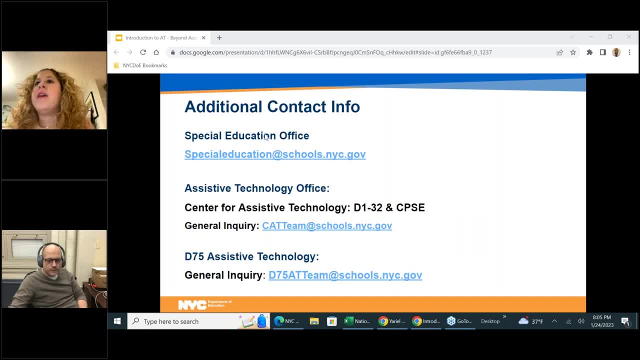 Oh, cough drop. Okay, It was about cough drop. So, Reema, cough drop is an AAC app. It is available on any platform. There is a 60-day free trial. So if you Google cough drop AAC and you wanted your school team to try it with your 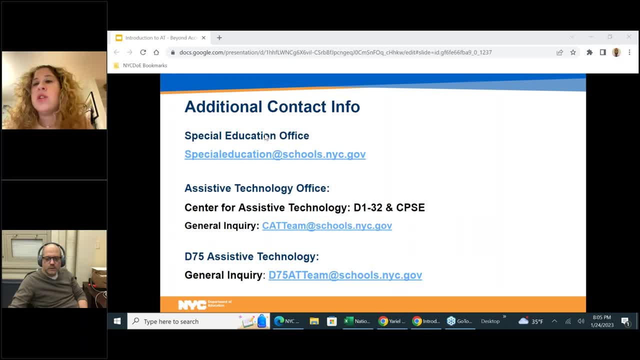 you know your child. you can do that, And it's available on a Chromebook, a PC. you know an iPad, an Android device. When we give it out, when it's recommended for assistive technology, we will recommend it on an iPad. 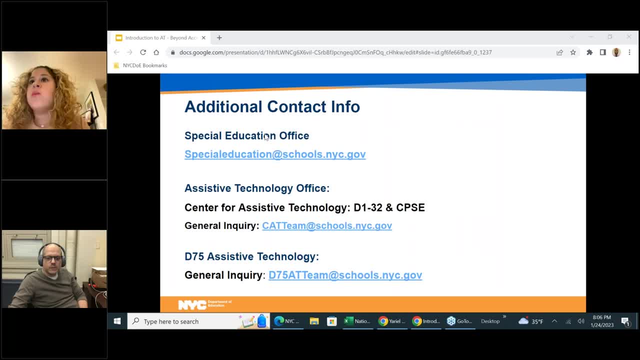 because that's the way that the student can access it for their curriculum and it's portable. But the advantage of it being available on other devices is that it's available on a computer. So if you have a computer, you know if you have a laptop. 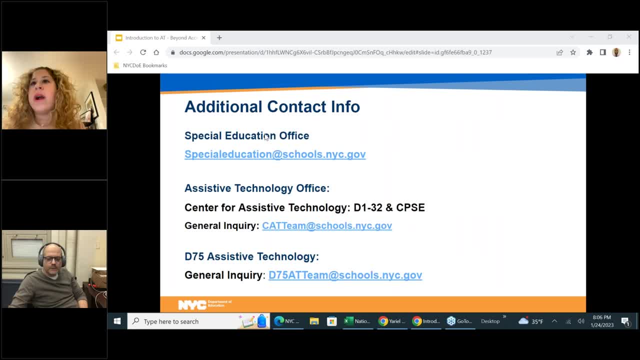 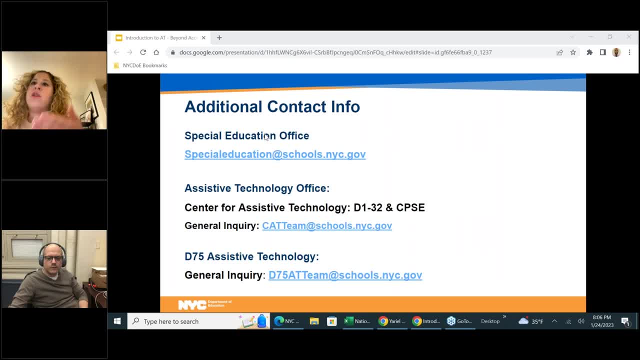 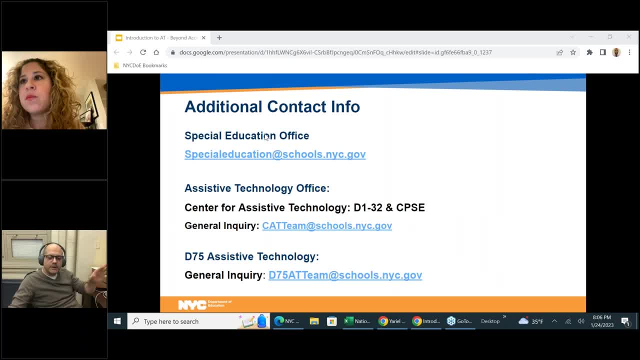 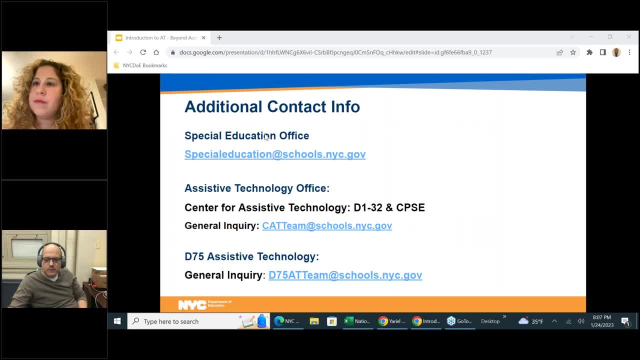 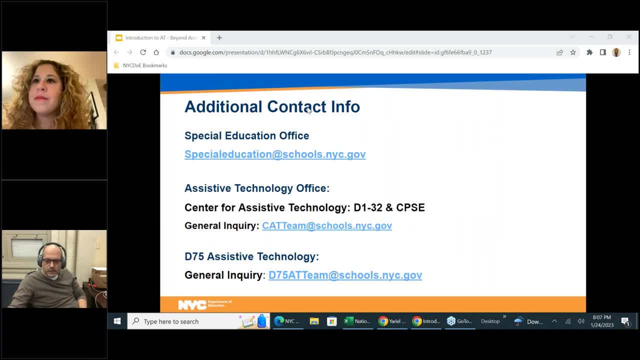 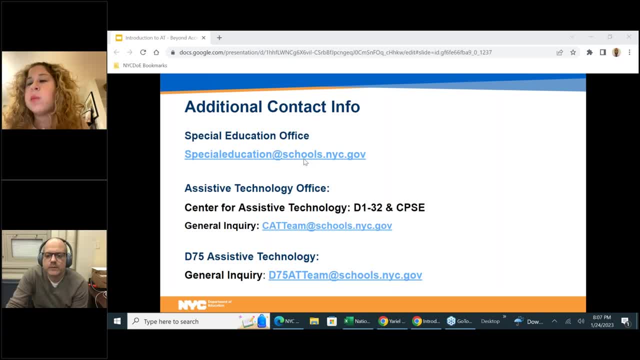 you know, please go to your IEP team if you would like to explore assistive technology for your child with autism. question: okay, which is important, because does the communication app, like lamp, get updated? yeah, and this particular parent, her son's iPad with lamp keeps crashing. so that would be that. 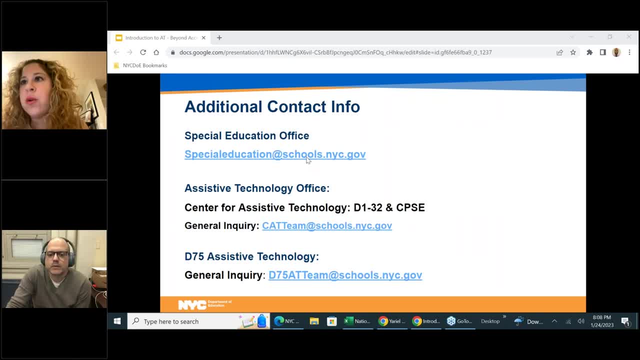 was so again, if there's a tech issue, you can either email cat team at schools, NYC, dot-gov or the d75 team, depending where your child is, and we will offer you tech support, and if the iPad is, you know, older and it cannot be supported anymore, 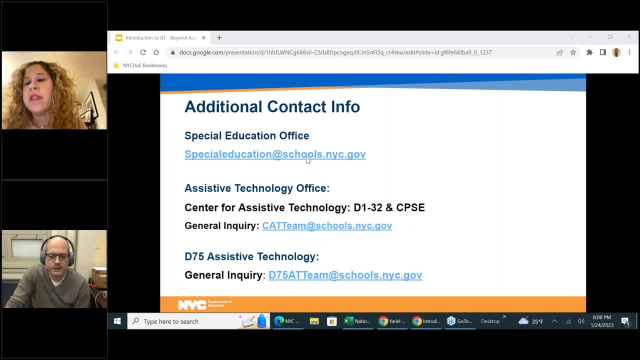 we will provide you with an updated iPad and with a lamp on a new iPad. that's right. it's important to note that we have the ability in the last number of years to remotely connect with these devices and if an update is required, usually they update automatically, but sometimes we need to push an update if 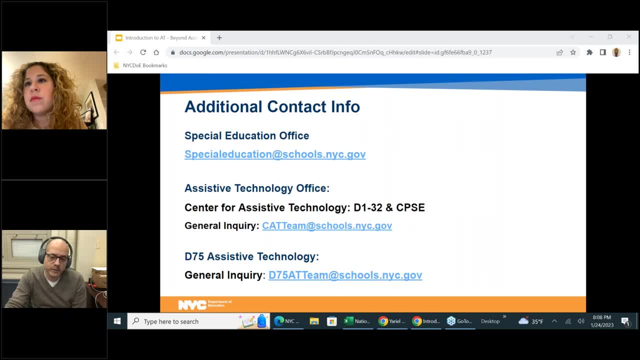 Lindsay, like your saying, if it's a bit older device and if it needs to be replaced, right, get it replaced. speak. should I bring my son's device? um? Salisha, please do bring your son's device. um, if it's a communication device, we we emphasize that that device should be with a student at all. 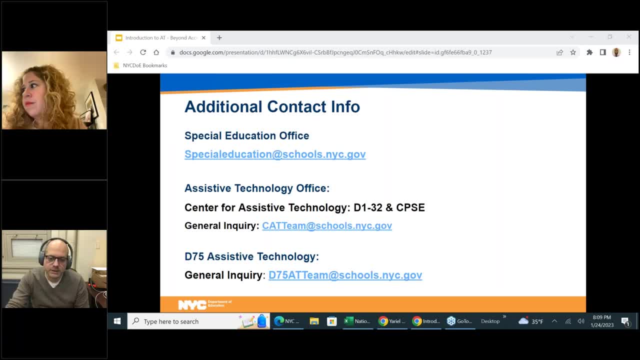 times, um, it's, it's a, it's a great experience. bring it to Saturday Academy, um, so that they can be incorporated into the routines. yeah, you can. actually. when we, if you email us, we can send you a booking and then you can book a specific time that works for you and your family to go. 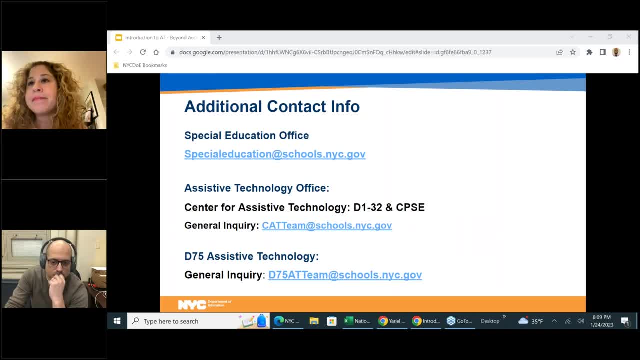 to a specific location to get support. um, it sounds like this is a uh from Miss Ellis. another Saturday Academy. if the child hasn't done testing yet, can they still go? they're waiting to be tested. is this Saturday Academy maybe? um, so, yes, in that case. David, you know we Saturday Academy is typically for students whose current IEP recommends AT, but 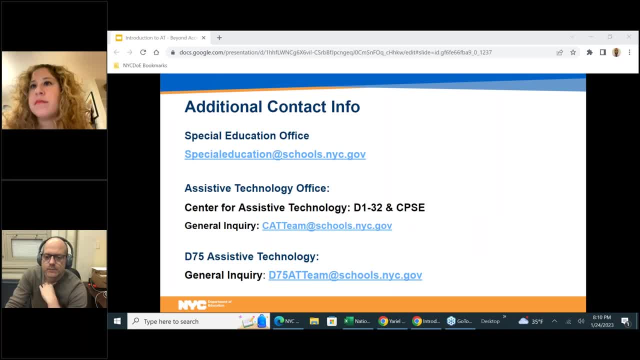 if a child is waiting, we could certainly provide some strategies and supports directly up to the um at Saturday. that would be cool, okay, thank you for that clarification, Suzanne. uh, one more time with QR code. sorry, I think that may be an Andre question. just keep the QR code slide. 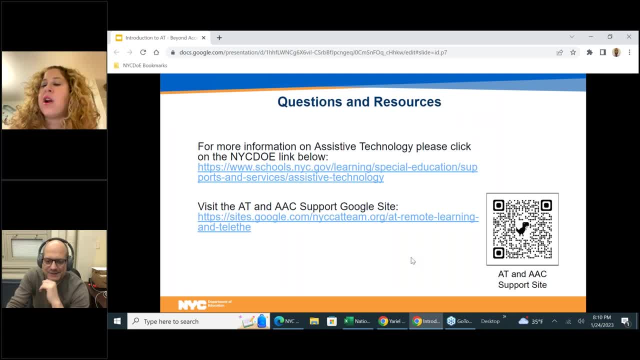 up. you can copy the Q, can use the QR code with your phone, but if you don't have that capability, you can take a picture of this slide with your phone and you can just type in the https. you know, sites, dot, googlecom, and that will also bring up this resource and it has a lot of information about 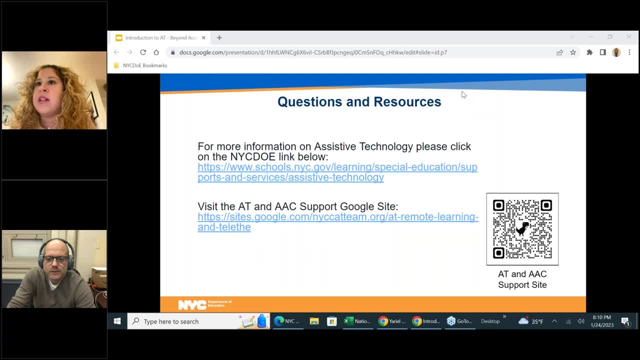 communication, writing, reading, math, executive functioning skills for parents and families. um, some go-to sheets, some implement implementation ideas. so we encourage you to do that for our students: implementation ideas. so we encourage you to visit it. yep, and we'll include the links in the follow-up. 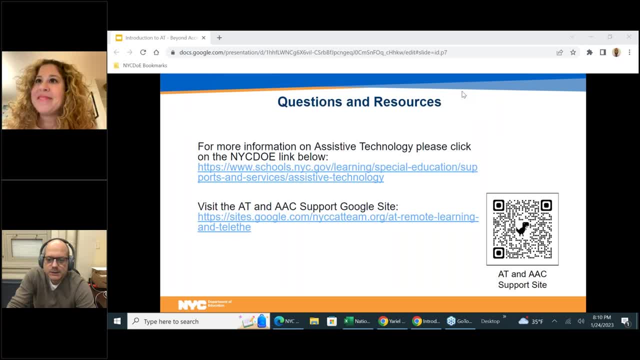 email that everyone will get. uh, 24 hours, 24 hours after our session, okay, and then you'll be able to click it when you get the email. so don't worry about our little dinosaur qr code. andre, do we have two more minutes to do a round robin with a question? yes, sir, yep, we can finish up two more. 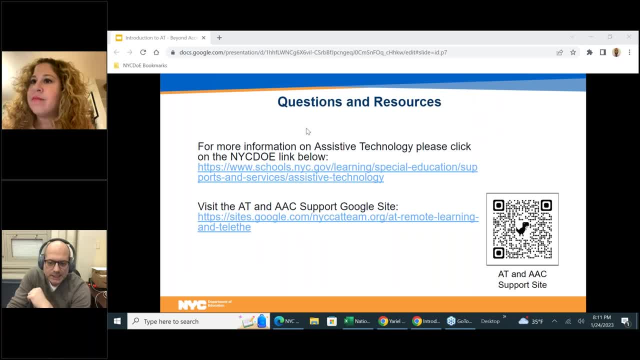 minutes. okay, uh, rima is you're asking about the last program on the program slide she just maybe mentioned, maybe four slides ago. can we communication? can you specify, rima, what is the apps for executive function on one of the slides? um, we mentioned our most recommended executive functioning, which is google keep. 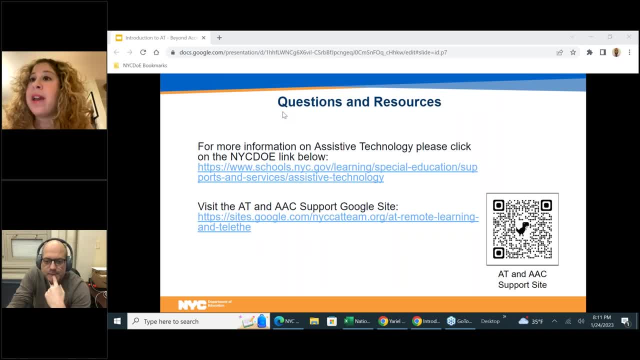 and that's available to all students because we have new york city, has a google domain, so that can be used, as you know, instructional technology, universal design for learning, or as an at tool. you gonna click on the leadership fee of the state and we definitely rally, encourage you to go to google keep. 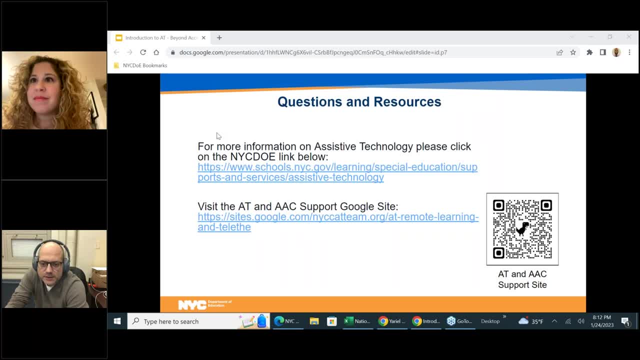 core advisors duzane. this is an amazing um. it's amazing feedback from miss flores. i attended the saturday academy on saturday and the staff were amazing at the dinsmore location. that's amazing, that's great. thank you. Yeah, Colleen, It's Colleen Yep, Go ahead. Center for Assistive Technology. We are districts one. 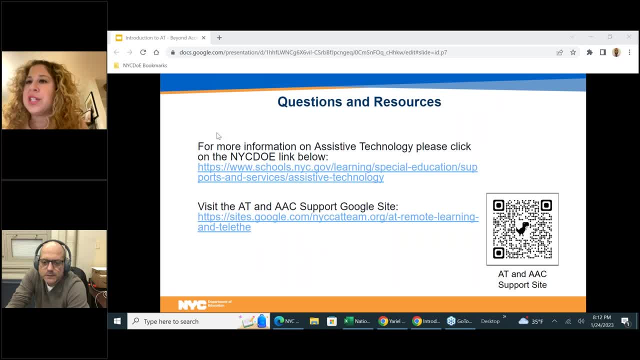 through 32.. So you can email us with any questions. But, as Suzanne said, Colleen, myself, as the directors we work closely hand in hand with Lindsay and all the rest of the supervisors, So if there's emails that go to either team, we always direct them to the right person. So don't. 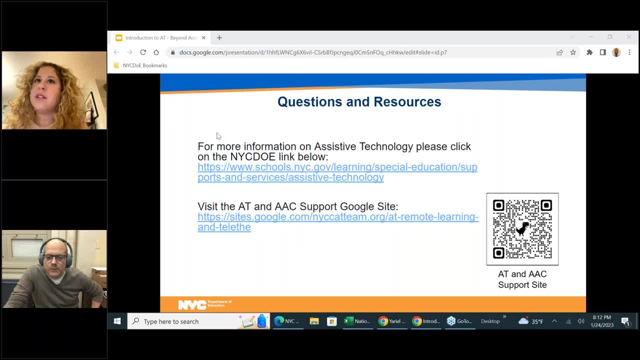 worry about whoever you email. We will make sure we answer your questions. The last program that works on all devices: Cough Drop, Cough Drop. Thank you, Natasha, And I think we answered the Wi-Fi connectivity. Is this being recorded? Yes, It'll be available within 24 hours, I believe. 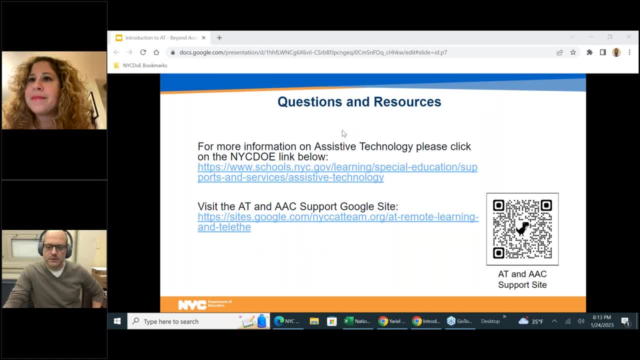 Andre said. That is correct, Lindsay, Thank you. You're welcome. I've done this before. This is a great question of a child already has an AT device but wants to add some of these apps. We would encourage you to speak to the IEV team. Remember what we mentioned during our presentation. 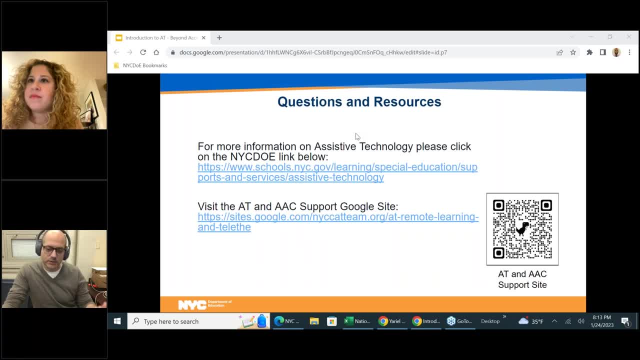 Assistive Technology is a process And the needs of the students will change And therefore, depending on their expectations, the team, including yourself and your child, may identify Other tools that are required, And you can certainly use us during a consult to assist in this process. 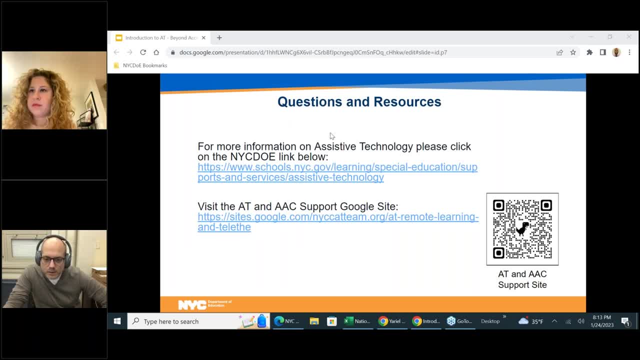 And this can be done remotely. The child receives AT devices. How can families engage AT teams to upgrade software? Correct issues? I think we mentioned this. a computer spread two years ago And the application needs updating Again. if there are glitches with that particular device, we would encourage you to speak to the IEV team. 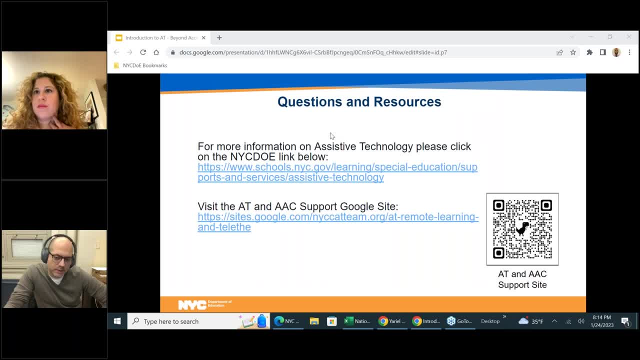 We ask that you reach speak to the your IEP team but also engage us in the process and will assist in the process of updating that device or updating the software on the device. Can parents ask for this at an IEP meeting? Another great question, As we discussed during the presentation. 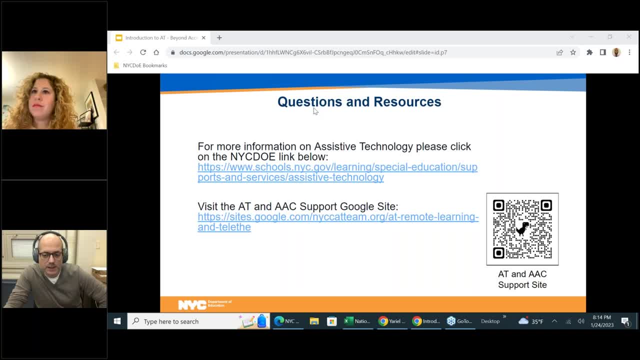 Assistive Technology must be considered prior to an IEP meeting. So we would encourage you, as the parents, to consider this And we encourage you, as the parent, to start asking these questions and whether or not Assistive Technology can help your child. Is Instructional Technology for kids, or it's only for kids with IEPs? 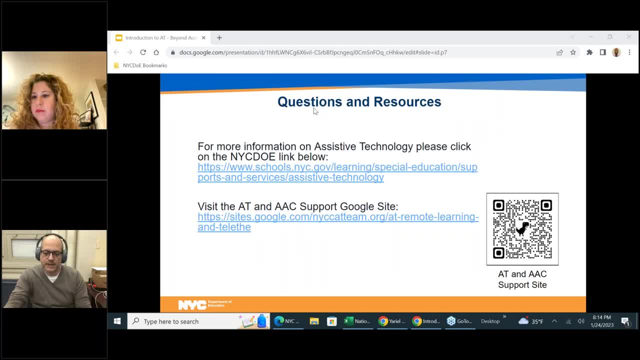 Instructional Technology? Great question: Universal Design for Learning. Instructional Technology is for all students, All students. I think we're getting to the end, Thank you. What happens if my son doesn't receive an event? What happens if my son doesn't receive an evaluation within 30 days? 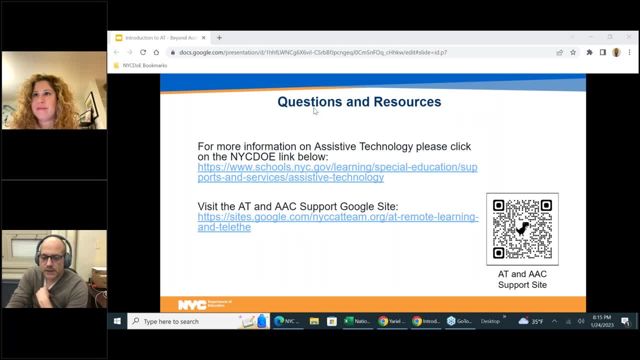 Is there a person I can speak to? I don't want the school year to end without him having an evaluation. We encourage you to reach out to our teams and we will work with you and the school team to remedy this situation and have your child evaluated as soon as possible. 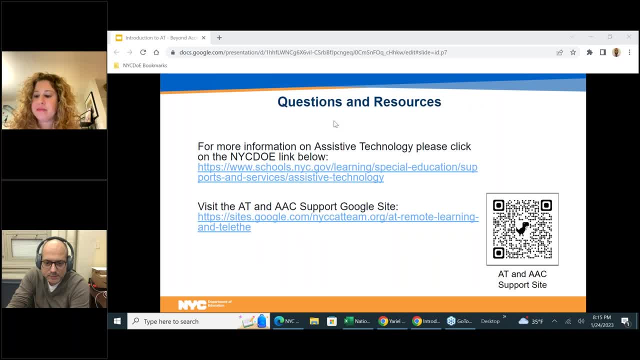 Mm hmm, Is AT the same as the iPad DOE provides? They use iXLine. No, so yeah, the DOE provided during the pandemic. they provide a remote learning iPad. That is Instructional Technology. If your student requires Assistive Technology, they may get a new device or at times, we may be able to add the Assistive Technology app to the remote learning device. 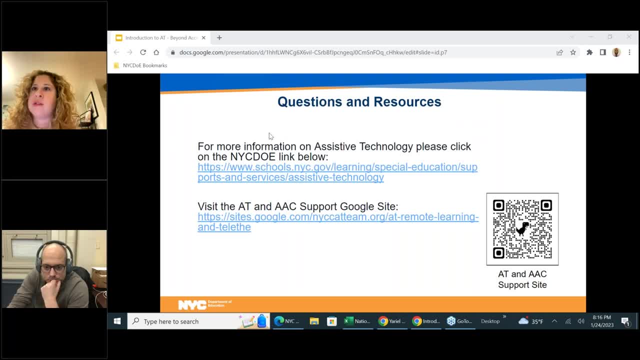 But that is not an Assistive Technology device, That's Instructional Technology. Hello, I don't have a computer at home. Can it be done by phone? I think this was regarding the presentation. Apologize, we didn't get to that. 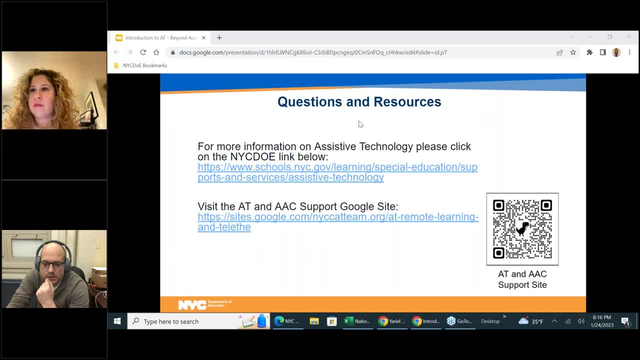 My son has a DOE. Thank you. Thank you, Ms Tarrant, Ms Grant, thank you, and thank you for all the amazing questions. I feel like I'm better from some of these other AT devices. How can I get reassessed? 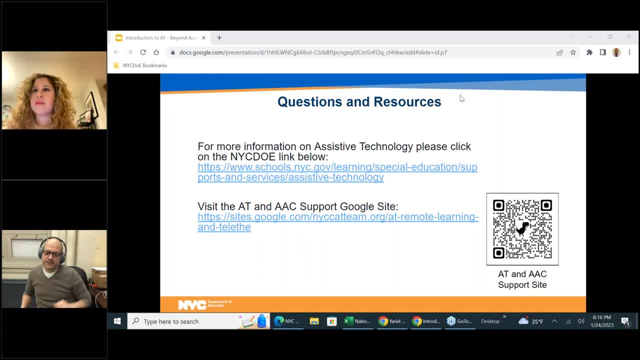 Um, This is also a great question. if my child has AT, but I feel he can benefit from some of these other AT devices, how can I get him reassessed? What we would say is: when your son has, or when your child has, Assistive Technology on their IEP, they also have the Assistive Technology service. 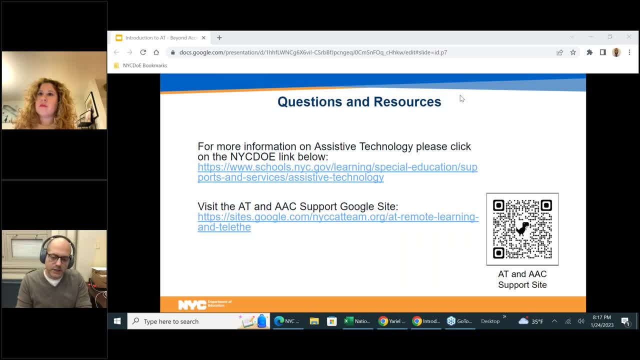 So you could speak to your IEP team and they could review the current Assistive Technologies and they can certainly use us as a resource for a consult Without even going through the reevaluation process. That's the beauty of the Assistive Technology service. 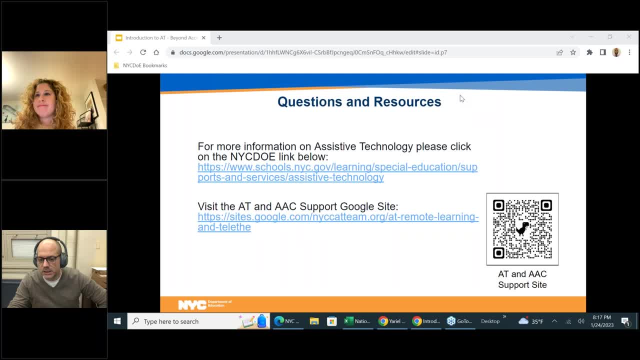 And it will expedite the process and actually get the help that your child needs. We have to. we have to cut it. yeah, be our last one. Okay, I'll put the emails up just for one more time, just for folks, if you didn't get a question answered. 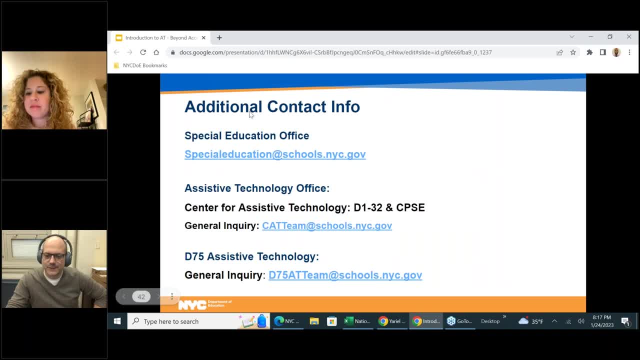 Okay, No, I'll put the emails up just one more time, just for folks, if you didn't get a question answered. I think you have a lot of time, Okay, Thank you. Thank you, Ms Grant. think the team did phenomenal. thank you all, thank you, thank you, thank you I.